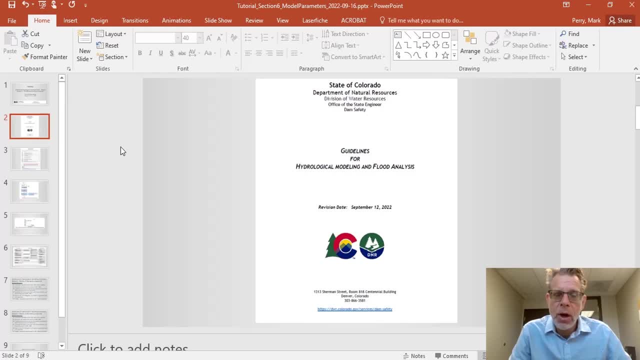 a lot of potentially big changes in results as we've worked to synthesize about 30 years worth of hydrology flood data, rainfall science into a pretty big overhaul of our dam safety, Colorado's dam safety, hydrology methods. So anyway, we felt like it was very important for 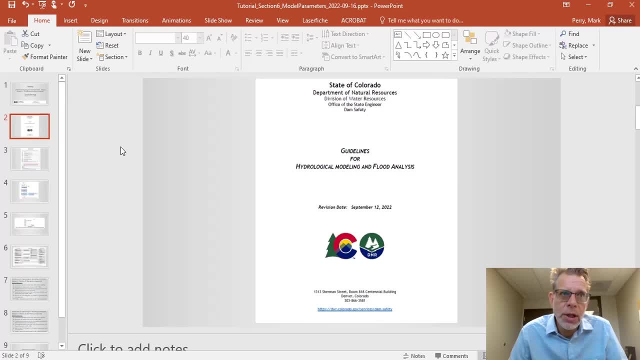 dam owners, consulting engineers to have confidence in the methods, especially in some of the big reductions in design floods, PMFs- that we might be seeing in the western three-fifths of the state and mountains and West Slope, And so we've completed that process and went well. We had the reviews by leading industry. 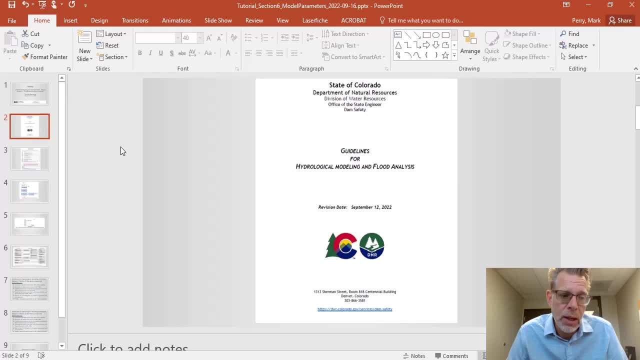 you know, nationally recognized industry leading experts in hydrology and flood analysis, USGS and light lolm. We had theiam and Ichi for iris engineering history lists. Mel Shafer with MGS engineering consultants, practitioners from AECOM and from reviewer from the Army Corps. 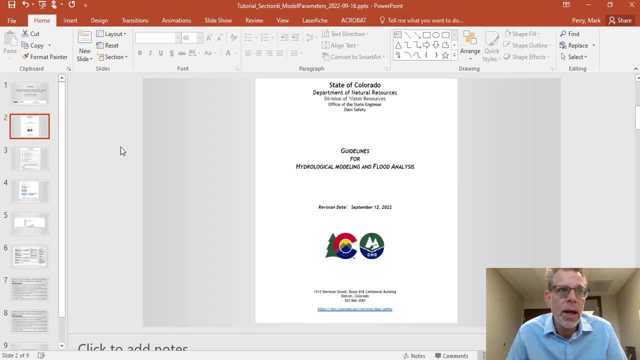 of Engineers Risk Management Center. So we appreciate all their input and the the final, that the guidelines as of are data data as of now, September 12th 2022. And those should be on our website now or shortly after now. And yes, this is a reality. What are they all trying to achieve? Better luck with that In mental health. Yes, Thank you, And two things: The best employee option: Mel Schaefer. 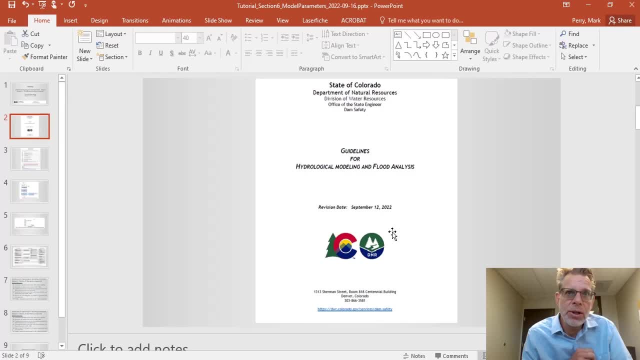 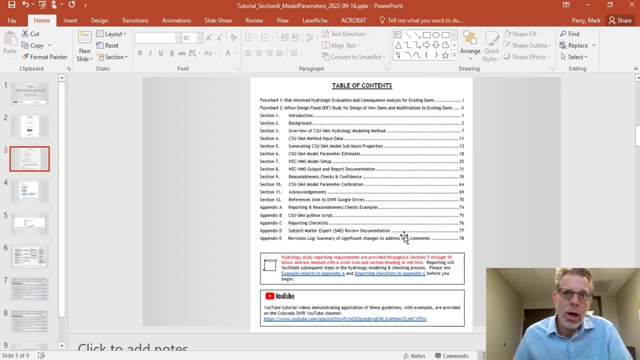 And you know we will issue this. Guidelines are living documents so we can issue updates, but as of September 12th they are considered final, no longer draft, And if you look at the table of contents, they now incorporate an Appendix D. subject matter: expert review, all the documentation, the comments from that review, resumes for the reviewers and the scope of work that we gave them. 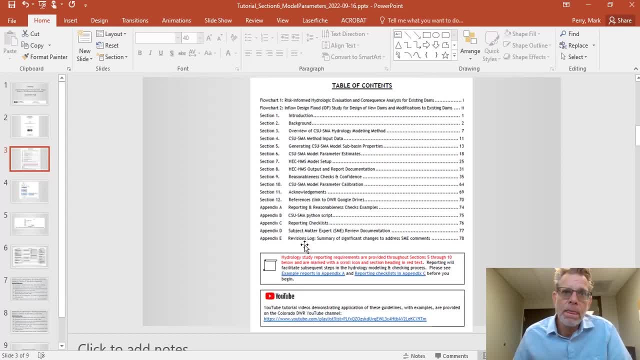 And then Appendix E lists a revision log to document the changes: number one to show you what changes have been made to the last draft, to the previous draft version that you had, and number two to show how we specifically addressed SME review comments. 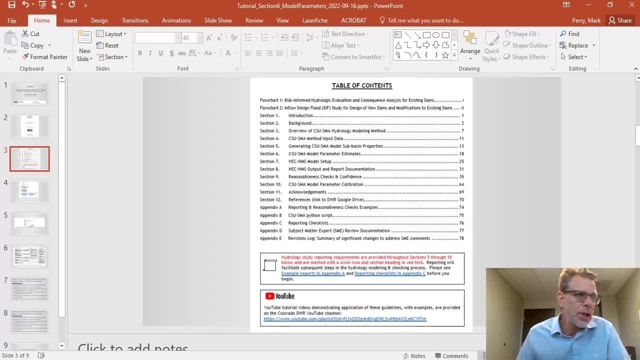 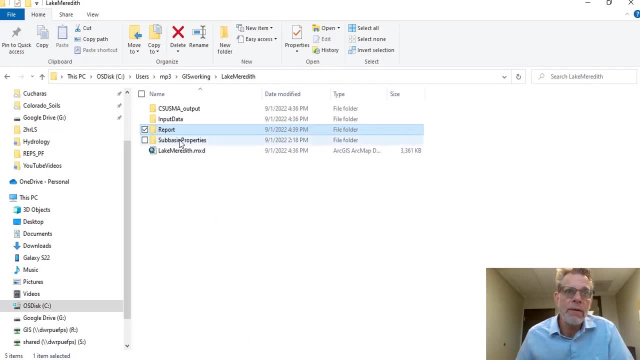 Okay, so let's, before we go on to Section 6, I want to do? I want to jump back quickly to Section 5.. And just Just remind you of where we've been. This is my example file. We're doing this or example project. we're doing this: Lake Meredith Basin or Reservoir on the eastern plains in the Arkansas Basin. 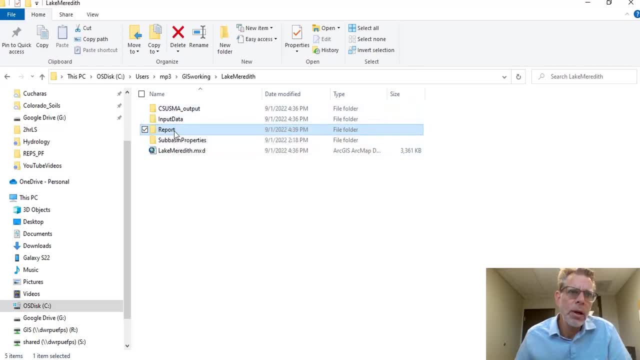 You can see my folder structure here. roughly, according to you know, following the guidelines, We have input data, We have the sub-basin properties And I have a I keep a reporting folder for all the separate reporting that's going. 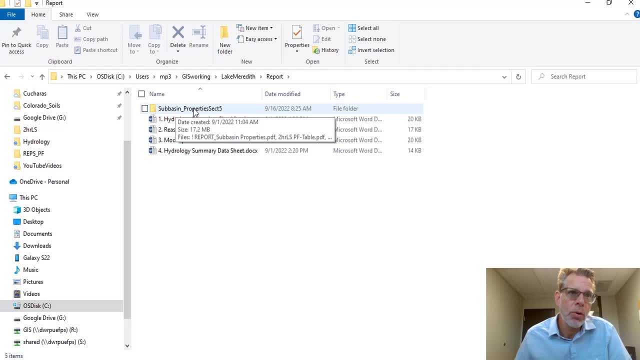 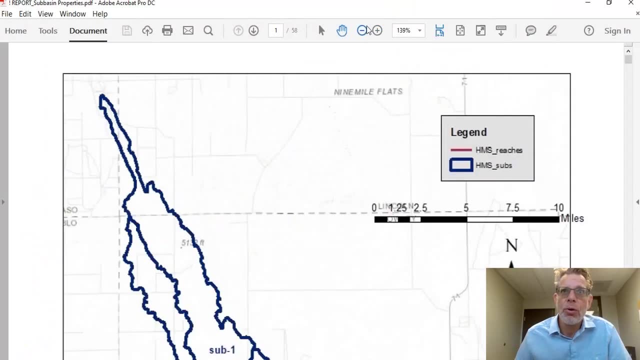 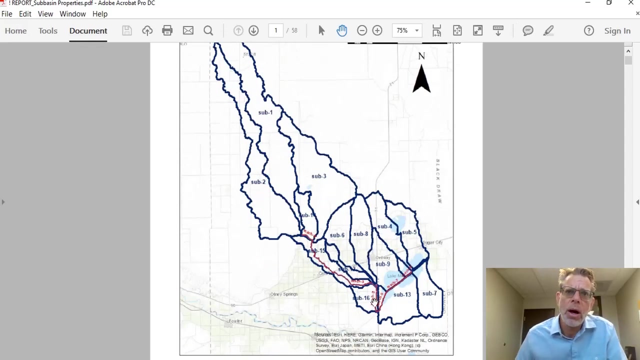 On as we work through the guidelines And so the Section 5 reportings, sub-basin properties, and I have a master PDF that has all of that And I just want to scroll through quickly and show you what that looked like. In the Section 5 video I showed output reporting from another example file, which is fine. 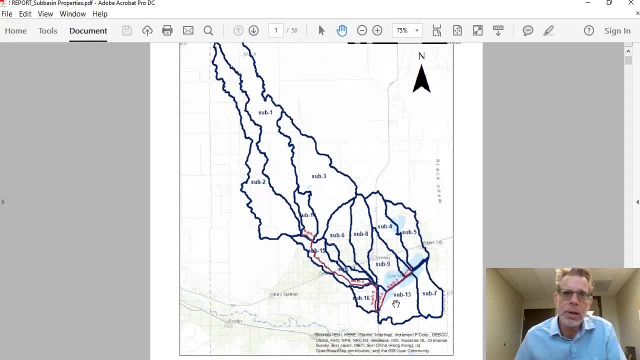 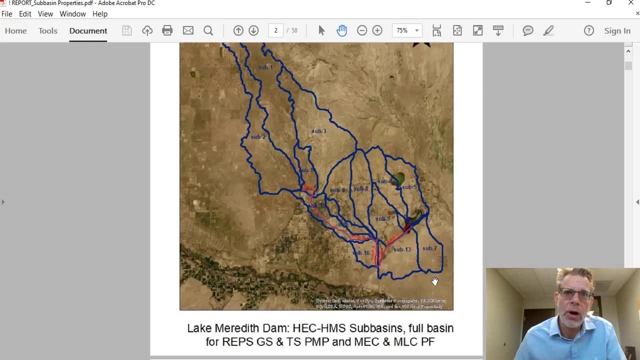 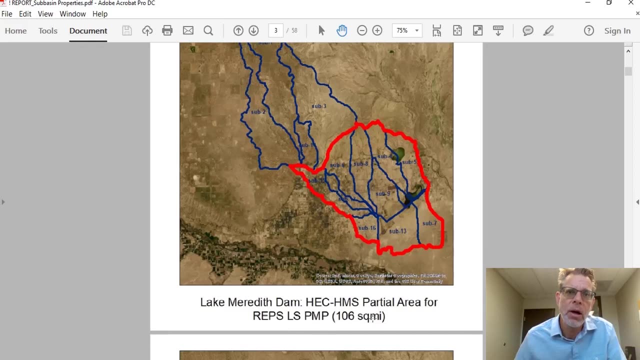 But I just wanted to do a quick recap. This is, for our example, basin Lake Meredith, showing the sub-basins map, sub-basins with Aerial imagery, then the partial areas. So this is the partial area for local storm PMP where we have the roughly 100 square mile storm area size limit for reps. local storm PMP. 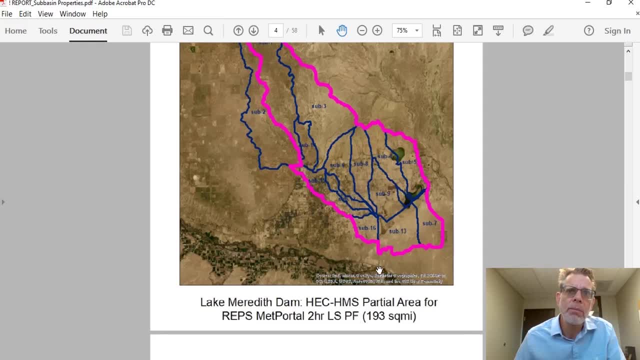 And then the second partial area is the. it has to be strictly less than 200 square miles in this eastern macro region for the two hour local storm precip frequency. So this is in met portal, The previous one map, I showed you partial areas for reps, PMP. 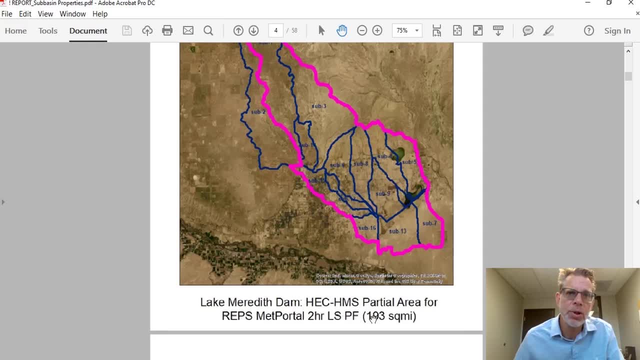 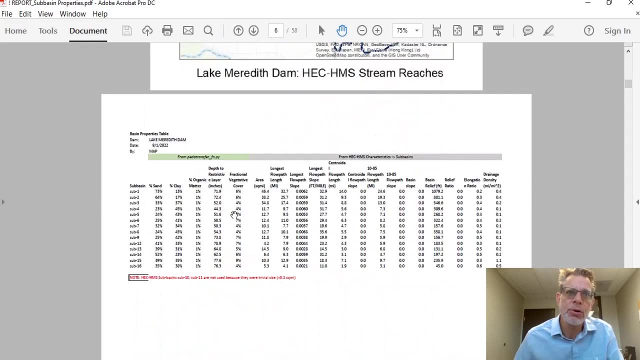 Now we're on met portal precip frequency, So different area, storm area size limit. So those are the partial area maps, Then a map showing stream reaches with those labeled, Then this master sub-basins property table that shows the output. 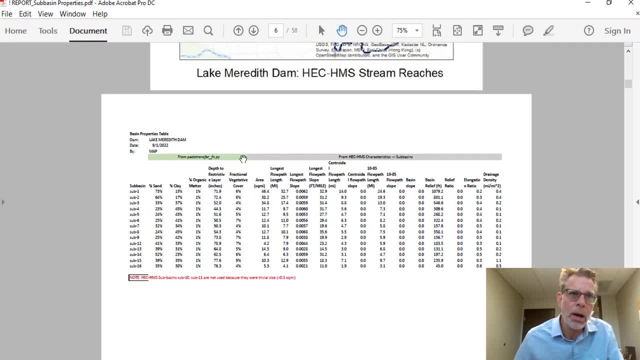 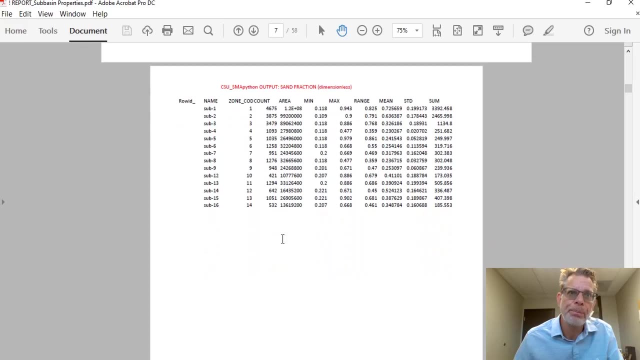 If you recall the output from the CSUSMA Python script that gave Sub-basin Average soil properties, And then all the output from the HMS characteristics tables, sub-basins, sub-basin areas, And we have the output from direct output from the CSU Python script. 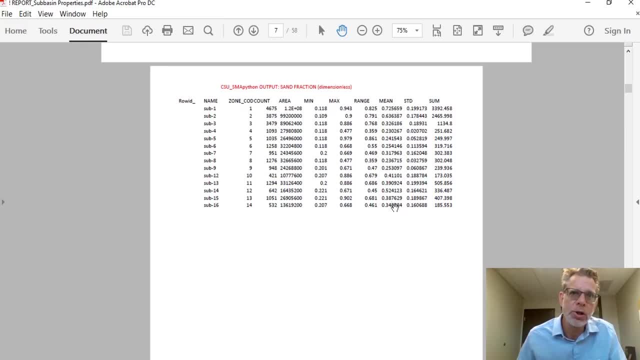 We want to see that, just to show. we're using this mean column on all these properties from this, from the zonal statistics. But we're using this mean column and we want to see that the data was input correctly. out of what exactly? So it came out of CSUSMA Python script. 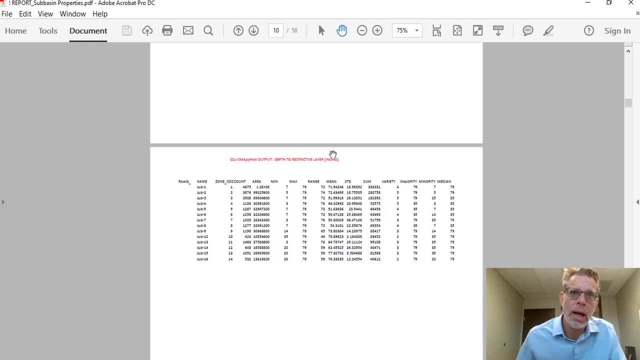 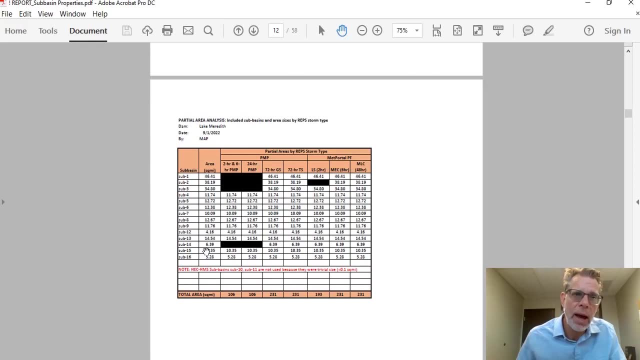 So that's clay, Organic matter depth restrictive layer and fractional fractional vegetative cover. This is our partial areas table, If you have partial areas. So if your basin exceeds the reps storm area size limits, the guidance is to do partial area analysis on those storm types that have relative tab that are restricted by reps storm area size limits. 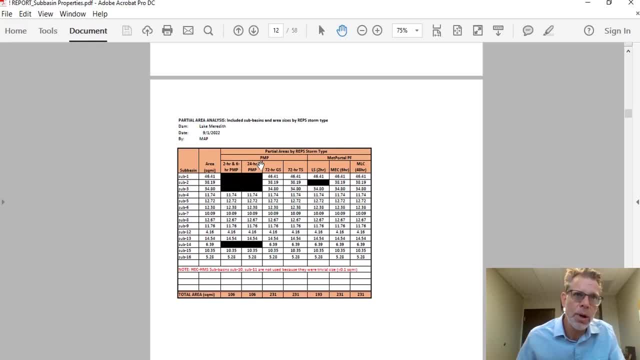 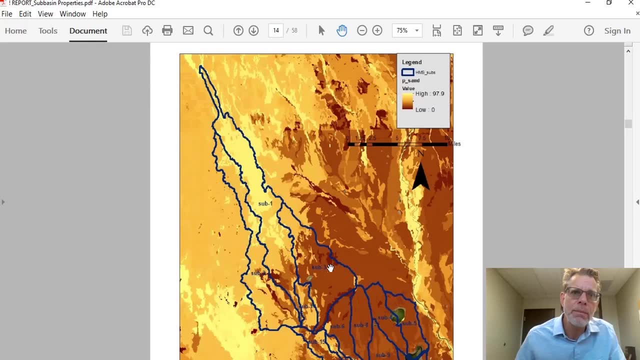 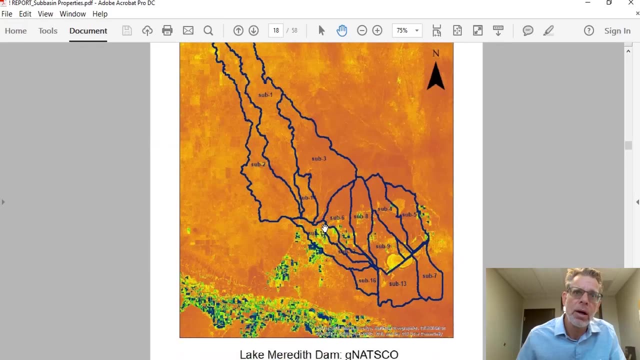 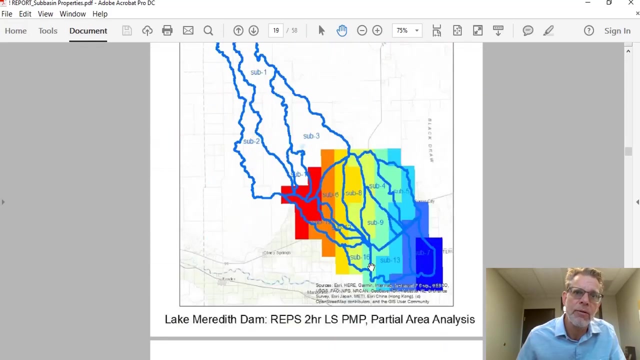 So we need to see Which sub-basins are you using for which storm type Reach properties summary table, then maps. We're asking for maps of sand clay, organic matter depth to restrictive layer. fractional vegetative cover just gives a good visual spatial representation of those. cross check everything we ask for the reps: storms output. This is for different PMP storms to our local storm Here, So we're asking for the reps storms output. This is for different PMP storms to our local storm here, So we're asking for the reps storms output. This is for different PMP storms to our local storm here. 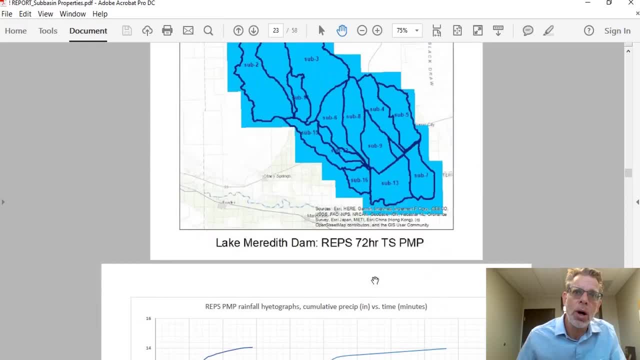 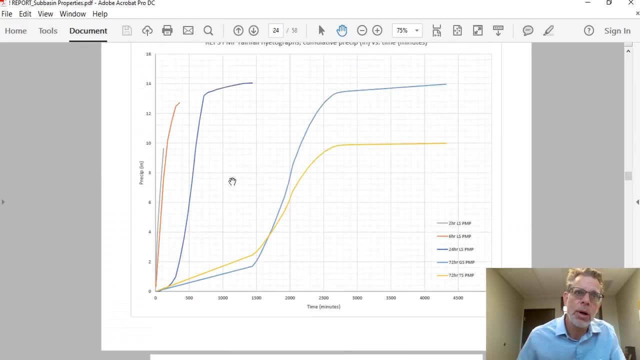 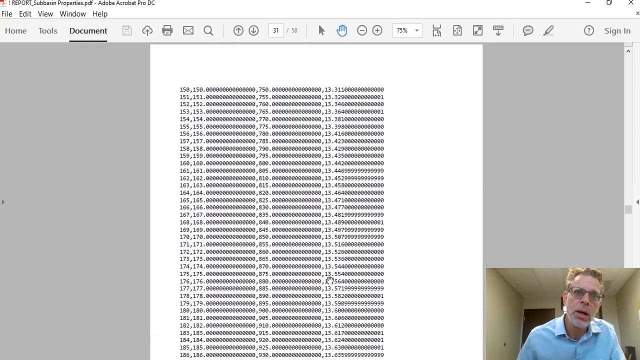 So we're asking for the reps storms output. This is for different PMP storms to our local storm here. Six hour local storm, So on. We have general tropical storms relevant for this basin and temporal distribution, temporal distributions height hydrographs- here The actual temporal distribution data from reps PMP tool. 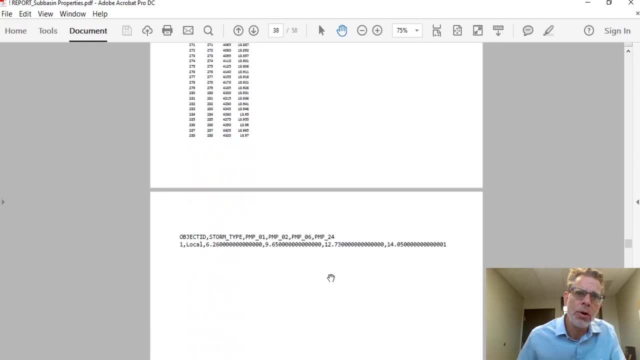 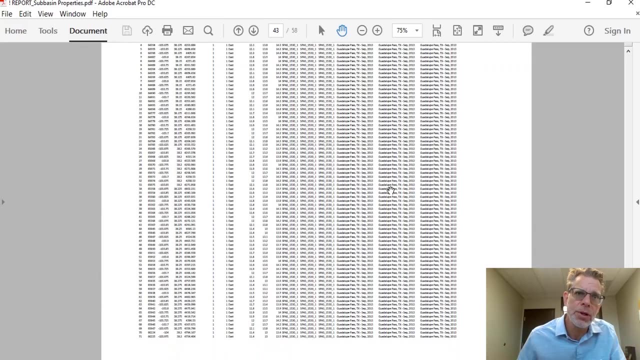 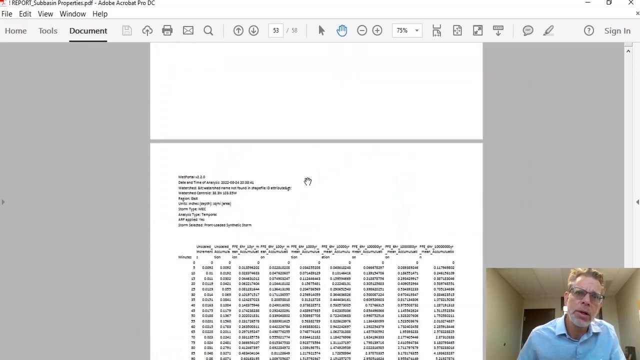 And then we get to After we've gone through all those storm types, Basin average and the point files And I've gone through, I'm going through this quickly, I've went through this in more detail. Section five tutorial. just to recap here: precip frequency output from the reps met portal for each storm type: 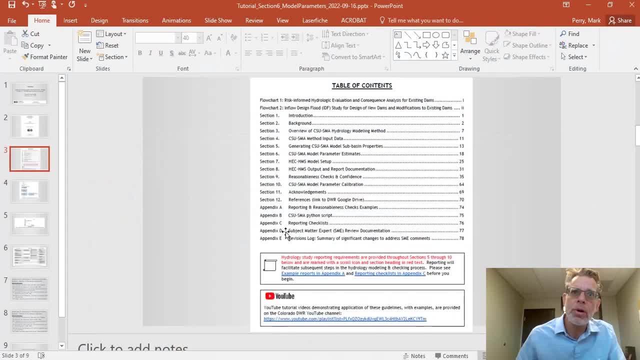 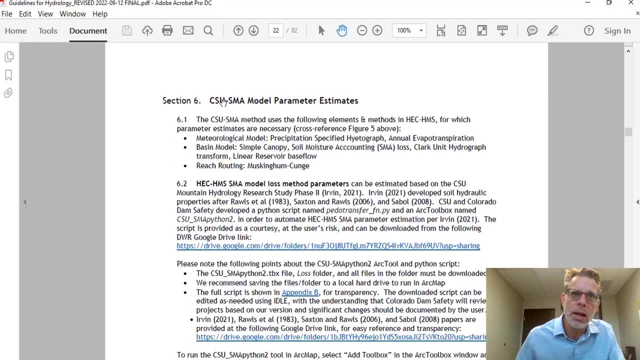 OK, And that's that. So that's, that is our, our properties. Now we want to use those properties to generate all the sub the model parameters. OK, So we're going to. now. we're on section six in the new hydrology modeling guidelines. 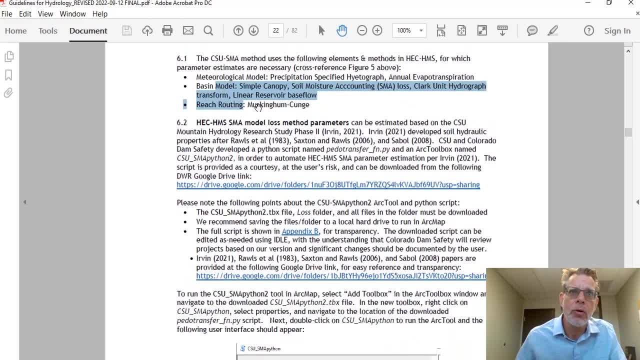 OK, If you. if you recall from the overview and tutorial section three, The CSUSM method uses these following Elements and methods: in Heck HMS so that meteorological models we use precipitation, specified hydrographs And annual evapotranspiration in the basin. model elements use the methods: simple canopy. 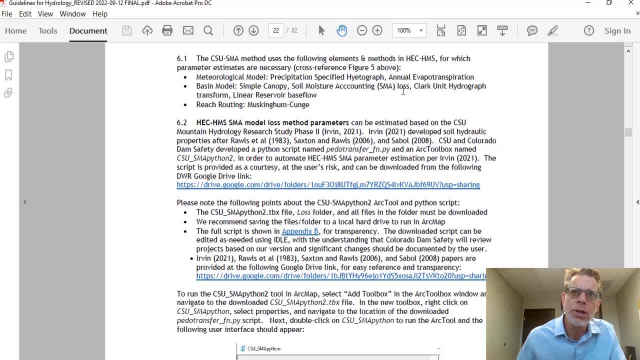 Basin model elements. use the methods: simple canopy Basin model elements. use the methods: simple canopy soil moisture accounting for losses. Clark unit hydrographs for the runoff transformation and then linear reservoir for base flow and reach routing is by musky animal country. all right before this next section of the guidelines goes. 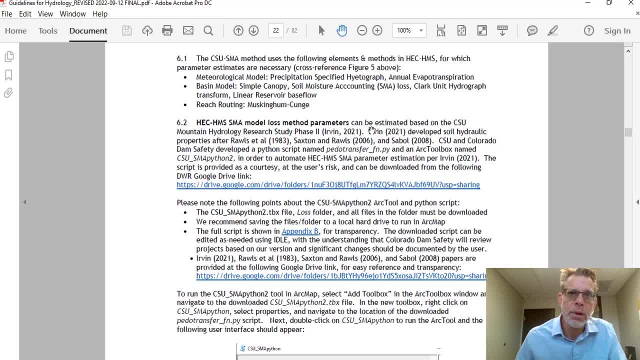 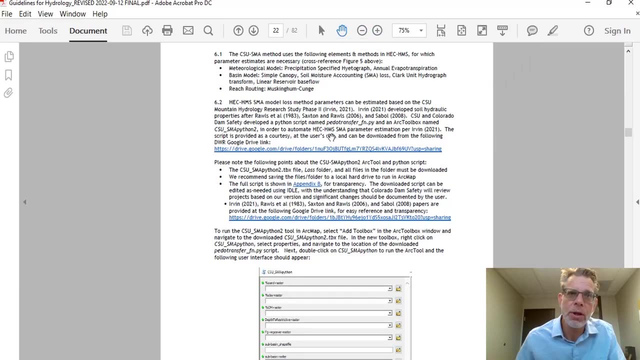 to the CSU SMA Python script and arc toolbox to calculate two parameters. but before we do that, I'm going to spend. this is a pretty easy. this section is pretty easy because it's mainly automated, but I want to spend time talking about the parameters so that there's no, we don't feel like it's a. 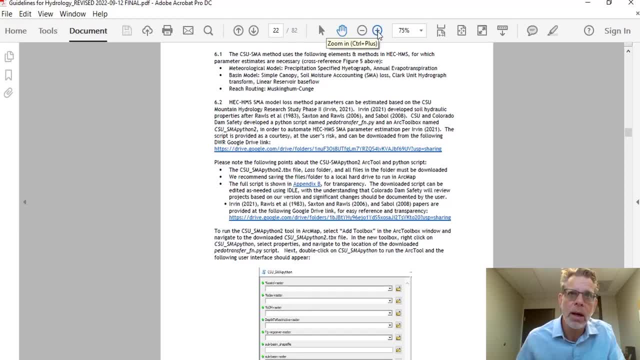 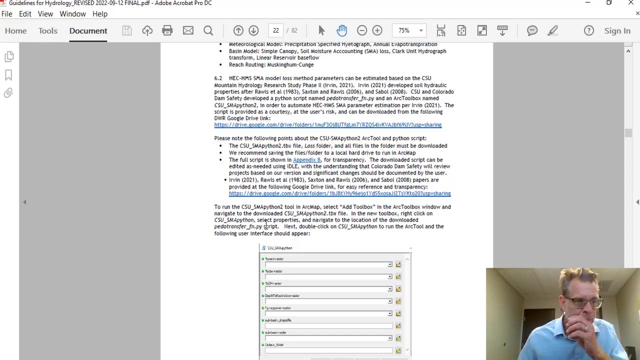 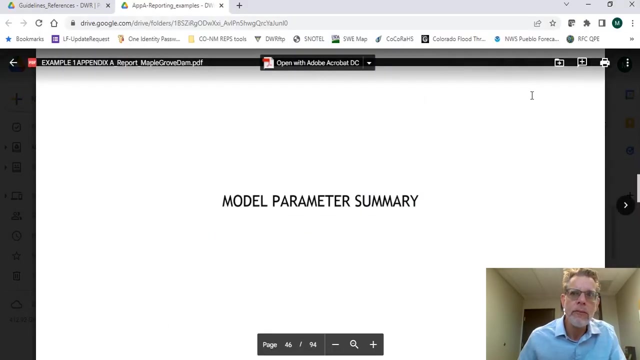 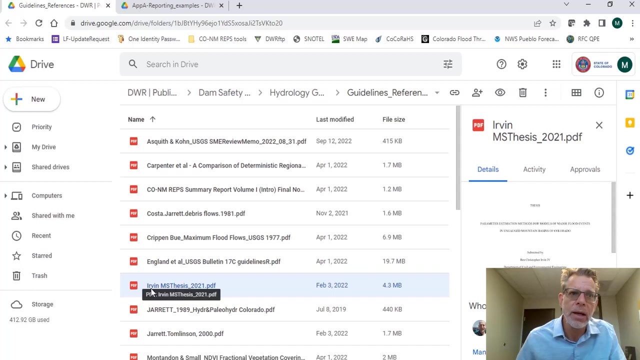 black box. everything in it is well documented. the information is here for anyone who wants to you know however deep you want to explore it. all right, so the CSU SMA model parameters- parameter estimation methods- come generally from the from Jeffrey Niemann, Dr Niemann at CSU and our second grad student phase two of the CSU Mountain Hydrology Research Study, Ben Irvin, his master's thesis. 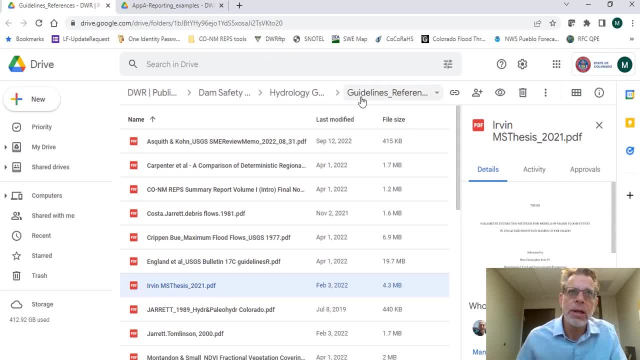 And we have that referenced in the guidelines. so section 12 of the guidelines, The references section, has a Google Drive link and we've tried to provide most all of those references for easy reference for you. So Irvin, master's thesis, And then Ben and we all co-authored a journal article saying: you know with this, generally the same information a little more concise. 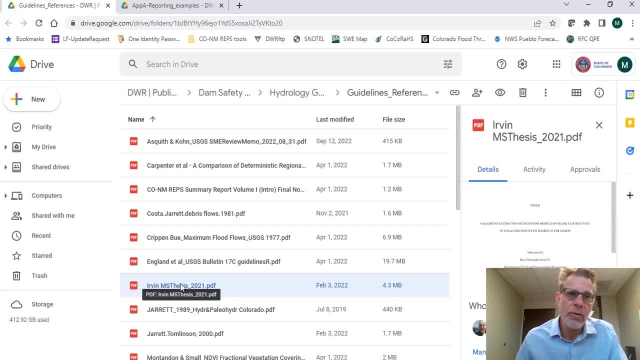 and a few updates, But that is currently under review. So when that is published- which we do expect it to be- we will update the guidelines and update the references section and then update the put that finished paper on their Google Drive for the guidelines. 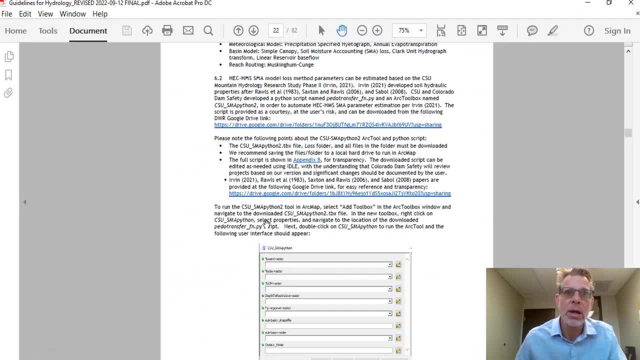 Okay, Back to the guidelines then. The soil properties are all in the method, are all calculated or generally calculated, And those are calculated by the series of papers from Rawls and Saxton and Rawls- And those were actually the same. 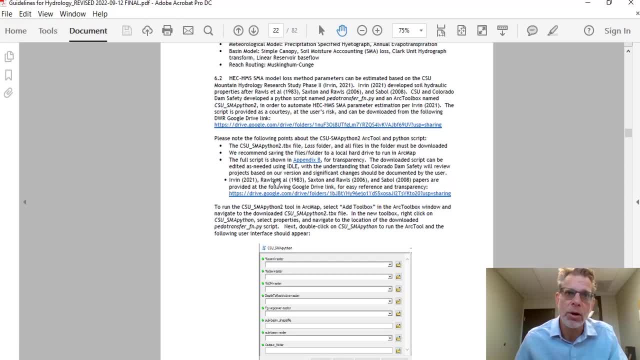 There was a set of research done by Agricultural USD Agricultural Research Service to develop green and ant properties based on soil texture USDA soils classifications And they were generally the same papers used by used by George Sable in our previous 2008 guidelines. 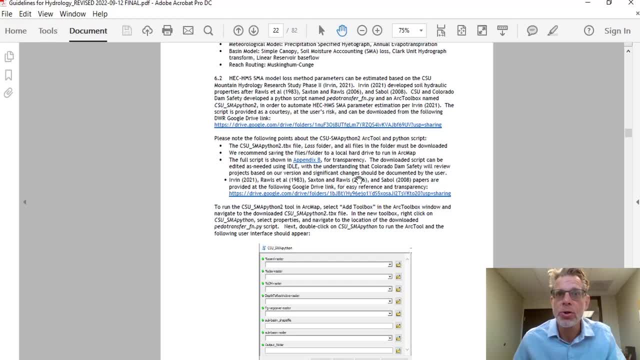 So those papers- the Rawls, Saxton and Rawls- Are provided on in our Google Drive of references And the previous Sable guidelines are still used. you'll see through here for several specific items. In general, the pre- our previous hydrologic basin response parameter guidelines from 2008 are superseded by these current new hydrological modeling guidelines. 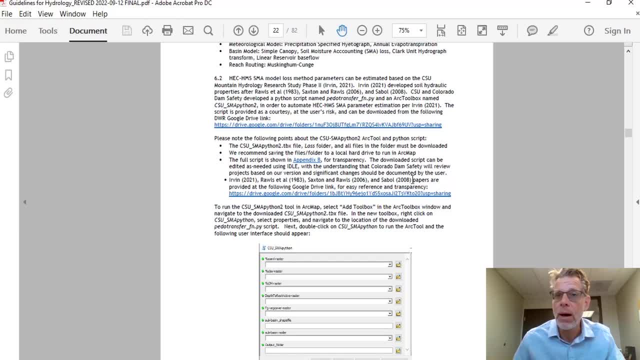 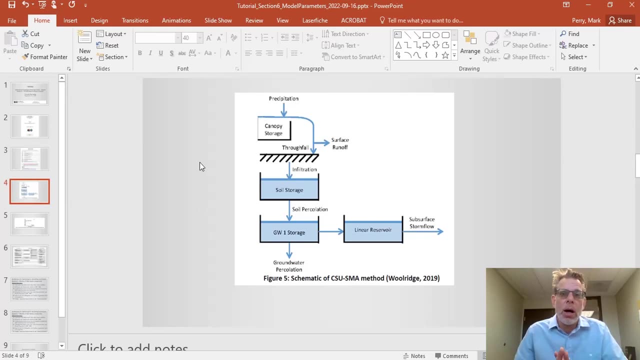 But we still reference them and we still use several of the equations From from that, from that, those previous guidelines. Okay, So let's go. let's go and to back to our PowerPoint here and just do a quick. this was from section three, again, where we gave an overview of the method. 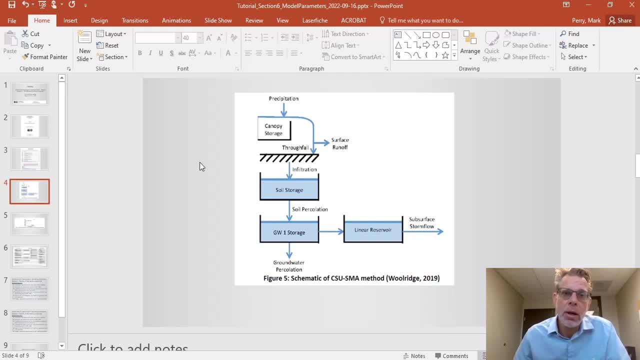 But let's just quickly recap that and talk about the CSUSMA modeling method and its its application in HEC-HMS. It's all developed using HEC-HMS, All right. so we had this schematic where we have precipitation falling. 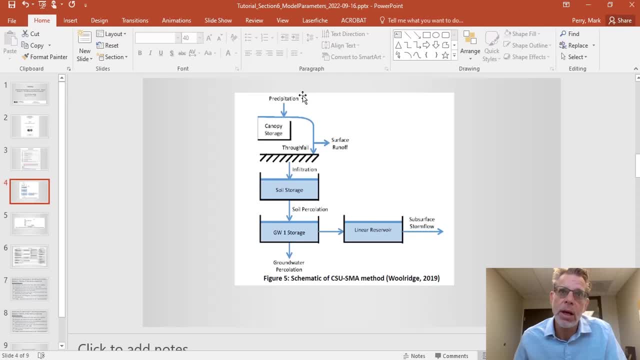 Of course the design rainfall comes from REPs, REPs-PMP and REPs-METPortal precip frequency. it goes into canopy storage. Any once canopy storage is exceeded that comes out as throughfall and falls to the ground. 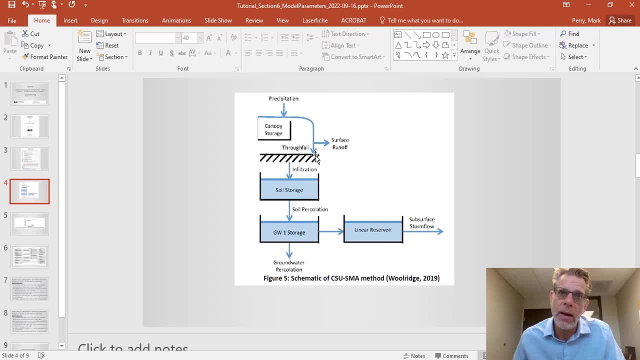 It infiltrates at a variable infiltration rate which is a function in the in the HEC-HMS SMA soil moisture accounting method. That infiltration rate is a function of soil water storage. So it starts at maximum infiltration rate when we are at zero soil water storage and then it decreases to zero infiltration at full soil storage. 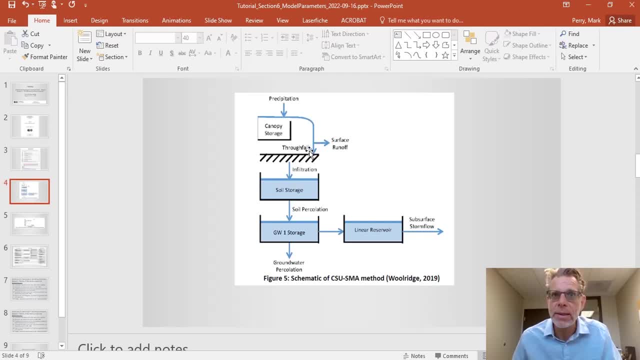 Once the throughfall exceeds the soil, that variable soil infiltration rate, the water will exit at. it'll be excess precip and it will go to surface runoff- Okay, Through, And that will be transformed For the precip. excess precip will be transformed to runoff using the Clark unit hydrograph. 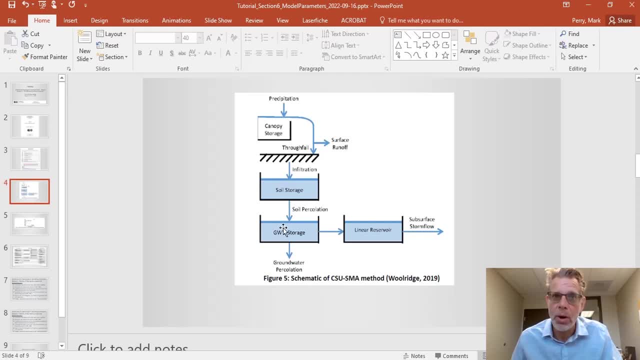 Okay, Now out of that soil storage water can percolate into a ground, a shallow groundwater level. Out of that shallow groundwater water can return as subsurface flow through this linear reservoir and return to be part of the surface water. hydrograph- runoff hydrograph. Okay, And out of that surface groundwater one shallow groundwater storage water can also percolate. Okay, And out of that shallow groundwater one shallow groundwater storage water can also percolate to deep groundwater, which is a loss to the system. 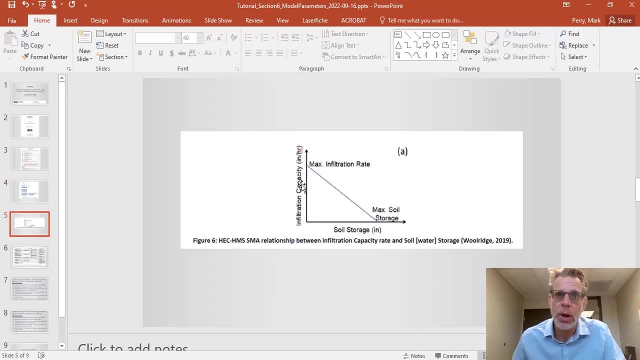 Okay, Now here's just a schematic showing that or a graph showing that. variable infiltration rate, soil infiltration rate. So at again, at zero storage it's maximum, And at full soil storage- maximum soil storage capacity- the infiltration rate goes to zero. 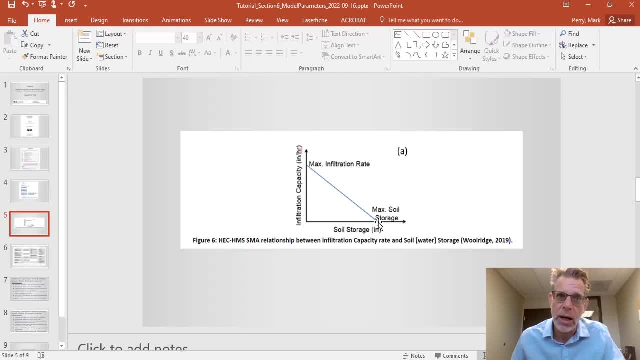 Okay. So this is a big difference from previous methods, like our previous guidelines, green and amp method, or initial and constant methods. Okay, Where infiltration losses were in infinite sync, Number one, they continued forever at a K, even at soil saturation, at a K saturated conductivity rate, with no respect or no recognition of soil saturation and potential saturation. excess runoff. 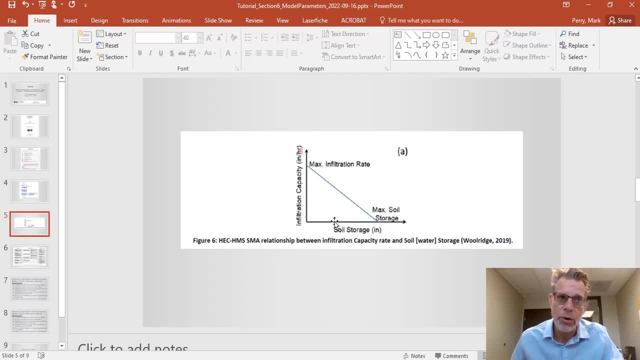 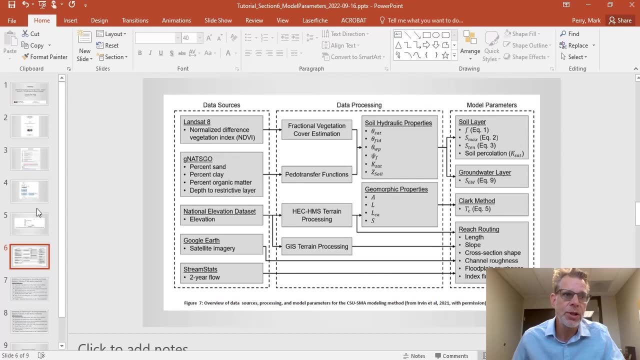 And then those losses disappeared from the system. There was no return as groundwater and no potential for saturation- excess runoff. Okay, So that's these. these graphs can be found in our guidelines, in section three and as well as this table. So Dr. 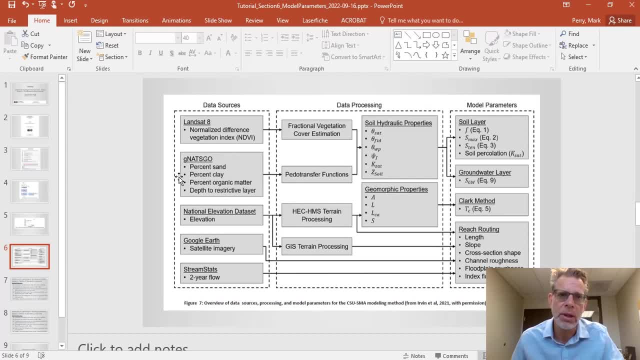 Niemann prepared this and I believe it's in Ben Irvin's thesis or in the paper that we have under review, But I think this is helpful. It's from section three gives a good overview of the entire CSUSMA modeling process and a pretty. our guidelines pretty much follow it in the sections. 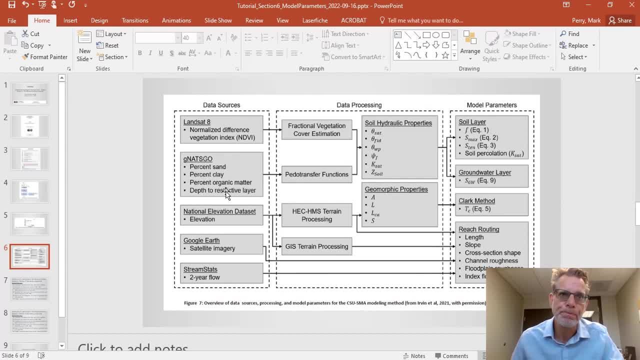 So we had section four, we had section five, we had section six, we had section seven, we had section eight, we had section nine, we had section 10, we had section 11, we had section 12,, we had section 13.. 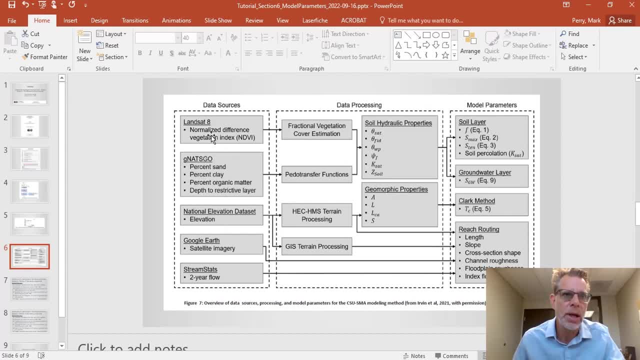 We had section four where we got the input data. These were all our data sources to get the Landsat imagery, GNATSCO, soils, DEM, StreamStats data. Then we did our processing in section five, basically what we call subbasin. 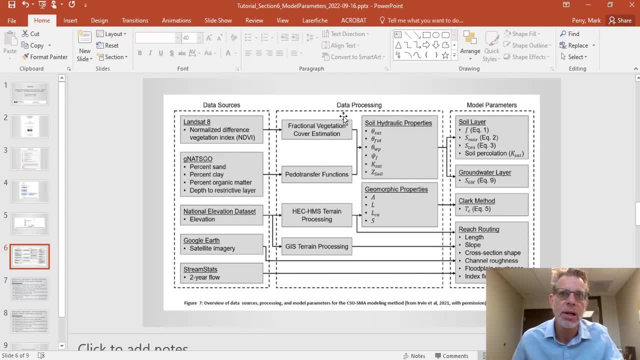 We did some pre-processing and then generated subbasin properties And that was our fractional vegetative cover. We did HECA, HMS, the terrain processing, generated terrain subbasin properties. Now where we used, we went ahead in section five and ran the CSUSMA Python script and we generated our percent average subbasin average soil properties. 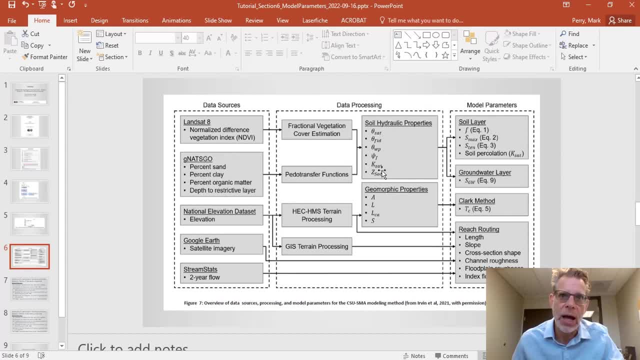 In this section. now I'm going to talk about these actual soil hydraulic properties and then how those are used by the CSUSMA script, by those papers from Saxton and Rawls et cetera, to calculate the HECA, HMS, SMA loss and other SMA or sorry, HECA, HMS element parameters for use in setting up the model. 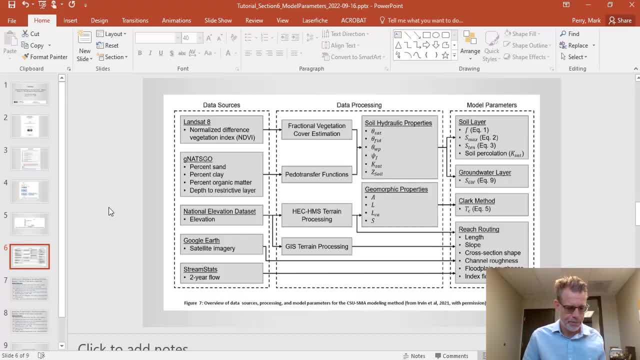 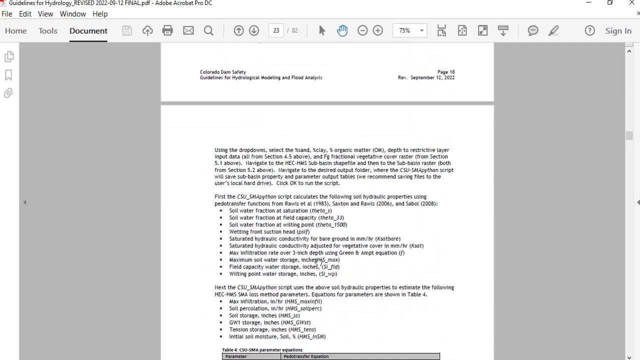 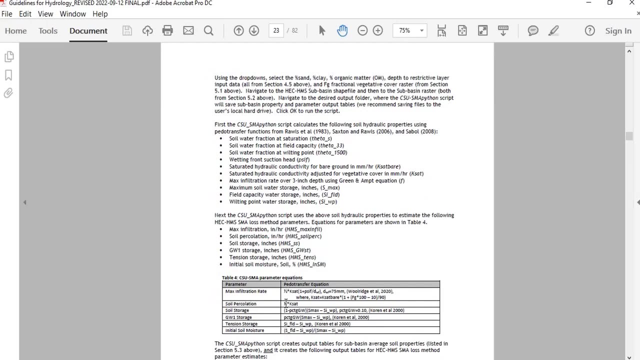 OK, so that's what we'll cover in this section. OK, so section six, let's talk about the actual, the parameters and the soil hydraulic properties from Rawls, Saxton and Rawls and then how they relate to parameters, And then we'll go through the remaining HECA, HMS element parameters, just discussing them. 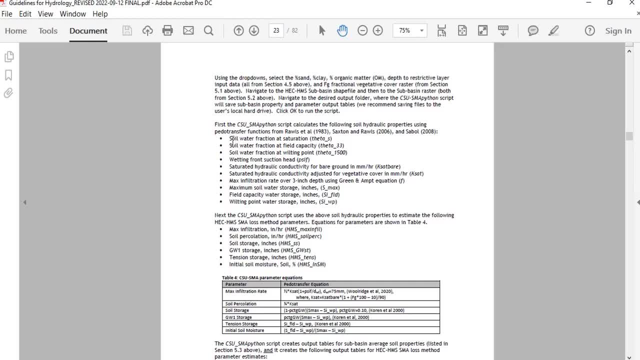 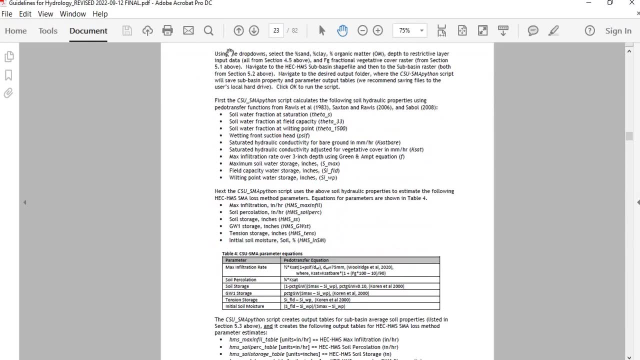 So everyone knows what, what they are. And again, there's no, no black box here. All right, So let's just, we're just use the guidelines. I just flipped to section page two of section six, the second, sorry, the second pages of section six in the new hydrology modeling guidelines. 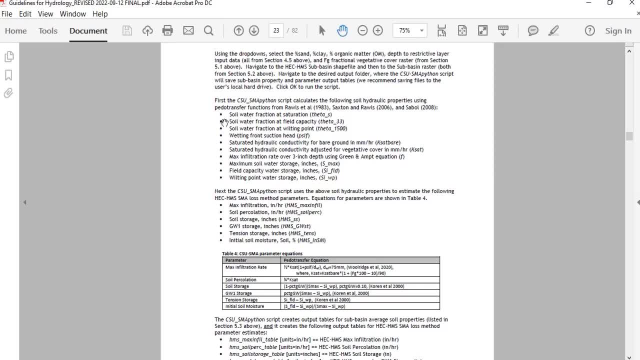 And let's just work off of that because that's what you'll have To reference, So that's what you're working from. So the first, first list here, bulleted list in section six, it lists the actual the soil hydraulic properties that are going to be, that are created or calculated from using the CSUSMA Python script. 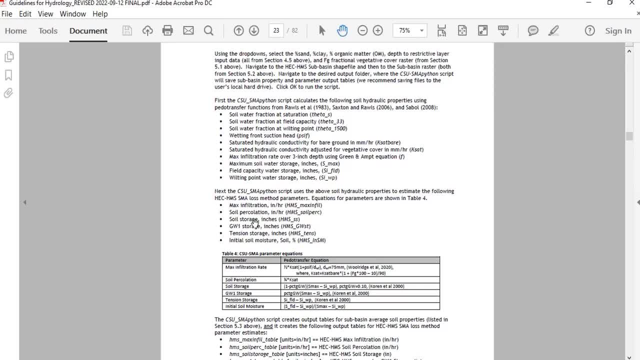 And this is. this is the ARC toolbox. I'll get into this next, But I want you to understand what it's doing before we actually open it and just run the thing, Because it's after that it's pretty much just clicking a button. 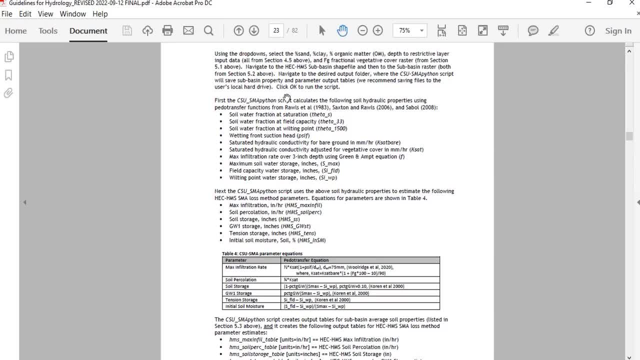 OK, so it's going to by Saxton and Rawls and using the soil properties which the script generates from the GNATSCO rasters, from USDA, NRCS GNATSCO rasters for sand clay, organic matter depth to restricted layer and then our fractional vegetative cover raster. 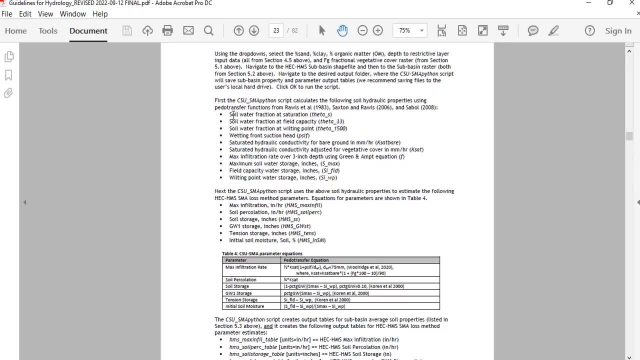 So it's going to. the script will create this soil water fraction, Soil water fraction as saturation. So these soil water fractions are just volumetric. OK, so right, Regardless of soil depth, it's just the fraction, So the amount of pore space that will be filled fractionally for for saturation and then field capacity. 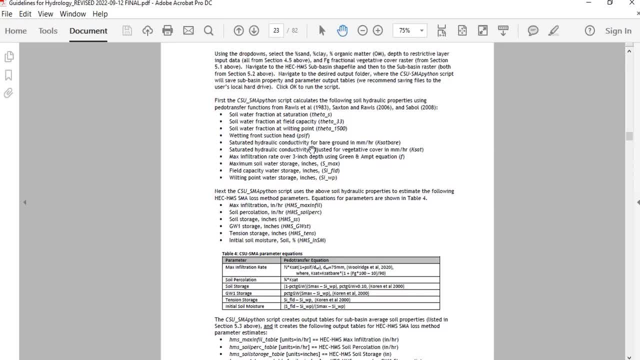 You know if people aren't familiar, depending on your background, how familiar you are with soil. soil hydraulics and soil physics field capacity is just the capacity that it at the limit of gravity drainage, so that soil starts out saturated. It's full. All the pore space is full. It'll drain under gravity to a certain point. 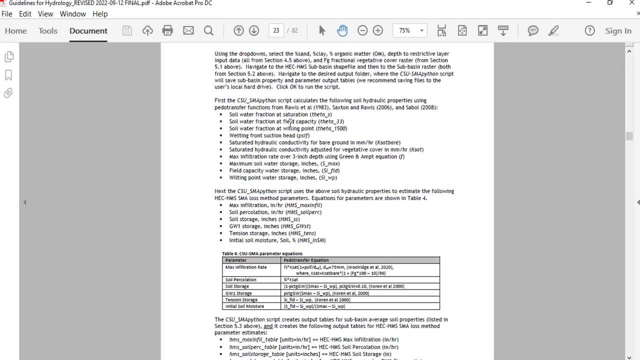 And then it's. then the remaining soil is held in tension, or capillary under capillary head, And that limit is called field capacity. OK, Then from field capacity there's another limit under capillary action, That's how much soil the plants can produce. How much soil the plants can pull out. So the plants pull out. They have their own capillary action and they pull out a certain amount of soil by, by evapotranspiration Right Or plant transpiration. So that takes us down to the wilting point. 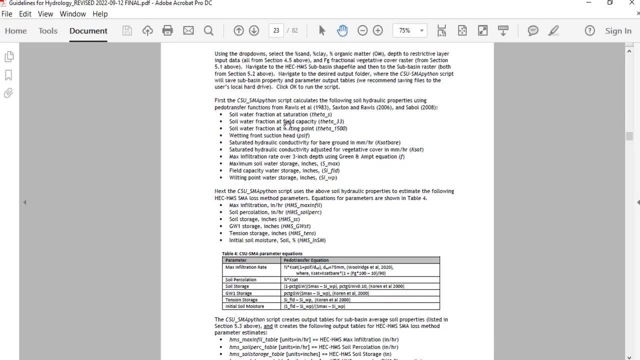 So the soil property, hydraulic property. next, or hydraulic property, is water, The soil water fraction at the willing point. OK, Then wetting front suction head. That's just a soil property based on soil texture. You know again you're getting. you're using sand clay, organic matter, that stuff. 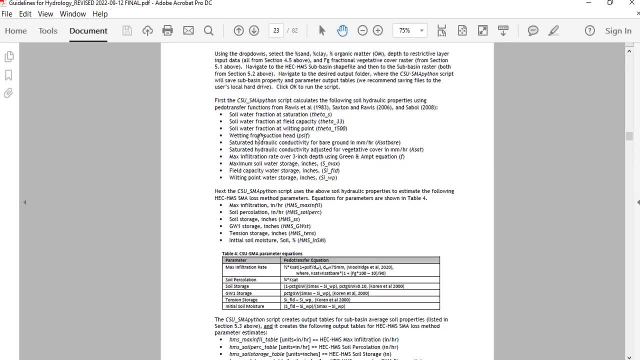 And that's essentially the capillary action, or head in the soil, based on soil texture. Then we have an important one, the KSAT, saturated hydraulic conductivity, And that's for bare ground. And then the script uses our previous Sable hydrology guidelines. 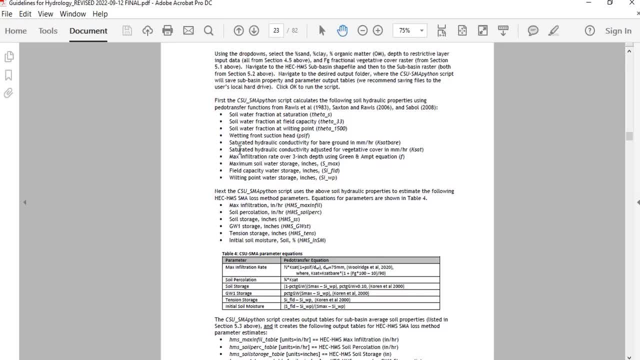 Really a relationship that was in there That increases saturated hydraulic conductivity based on vegetative cover. So that's why it was so important to get that there, Why we spent the time getting that fractional vegetative cover raster image. I told you it's not to get in the previous section five tutorial, not to get too bogged down in that, because we do have lots of opera. 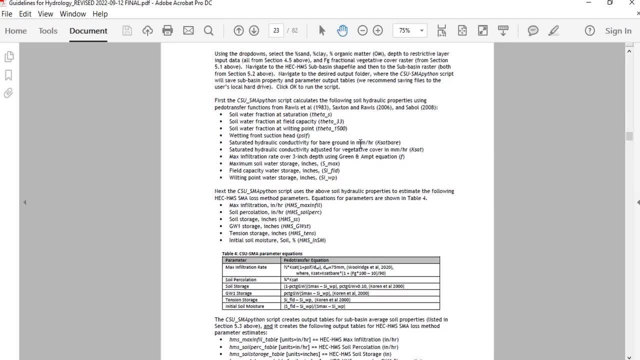 It's just a factor that's used. It's just a factor that's used to increase the bare ground case, But we have opportunities later in this method to calibrate the infiltration rate if it's not matching the observed flood record. So it's just a. it's just a step in adjusting that bare ground saturated hydraulic conductivity. 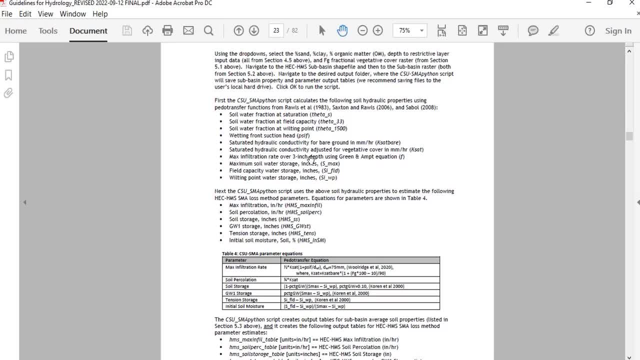 Then. then the script uses the green, actual green and empty equation To calculate a max infiltration rate. Okay, green and empty calculates a variable infiltration rate. right, But it's it that it has a variable depth as the water, soil, water, infiltrates. 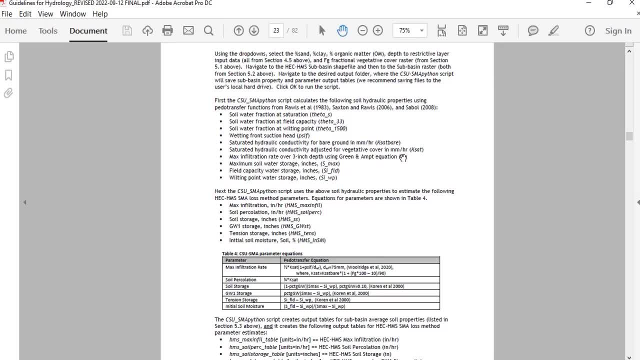 And and it will level out at. like I said it previously, it will level out at KSAT, So it can take the actual greening up methods. If you use that loss method in HMS, it would be variable based on depth, volume of infiltration. 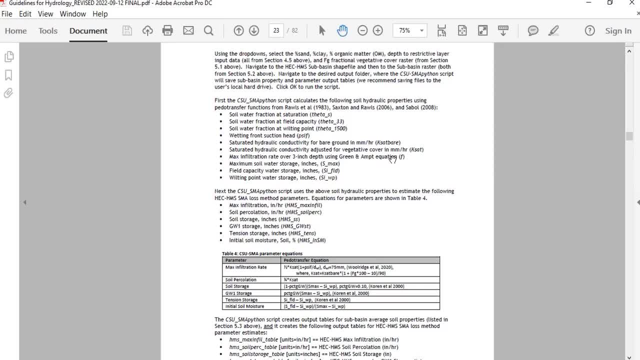 But then it would continue Infinitely at KSAT infiltration rate. We don't want that. We all we want here is just the maximum infiltration rate to use in our SMA method And we're using the green and empty equation to estimate that over an assumed three inch depth. 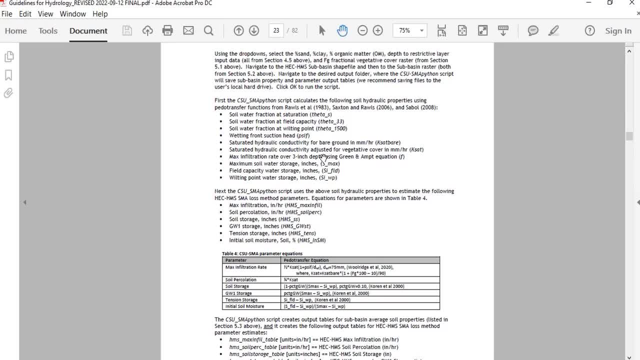 There's reasons for that And it's discussed in in Irvin's, Ben Irvin's master's thesis. But it's just a. it was just a good number to look at, representative of the maximum infiltration rate. Okay, Then these last three soil hydraulic properties: just convert these upper soil fraction volume, volumetric soil water limits to a equivalent depth of inches. 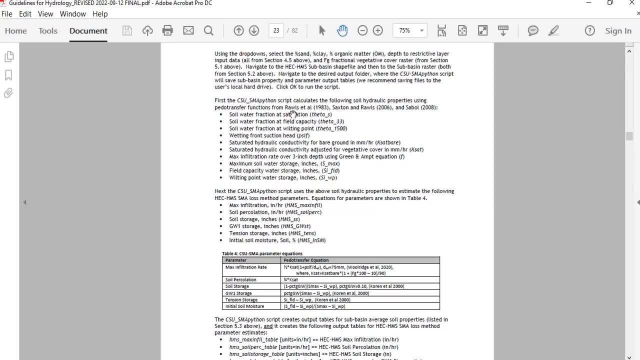 And that's just by multiplying these fractional, fractional amounts by the depth of the sub basin, average depth to restrict your player. So the depth of our soil layer, Right. So this fractional, fractional saturation times depth, So depth, is going to give us maximum soil water at saturation, or soil water at saturation inches. 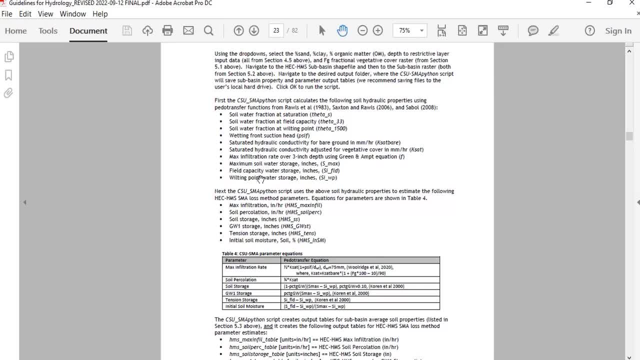 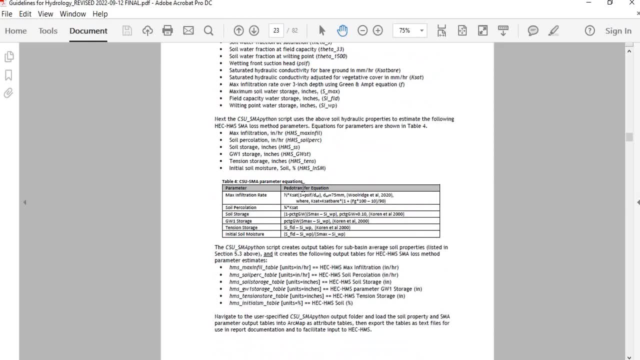 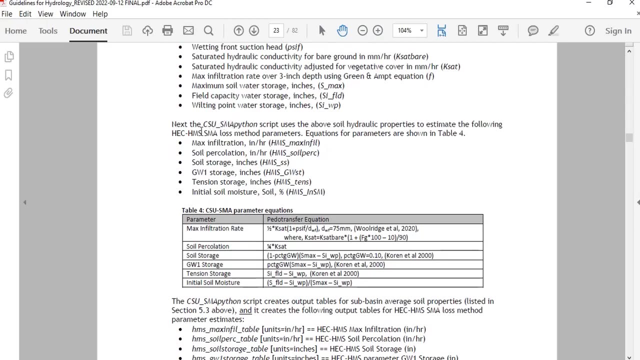 Same field capacity, water storage in inches and wilting points or water in store, And so willing point soil water storage in inches. Okay, So those are all used then to actually estimate the actual CSU SMA loss parameters, Using it by the CSU SMA Python script in our toolbox. 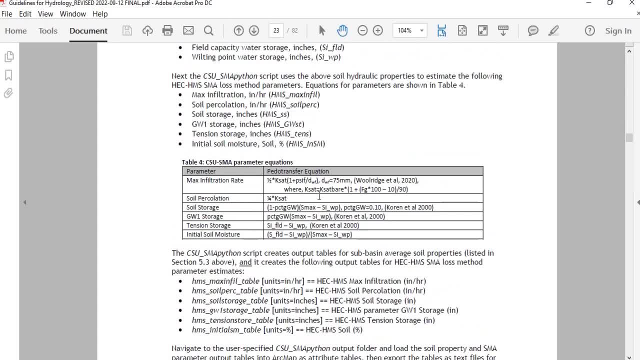 Okay, So these are the equations that Ben Irvin developed in his testing phase two of the CSU mountain hydrology method. that the test basins where they developed. He developed these research, these basins for these model parameter estimation methods, And then they did a verification phase where they they applied the method. 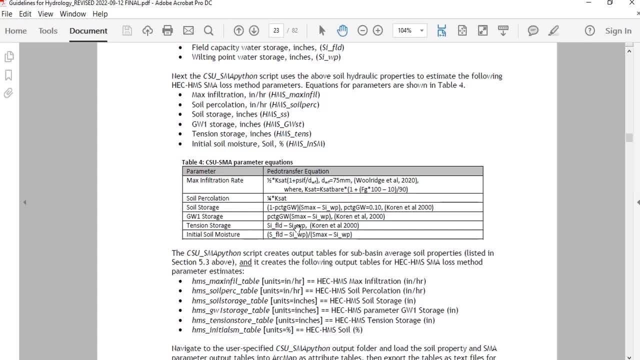 They applied the method to some new basins and three new basins And, I believe, five historic extreme storms in the San Juan Mountains and verified the methods on on those basins. Okay, So that was the phase two research And these equations come from Ben Irvin's thesis. 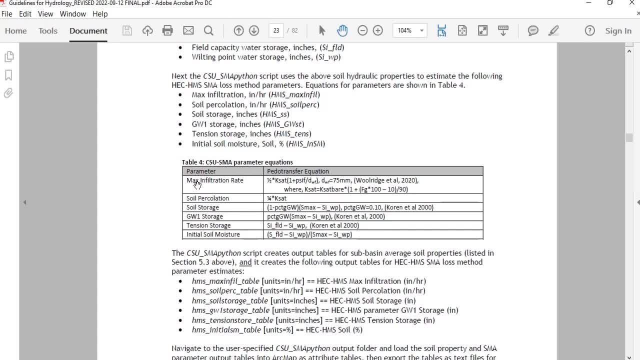 So to get that the heck, HMS- maximum SMA loss method, max infiltration parameters- You use this equation. Okay, Ben Irvin used us masters work, use this equation Right. So this is this is the, this is the green and amp equation And we're using this three inch depth, or 75 millimeters. 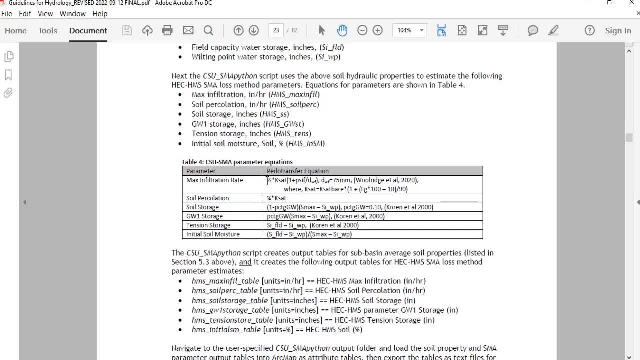 And the recommendation was to use one half bare ground. case sat in. I'm sorry, It's adjusted. case sat in that equation. Okay, So it's factored by a half. This is Si. F is the capillary suction head. This depth right in front is three inches. 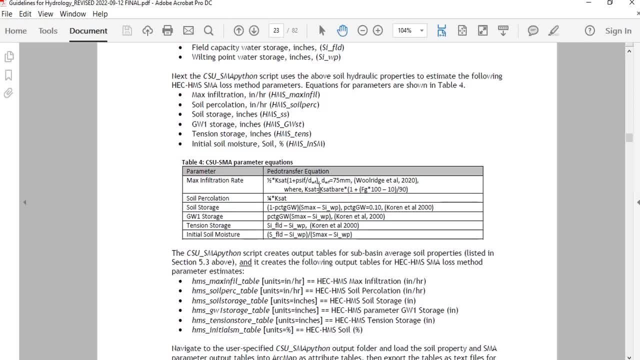 Okay Case, that is, there is the vegetative adjusted value. that's bare ground And this equation is from our old Sable 2008 hydrology guidelines: Fractional vegetative cover times: 100 minus this 10 percent, And that's over over 90.. 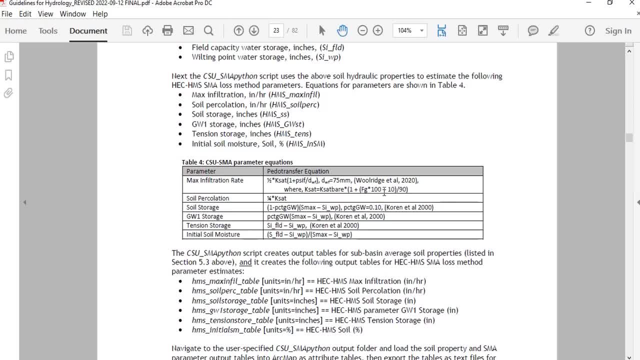 So at 100 percent vegetative cover, This that the bare ground case sat is actually doubled over the for the vegetative adjusted case. Okay, Then next soil percolation. So that's the amount of, that's the water that goes out of soil storage and into that shallow. 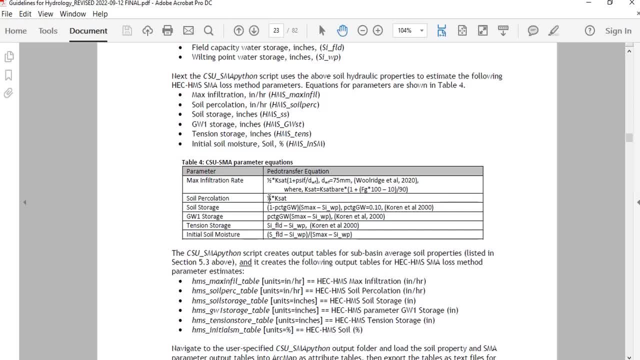 groundwater, Groundwater one layer in tech, HMS, SMA loss method And we use one quarter of that vegetation Adjusted case at now I believe in in CSU and their mountain hydrology research study. used one half case at in some of our efforts. 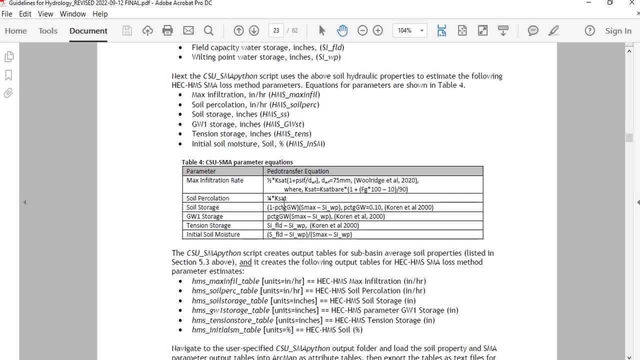 What we saw is that was putting an awful lot of water into the subsurface. We backed it off to one quarter. Now that can be calibrated. So if you're more comfortable with a half, based on the research, you can certainly change the script. 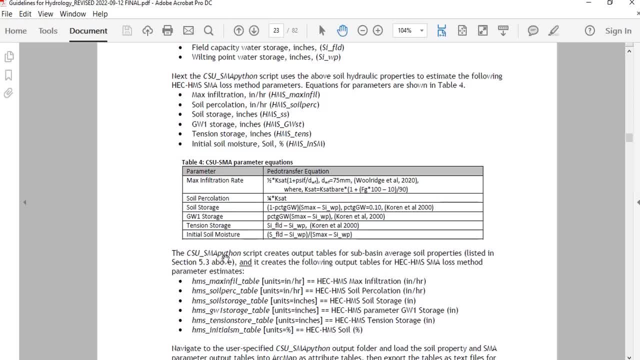 And I will show you how to do that. The script is available and it can be changed. Essentially is open source. I'll talk about that a little bit later. So it's not get, we'll get sidetracked on that. So storage. 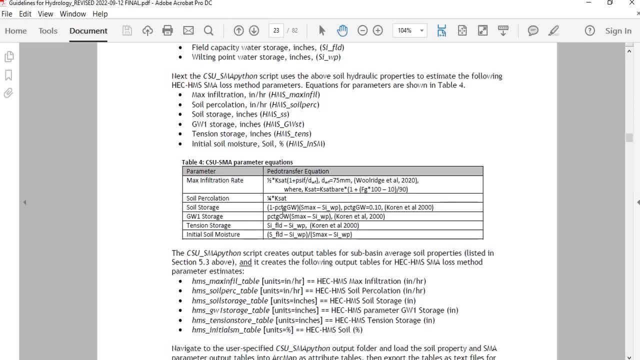 So the water storage is the. the method that urban did at CSU mountain hydrology research study did, is to assign a percentage of the total soil storage, So stores, storage being that available water between saturation and wilting points, And then to assign a fraction. 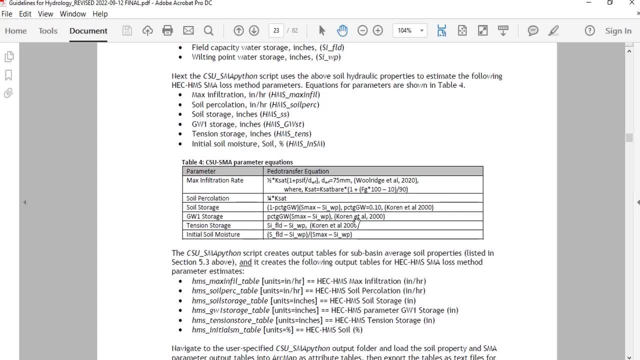 They used 10% to groundwater storage And then the difference 90% to the soil soil layer in heck HMS. So that's one minus this percent groundwater times this available soil water in the soil profile, And then groundwater of course is just that groundwater percentage times the same available soil water in the soil profile for each sub basin. 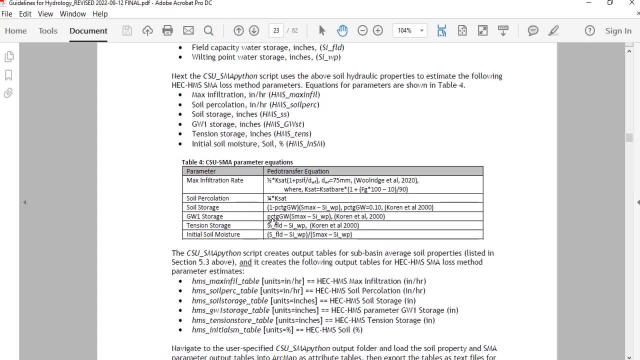 Tension storage. Then is that water that I was saying is held between gravity drainage and plant evaporation. evapotranspiration uptake Heck HMS once needs to. this SMA loss method needs to know that. And then an initial soil moisture is just a starting condition. 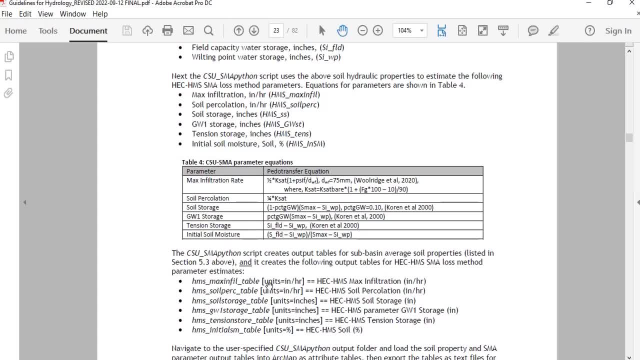 And we. the way the script is written right now is that that initial soil water condition is Is set at field capacity. So that's field capacity minus willing point over as a fraction of the total available water saturation or as max minus what wilting point. 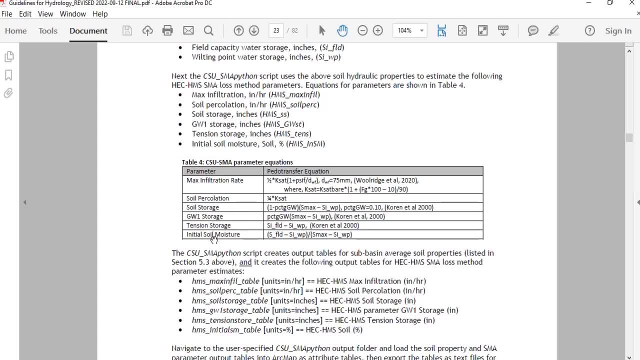 If you want that to be different, That is the general recommendation that we've had for calibrating for the CSU study of mountain basins and historical extreme floods in Colorado. Generally our soils, Jane, especially mountain soils, Drain very quickly. 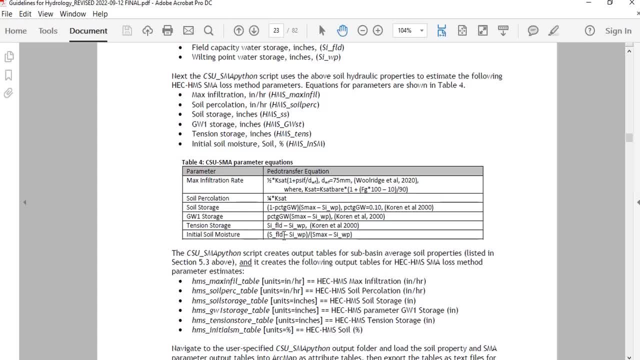 And what we saw in our proof of concept study. If you remember, back to the introduction of these tutorials, introduction to the guidelines, We did a proof of concept study on a for a large dam basin study in the Front Range Mountains And what we saw there, based on historic, the historic flooding from the September 2013 floods. 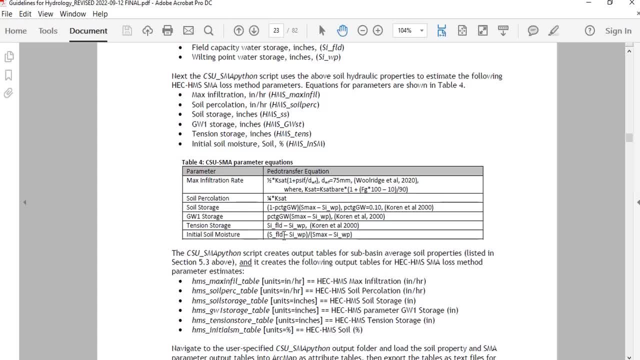 Is it within a matter of days? after a historic- Probably five hundred hundred years, Five hundred hundred year to five hundred year recurrence interval, Storms and floods, We saw that the soil had pretty much drained back to field capacity when we went and looked at subsequent events. 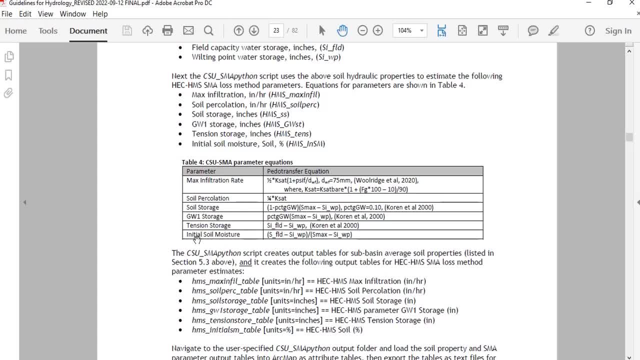 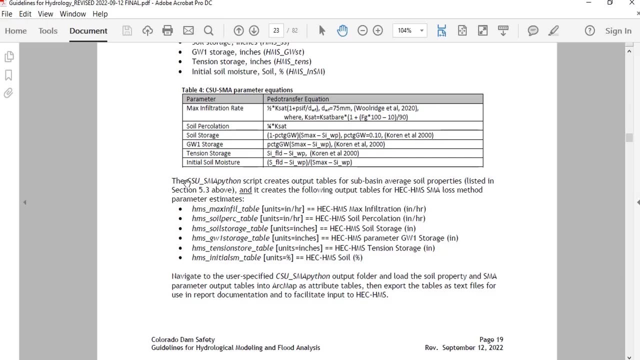 Continuous, a continuous simulation. Looking at a continuous simulation over the week following the September 2013 floods. Okay, Now The script- The CSU Python script- Actually calculates, gives these parameter estimate tables. So if you compare this bulleted list, 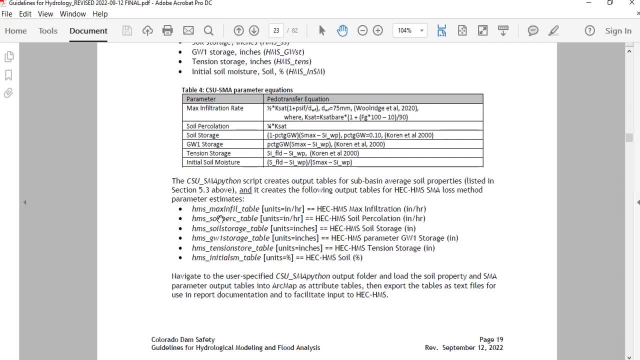 This is the actual output from the CSU SMA Python script And these parameters correspond. These are the table names that in the output correspond to each of these. in table four, And these are these correspond to the gives the equivalent heck HMS parameter name. 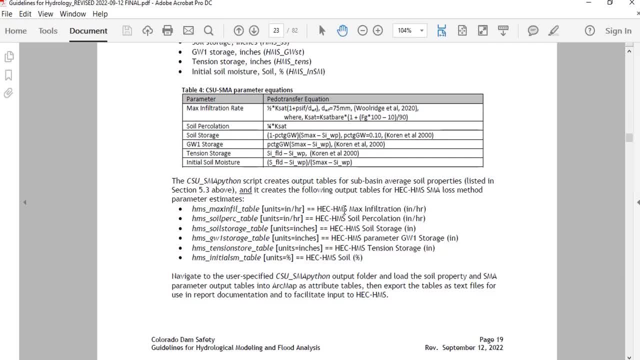 But these are generally each specific parameter for the CSU Or for the- sorry for the heck- HMS SMA loss method. So this HMS max infill table from the CSU SMA Python script is what we'll use. That mean column again from the zonal statistics. 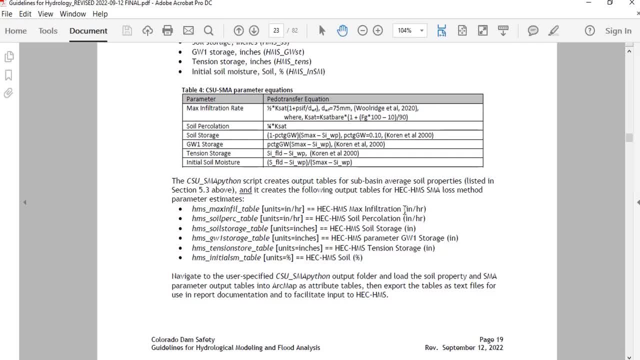 We use that for the heck HMS max infiltration parameter estimate. Get free. And these are all by site calculates is all by sub basin. So each sub basin set up in our heck HMS model, So perk will be this HMS So percolation. 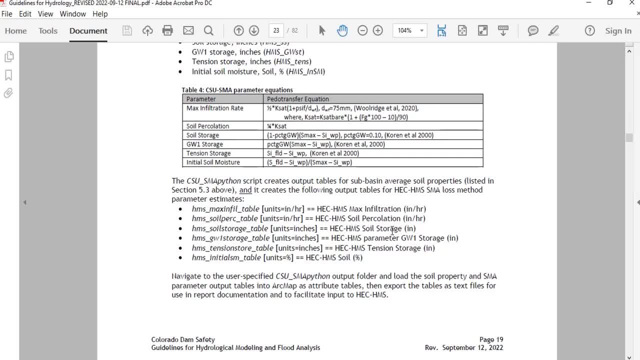 So percolation parameter, Soil storage, So HMS soil storage parameter. Groundwater, Groundwater, one storage parameter in heck HMS, Heck HMS tension storage And then in heck HMS the soil percent is that initial starting soil water condition? Okay, So essentially antecedent moisture. 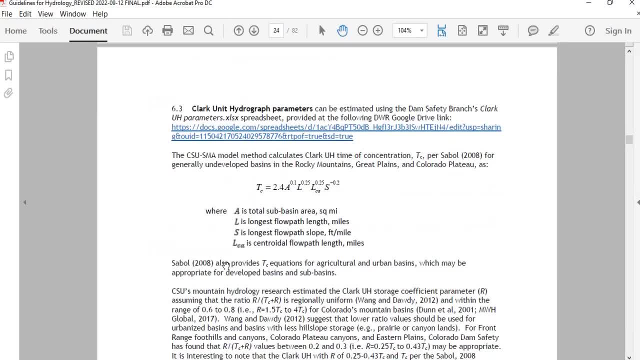 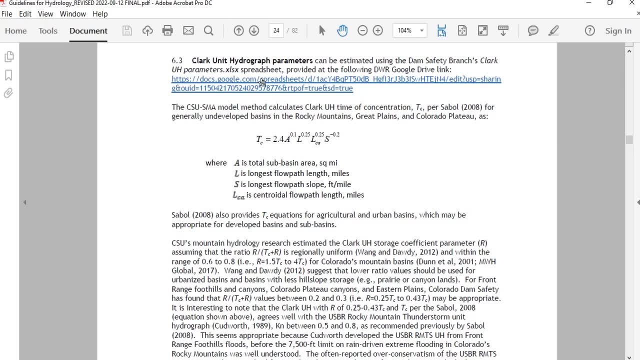 Okay, Next, that's. that is all regarding the heck HMS SMA loss method. Next, let's talk about runoff transformation, And there's a fair amount to talk about here in terms of guidance. It's easy to do, But let's just talk about the guidance and what the recommendations are. 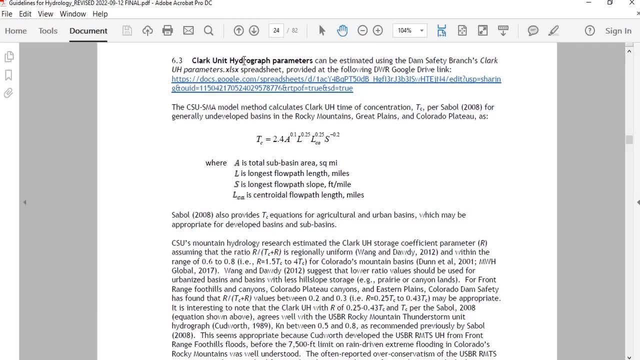 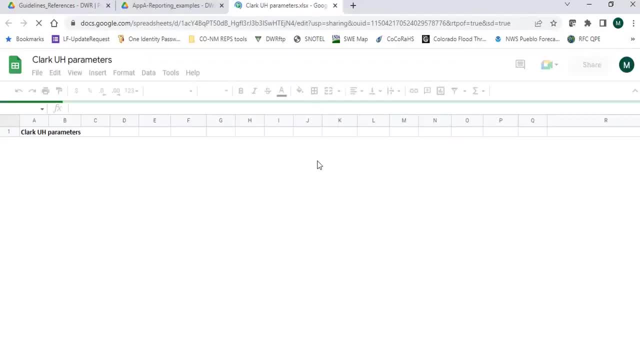 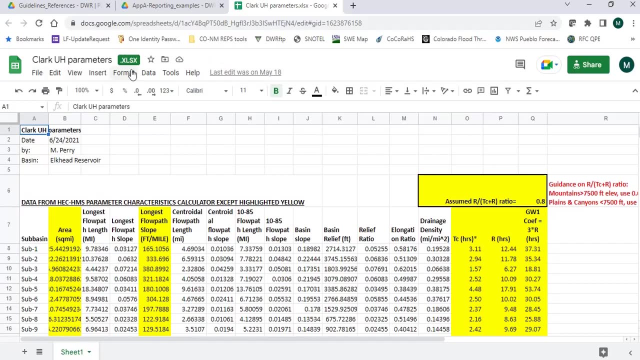 Okay, So we, we provide, we provide a spreadsheet here and you can link to that. Let's just go ahead and open that And again, that is as with the others in the previous properties, section five tutorial, That is, it's opens in Google. 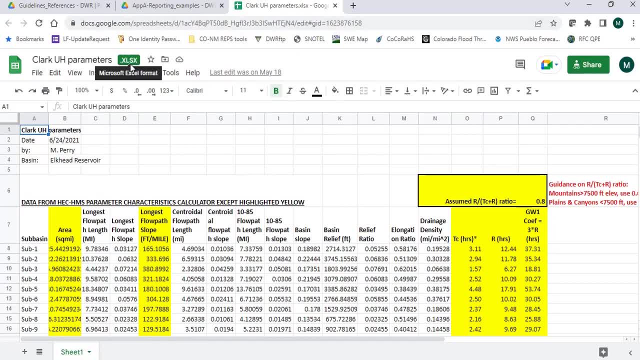 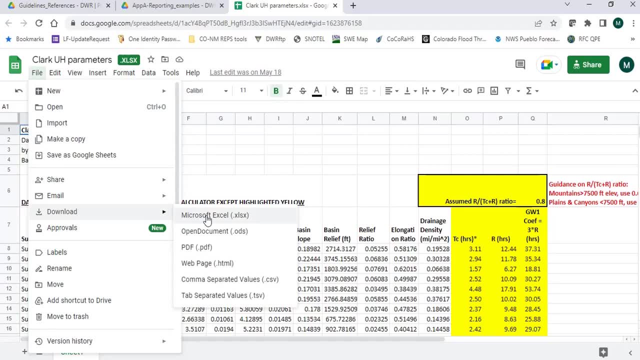 Sheets, but it's actually a HXLS and an Excel format spreadsheet, So you're going to want to use it correctly. You're going to want to download that and save it as an Excel file and then reopen it. The idea with these is they're filled out for an example base. 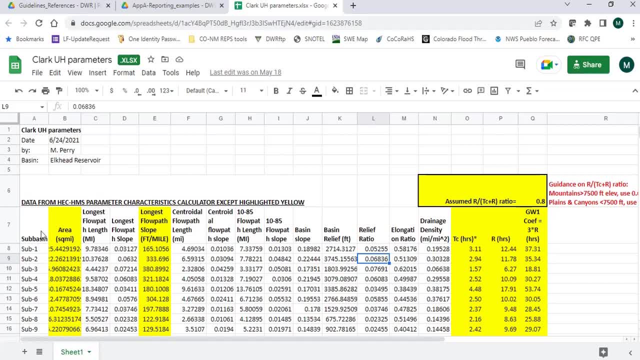 And so you can see. But the idea is, then you can just wipe out anything that's not coded in there. You would just clear it, clear the spreadsheet, and then use it for your. use it for your analysis, your basin. Okay, So let's then go back to the guidance on Clark unit hydrograph parameters. 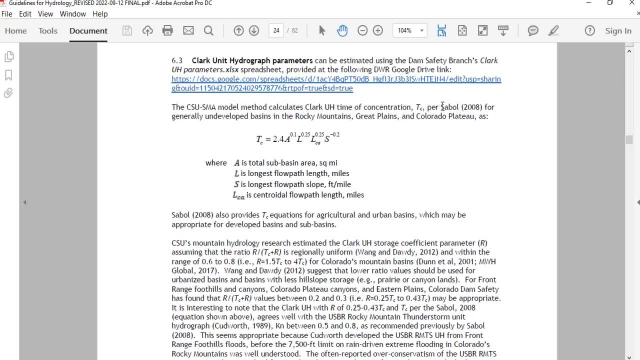 So, firstly, we still again, we're still using from George sables the sable. our previous hydrology hydrology hydrology based response parameter estimation guidance from 2008 had the equation for Clark: unit hydrograph time of concentration. We didn't typically use it. 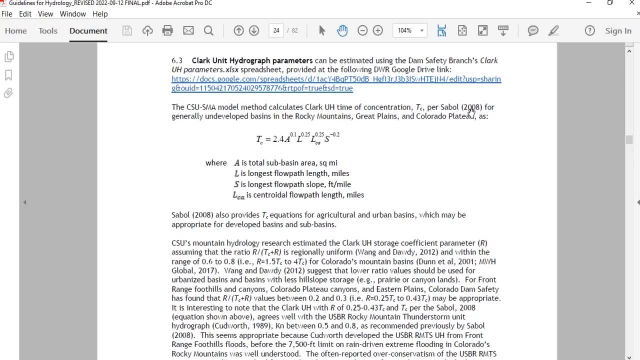 We usually use the guidelines focused. those previous guidance focused more on Cudworth's reclamation, reclamation beer, reclamation USB, our unit hydrographs. We're not using reclamation hydrographs anymore. The new, this new, our new hydrology got solely rely on green and amped. 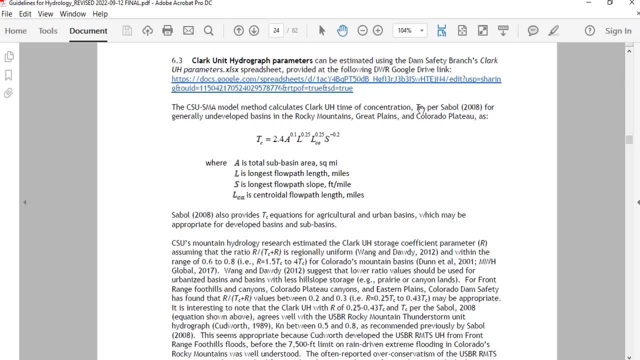 Okay, I think that is as a recommendation. So we're. we just picked the Clark, the previous Clark unit hydrograph. We see in our information from sable This is the general time of concentration equation that our previous guidelines provided for the Rocky Mountains, Great Plains and Colorado Plateau. 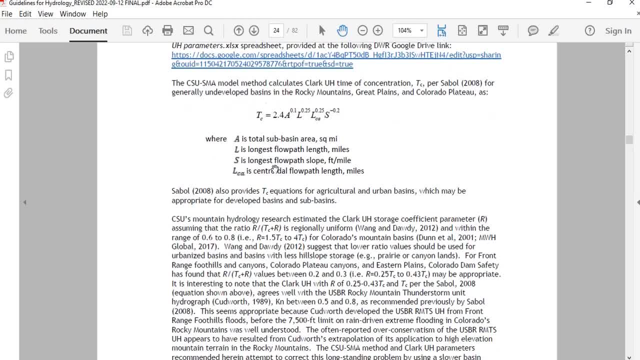 Okay, So we're still recommending that as a starting point. that uses critical time for Clark unit hydrograph as a function of sub basin area length, the longest flow path slope in feet per mile and the length of the centroidal flow path. Okay, That's that. information all comes out of our training. 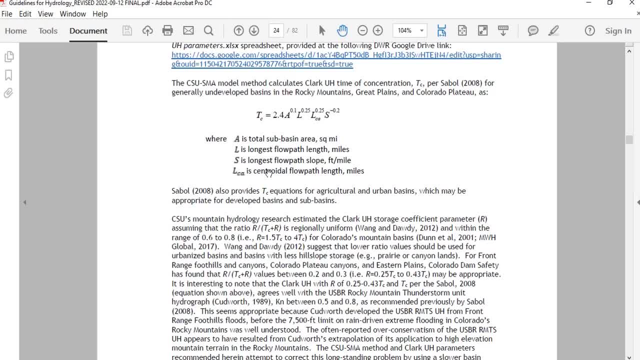 Analysis and heck HMS and we exported the. we copied out the the characteristics, sub basin characteristics table from heck HMS. Okay Then sable does provide other PC equations for specific air, land uses and agriculture and urban development which may be relevant for individual basins and sub basins. 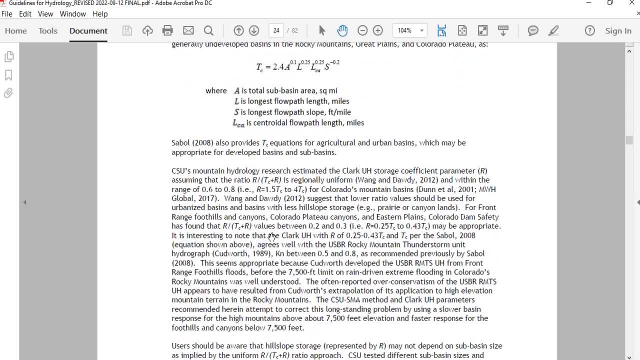 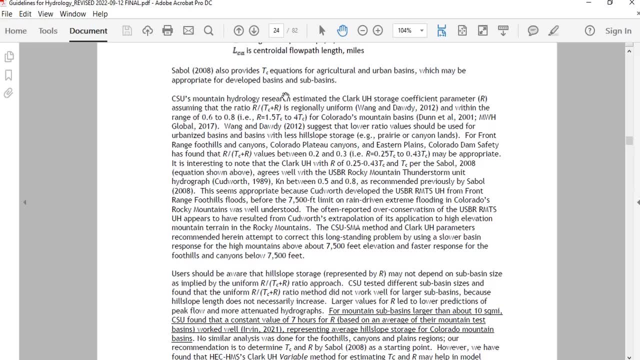 Okay, So now we have guidance here. We're going to look at some of these. Okay, So we have some guidance here on how to get are. so in CSU's mountain hydrology research They use an approach that is has been supported in the literature. where are the ratio of R over TC plus R is regionally uniform. 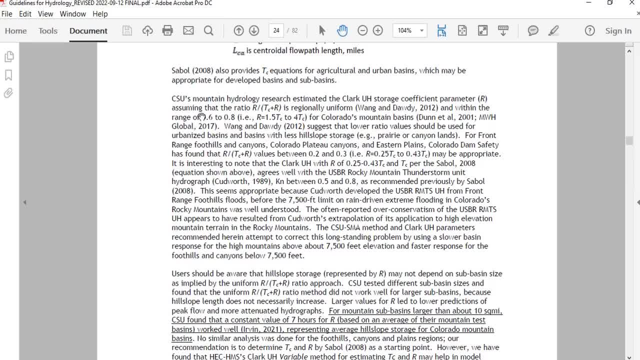 Okay And that's been observed in other studies and for mountains regions They've found studies have shown that that could be about point six to point eight. That's a very slow response Compared to some of the traditional runoff transformations We've used in the past and it probably suggests some sort of shallow subsurface flow as opposed to actual quick flow search true surface runoff. 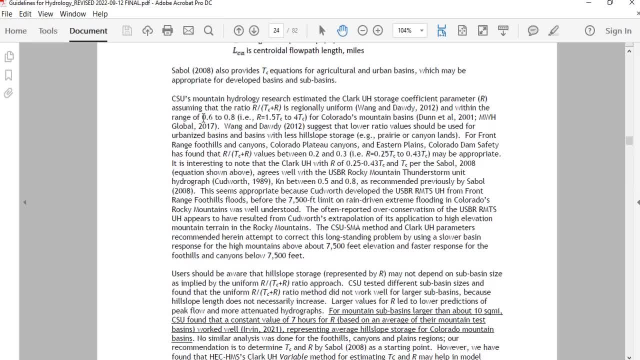 It's probably like an inner flow suggests an inner flow or a shallow subsurface flow, and that's consistent with other research that's shown that usually in mountain and forested basins You don't see actual surface runoff, even in intense thunderstorms. Okay, 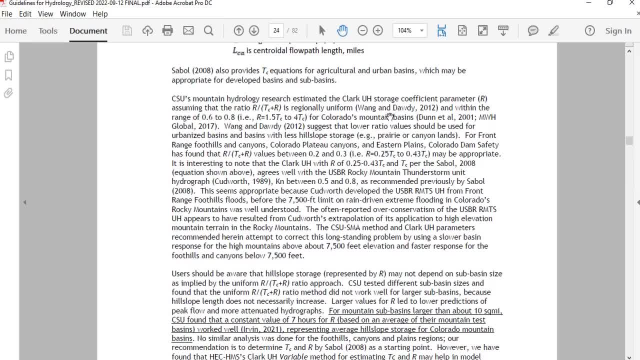 So that the ratio of R over TC plus R of about point six to point eight- It's that that's equivalent to saying R is about 1.5 to 4 times the time of concentration- Are represents. you can think of it as representing hill slope storage. 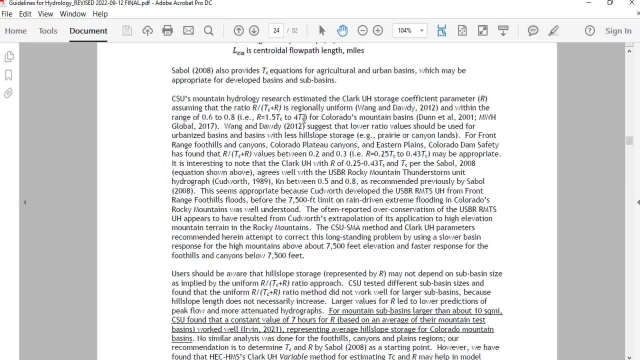 TC is the actual channel network storage. Okay, Now next that's for the mountains. This are point six to point eight. Now next is for the plains, the eastern plains, foothills and canyons, So that can be in the west slope canyons, Colorado Plateau or the Front Range Canyons. 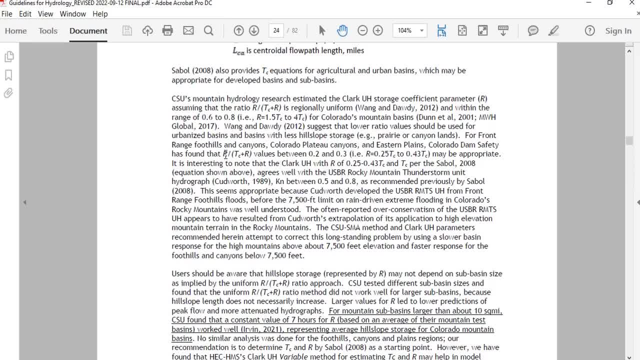 We see something very different. So there we see what we've seen. This wasn't covered in part of the CSU mountain hydrology research. We've done many example studies, test studies here For beta testing on our own in Colorado Dam Safety and after many studies in those plains and canyons, foothills, regions. 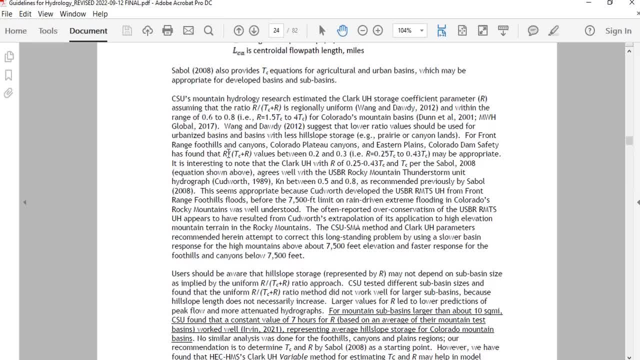 What we've seen is calibrating based on comparison to the observed flood record. We've found R over TC, plus R ratios need to be closer to point two to point three, Which is equivalent to, can be just rearranged to R, that hill slope storage being about one quarter. 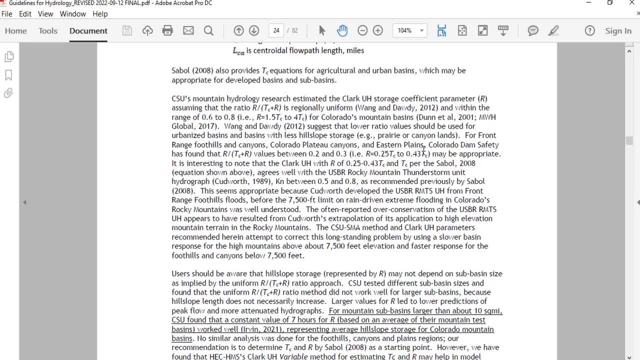 To point four. so point two, five to point four, three times the time of concentration, So that what you're seeing there is much faster right, Much faster, much less, much less hill slope storage and a much faster, flashier Clark unit hydrograph. Okay, 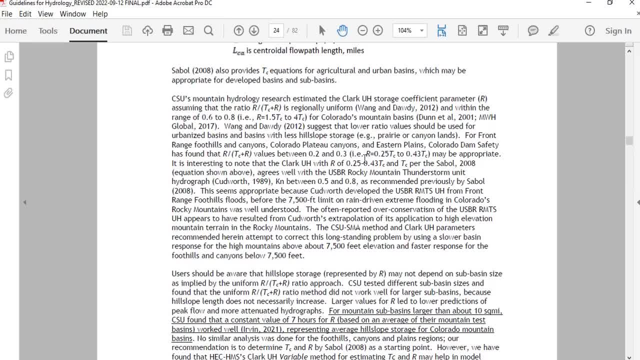 Now the interesting thing is is that when you take those quicker values, What you find is that in that you put them into Clark unit hydrograph, You find a unit hydrograph that compares pretty well To the old Bureau of Reclamation Rocky Mountain thunderstorm unit hydrograph. 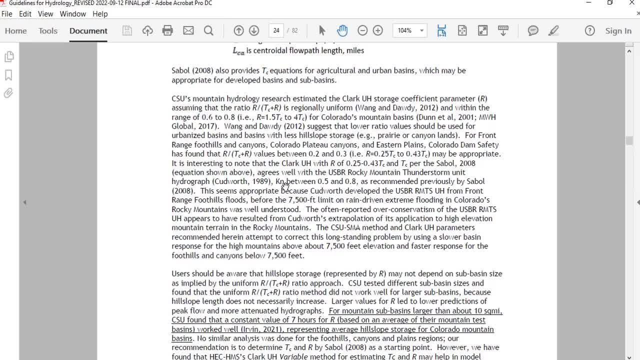 With the previous, with our previous guideline recommendations of a KN about point five to point eight. Okay, That seems appropriate. What the guidelines here say is our new guidelines say: is that seems appropriate Because Cudworth Reclamation mainly developed those USB, our unit hydrographs from Front Range foothills, floods, 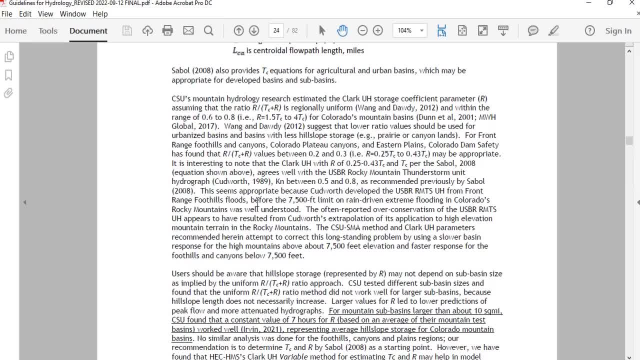 Remember, Cudworth cited a lack of general lack of experience, Extreme precip and flood information for the Rocky Mountains, And that's why that's what we propose throughout These guidelines- has been some of the source of error in the past and overestimating mountain and West Slope floods. 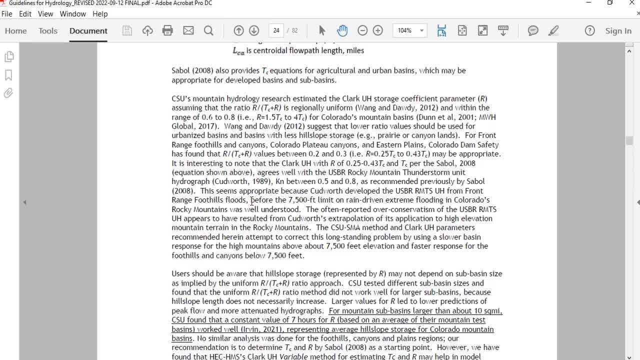 It's just that there wasn't data and there was a general extrapolation of Front Range foothills and plains, rainfall and floods, And here runoff transformation to the mountains and West Slope where may not have probably wasn't appropriate. Okay, So it makes it seems to make sense that, if you, what we found is these faster. 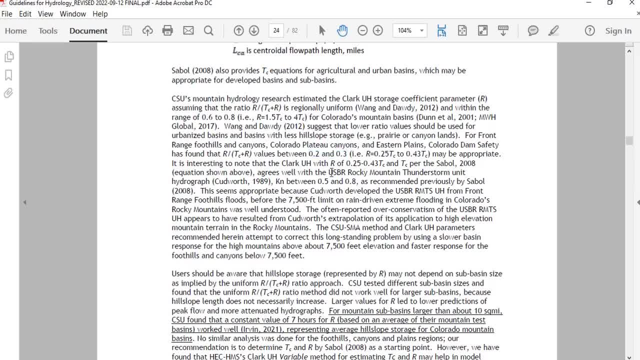 Less hill slope storage faster. Clark unit hydrograph actually compares pretty well to the old Reclamation Rocky Mountain thunderstorm unit hydrograph And I'll show you below. It also compares well if you just use the straight TC and our equations from from our previous stable guidelines. 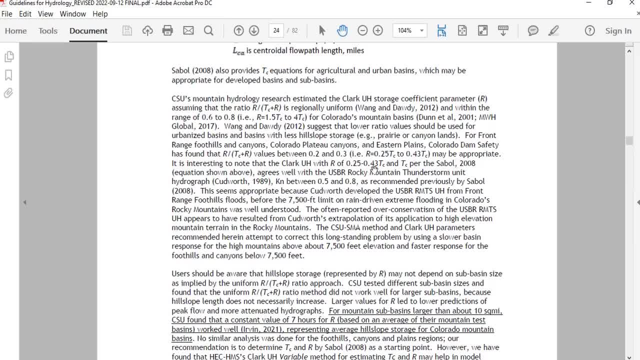 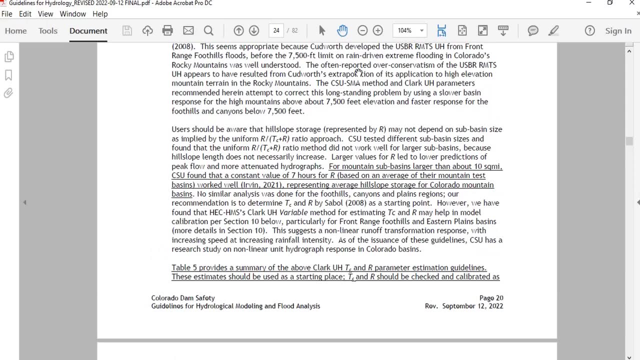 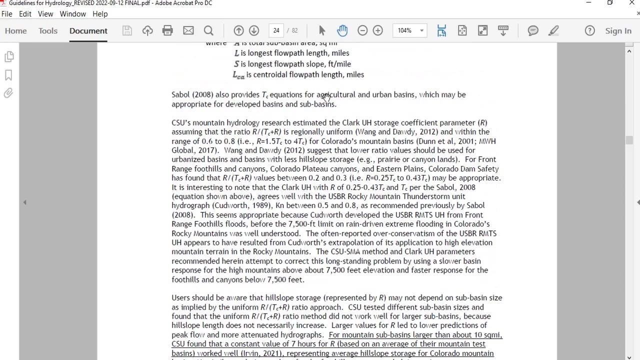 The previous 2008 hydrology guidelines. So that's what we're recommending for the plains, Eastern Plains, Colorado, Plateau Canyons and Front Range foothills and Canyons. Okay, Yeah, So that's the, that's the the advantage, and why we've moved to, why CSU and their mountain hydrology research moved to the Clark unit hydrograph, is because these variable parameters. 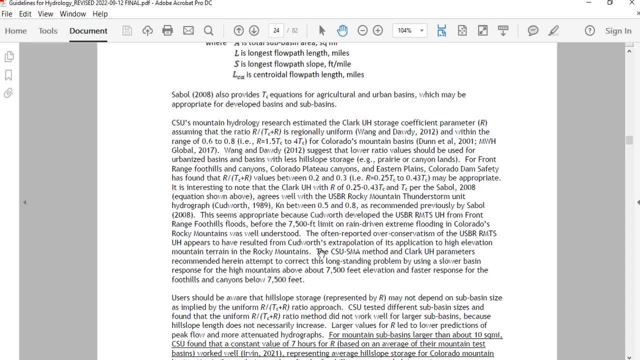 Allow us To better represent different types of runoff. So it's not all just modeled as a kind of a quick flow hydrograph, the way it would have been from using the Reclamation Rocky Mountain thunderstorm hydrograph. Now we can calibrate the observed. 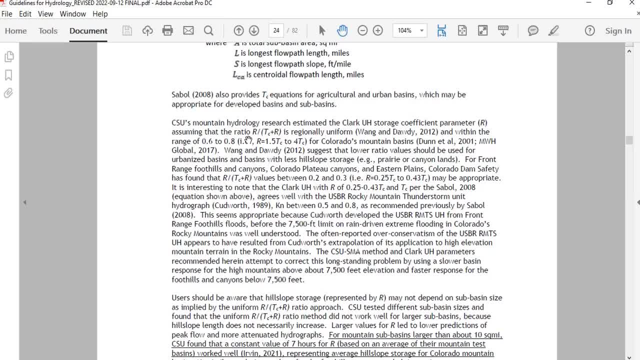 We have parameter estimate, recommendations, guidelines and then we can calibrate to observe flood records. by calibrating this RNTC in Clark unit hydrograph We can produce different types of surface runoff, Like like quick flow from the Eastern Plains, foothills, or more like subsurface shallow flow or interflow in the mountains, using these longer, slower Clark unit hydrograph parameters. 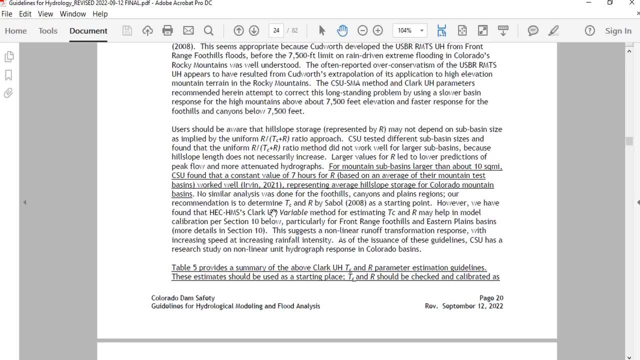 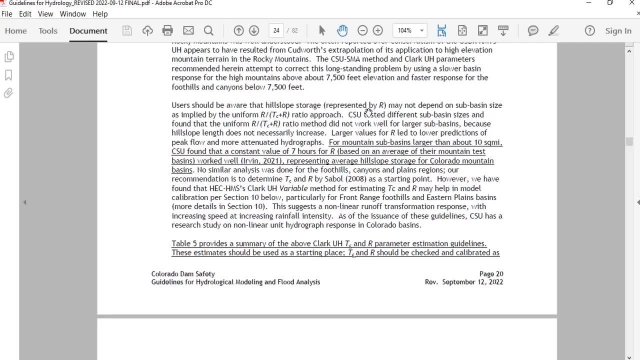 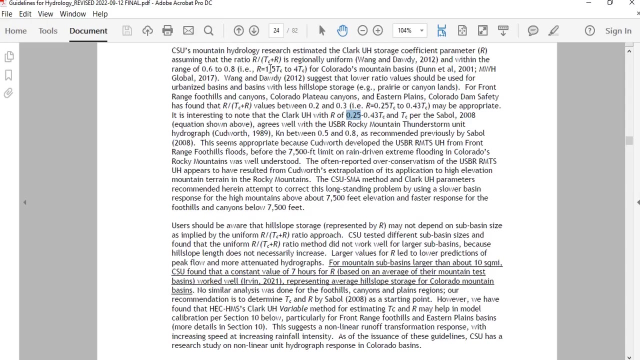 Okay. So the next thing in the guidelines is that the users should be aware that are may not strictly depend on TC The way this Uniform ratio approach Implies. Okay, So if you're using or get remember this, this just are this ratio just can be a rate rearranged to have R as a function of TC. 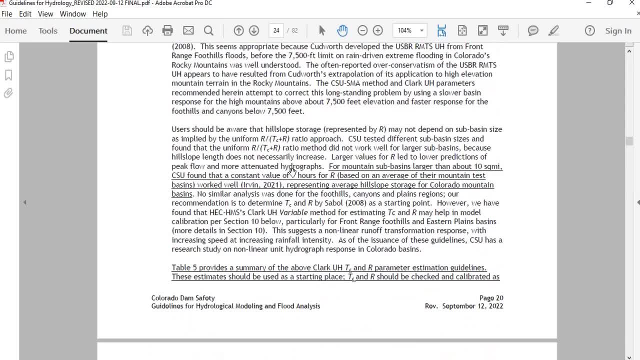 Well, that implies that the bigger TC gets, the bigger R gets. That may not be true as you get to bigger sub basin areas or big basins, because ours hill slope length does not what CSU in their research proposes, that hill slope length does not just continue to increase. 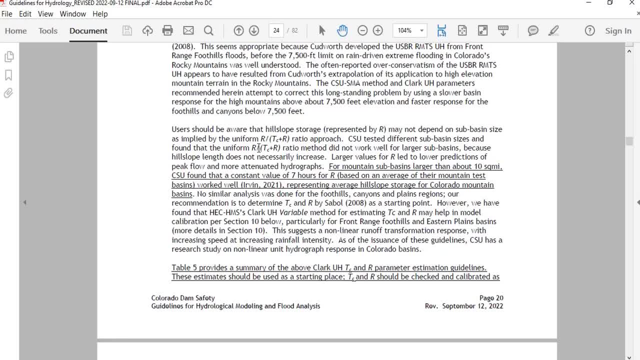 Infinitely. it has some finite length. It's a function of the geography and geo morphology. So what they said is what they found is that when they use too big a basins, this are not too big, too much hillslope storage and they under predicted. 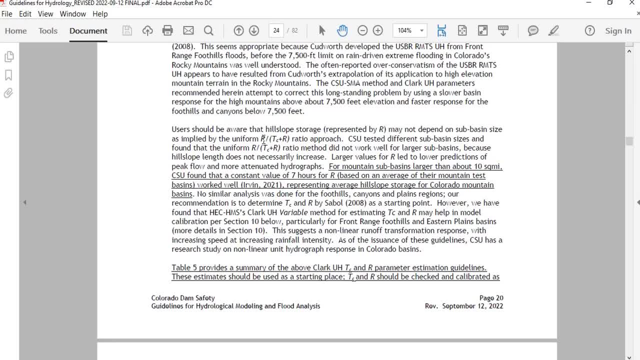 They under predicted runoff, peak flows. Now, I've said before, using our method here in the guidelines We do have the additional step of calibration checking, reasonableness checks against the observed flood record and we have the opportunity for calibration, calibration. So we don't need to get maybe as worried about this because we can recalibrate. 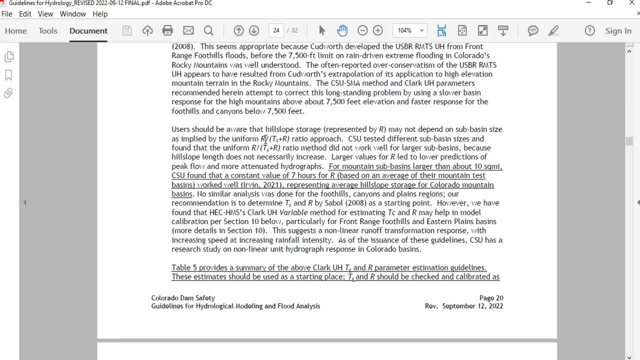 the Clark unit hydrograph later in this. It's covered in Sections 9 and 10 of the guidelines. But just to be aware that what CSU found is when they use too big of subbasins, TC gets too large. Well, not that TC gets larger. R gets too large as a function of TC. 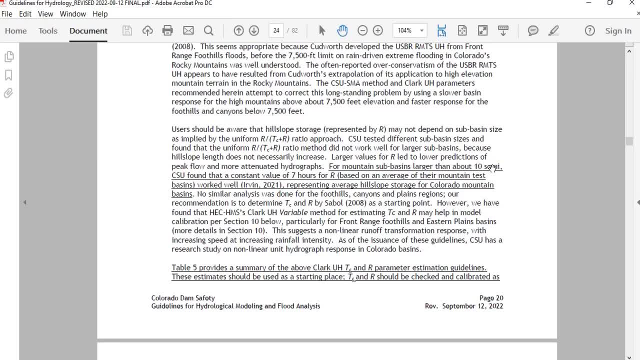 So what they proposed is when basins are larger than about 10 square miles. just to use a constant R, which they calculated as their average from their test and verification basins, they found about seven hours for R, So that would be like an average or representative. 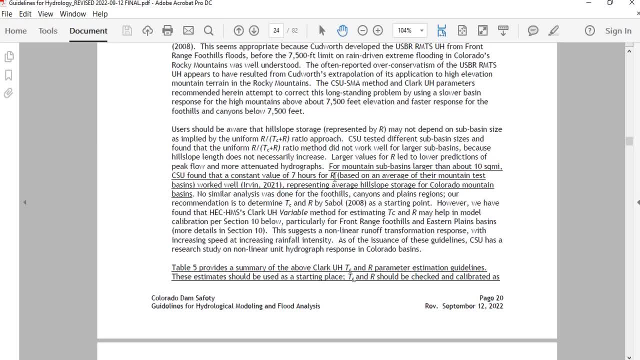 hill slope storage amount for Colorado's mountains Doesn't say anything about the plains. In their research study they did not do plains and foothills and canyons, And so we don't have equivalent guidance on that. but I'll show you how we would. 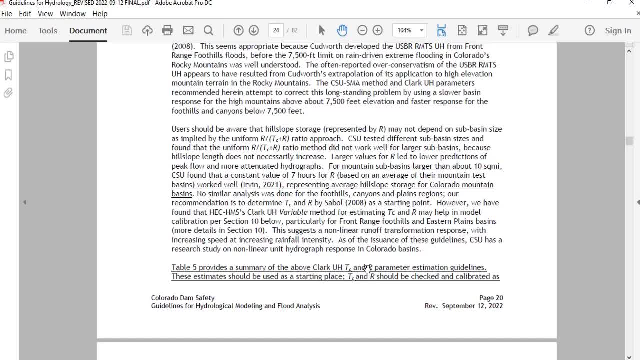 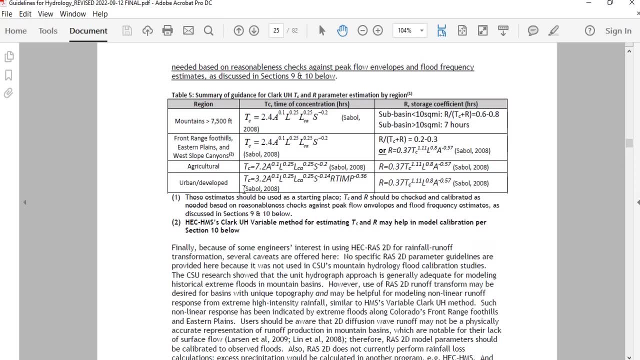 recommend handling the plains, canyons and foothills. Okay, so let's go to Table 5. And here, hopefully we have, after this written description, we have a concise summary of the Clark unit hydrograph TC and our parameter estimation guidelines by each region. So for 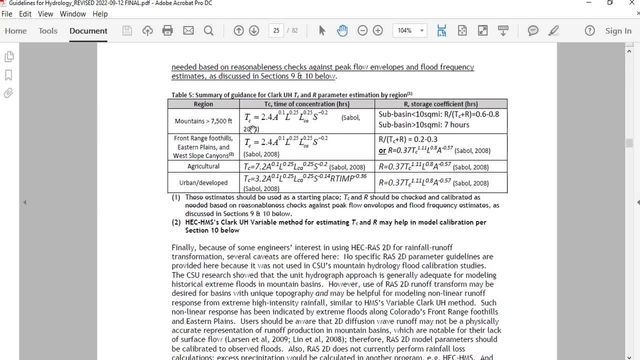 the mountains. we said: start with TC from the Sable 2008 guidelines for the mountains and plains regions. We said: start with TC from the Sable 2008 guidelines for the mountains and plains regions. And if your subbasin's size is less than 10 square miles, then we recommend starting with. 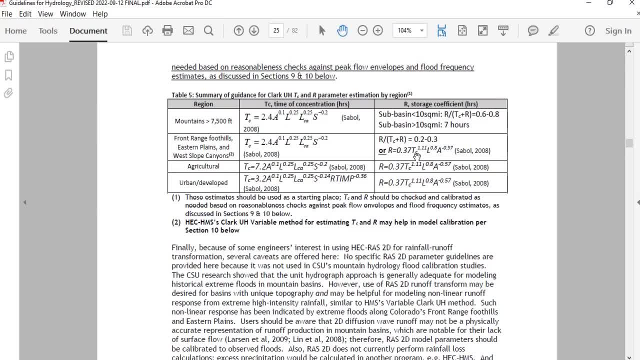 this R over TC plus R ratio 0.6 to 0.8 for this mountains region. If you get into bigger subbasins then we recommend just using this constant seven hours as an average hill slope length, storage length or time from the CSU Mountain Hydrology Research Study. 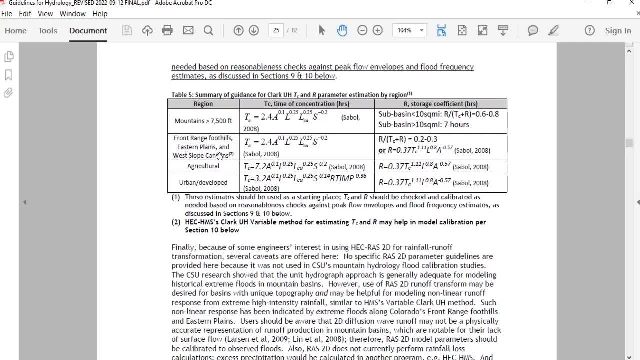 Now next for the Front Range: Foothills, Eastern Plains and West Slope Canyons. Same equation, Same, starting with the same TC equation from our previous 2008 hydrology guidelines, But then R over TC plus R, quicker ratio of 0.2 to 0.3, and like we talked about that above, 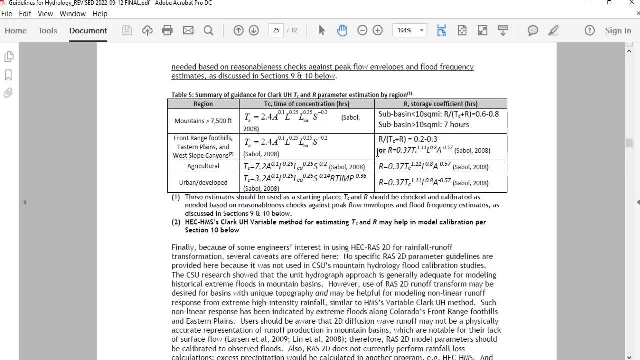 much quicker flasher Clark unit hydrograph or just bypass that altogether. And what we found is it's pretty similar to just using our previous guidelines: Sable's 2008 equation for a Clark unit hydrograph R. So if you use this equation from Sable, you're going to end up with a. 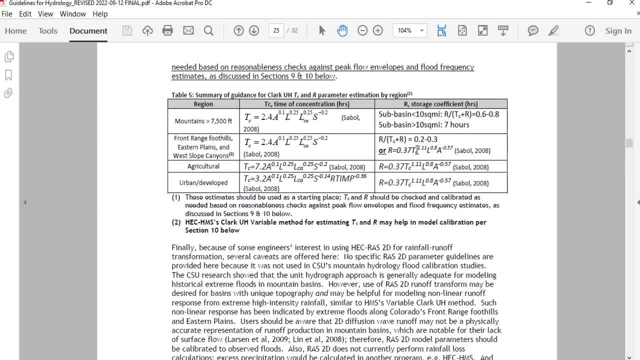 much faster. Clark unit hydrograph, and it's going to be about equivalent to this R over TC R ratio of 0.2 to 0.3.. So you can use either of those. So there you go Now for the specific again. 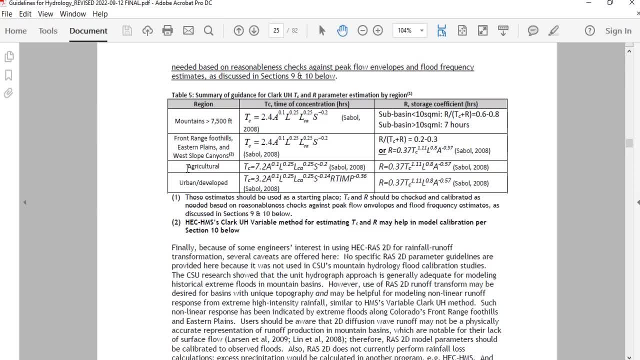 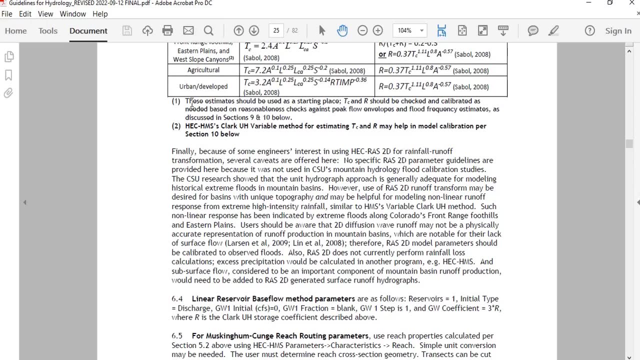 we said, specific land uses case by case, basin by basin. basis: Sable 2008 provided TC and R equations for ag lands And for urban or developed lands. Okay, Again, here we talk about that in these footnotes to. 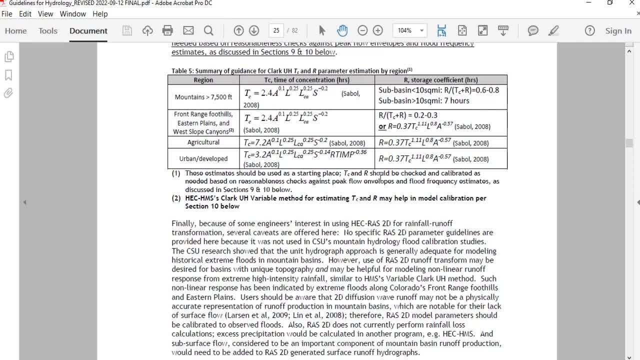 table five that these are can be considered a starting place. And we have the opportunity in sections nine and 10 in our guidelines for checking against results, against model results, against the observed flood record and for calibration. So these can all be calibrated as needed to match peak flows, the observed flood record And then what we'll talk. 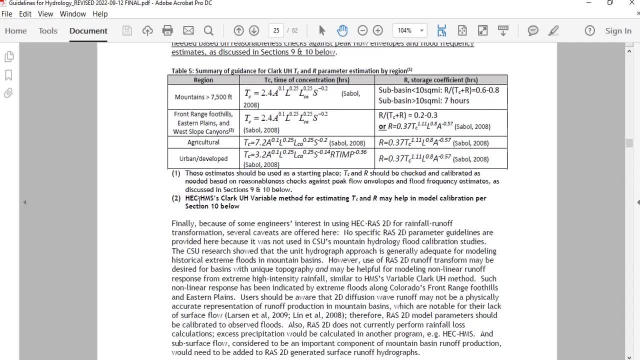 more about? is that later? is that what we have found is that to match the observed flood record on some of the extraordinary extreme floods that make up the peak flow, the peak flow envelope for the Eastern Plains and Front Range foothills, we need, we've needed to use the Clark variable. 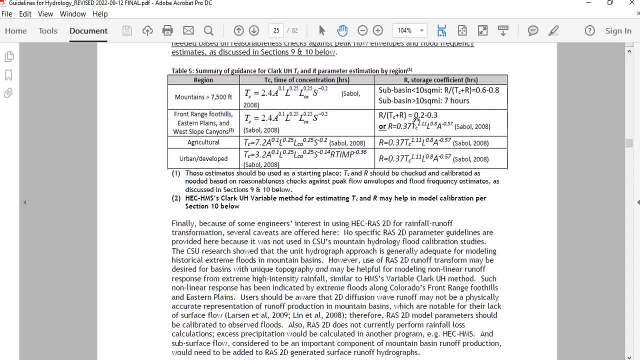 unit hydrograph method, So that use these as a starting place, But in the end, in our checking and calibration steps in sections nine and 10 of these guidelines, we end up moving to the variable unit hydrograph method, which creates a nonlinear response to as rainfall intensity. 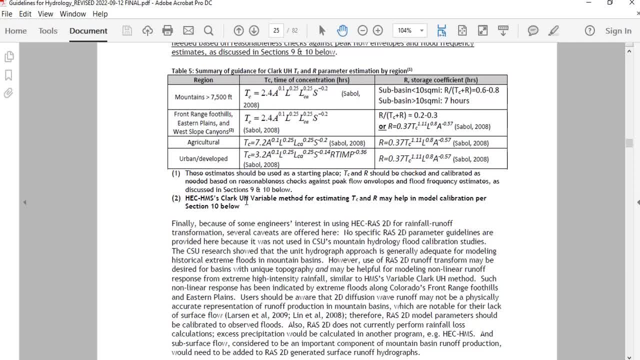 increases. And that is in fact what we seem to see in a front range runoff response: the large differences between some of the more frequent floods, like 100 year and thousand year, and then the floods of record which represent kind of the 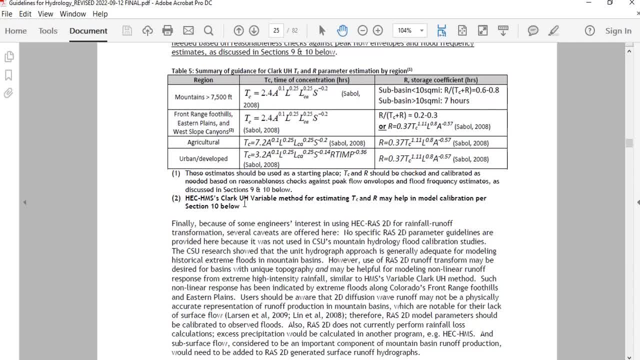 extraordinary floods like the Cherry Creek 1935, Jimmy Camp Creek 1965, things like that. We've had to use the Clark variable unit hydrograph method and CSU currently has a research study. We're collaborating with them on looking at nonlinear response in runoff transformation unit hydrographs. in some 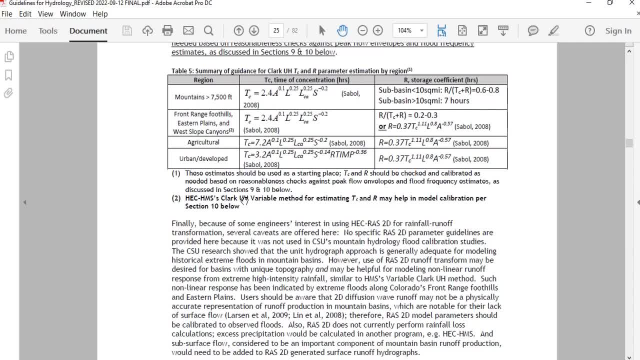 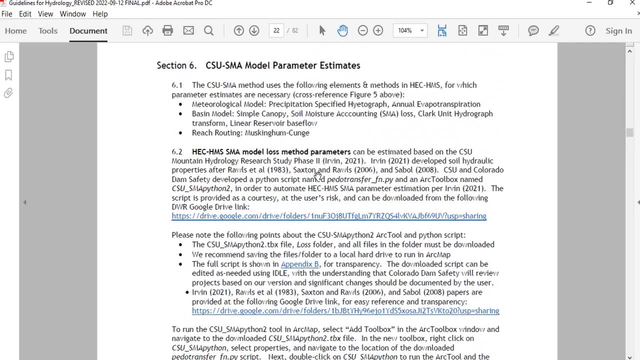 of these historic front-range floods. So in the future we hope to have better guidance or more, I guess, more support and more research supporting that use of a nonlinear, nonlinear response, if that's what we they find is appropriate. Okay, so now let's go to the actual CSU SMA Python script in our 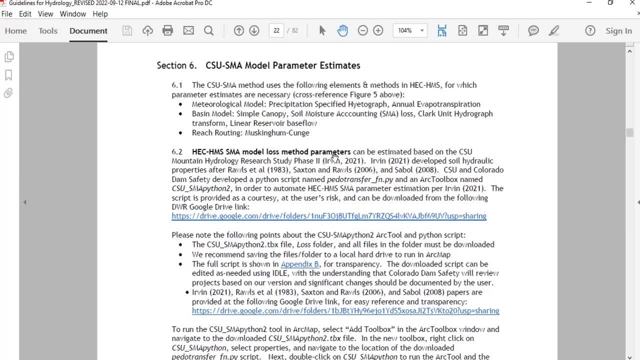 toolbox. Okay, so this is where this hopefully gets easy. Hopefully everyone feels comfortable at this point- a little bit at least anyway- of how the parameters are calculated and really where that, where the, where the estimation methods, the parameter estimation methods come from. So if you 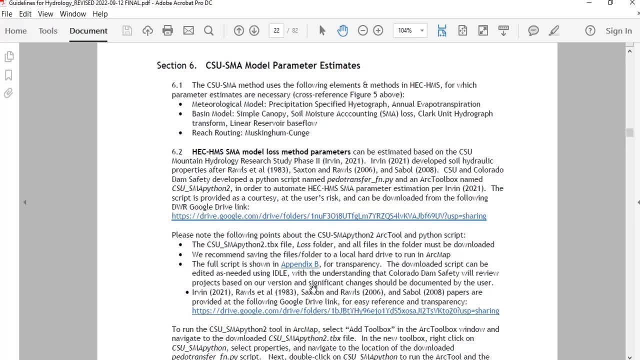 want to go to these references yourself and read as much about Rawls, Saxon and Rawls, the old Sable guidelines and Ben Irvin's master's thesis as you want to, but at least you know where they come from and how everything's calculated So. 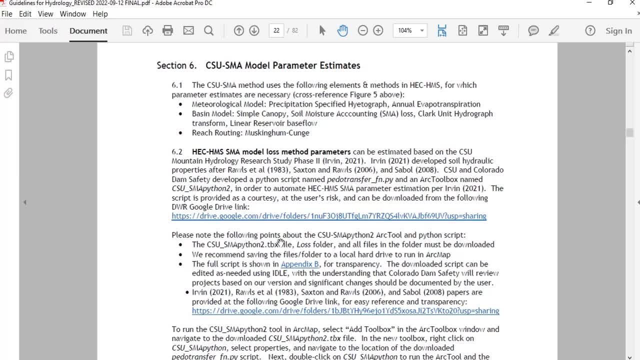 now let's just go to the arc toolbox and actually calculate stuff and get, get some parameter estimates for our HMS model. Alright, so we have this Python script that essentially CSU wrote as part- basically they wrote as part of the mountain hydrology study. we kind of tweaked it and made it a little more. 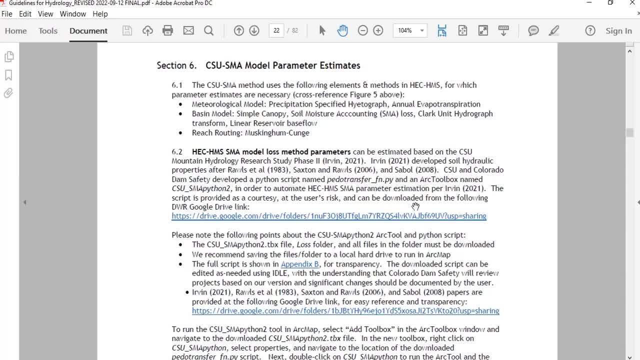 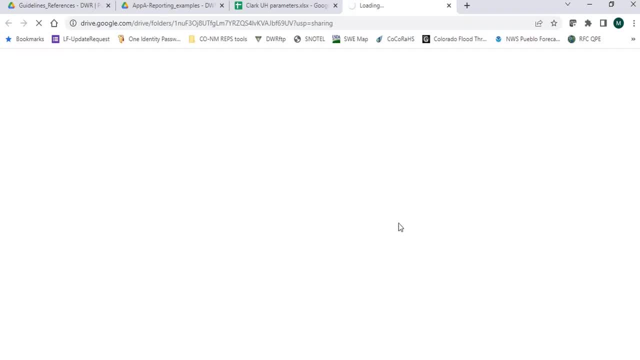 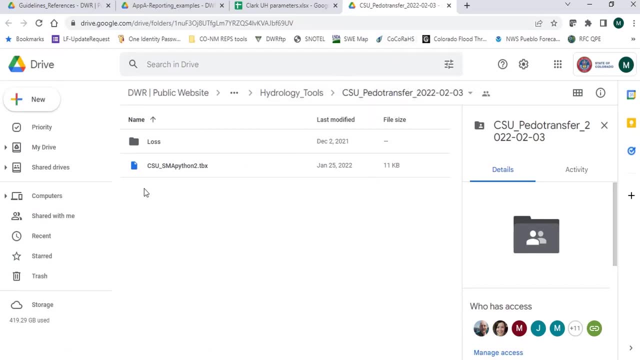 user-friendly and then turned it into an arc toolbox, so that's what we're gonna go to here. there's a Google Drive link. you should be able to pop that open these. the links are all embedded in the PDF guidelines, so you just click on that. it's going to take you to our damp safety Google Drive, where you'll find 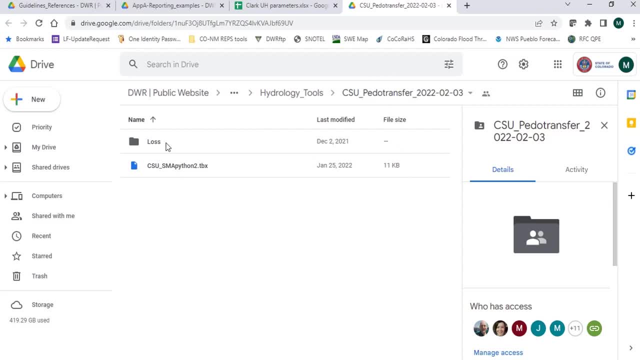 this CSU SMA Python arc toolbox. What you need to do is grab everything here. so there's this loss folder and the CSU SMA Python 2 TBX. is that our toolbox? and in this loss folder there's other information, including the actual Python script. Okay so. 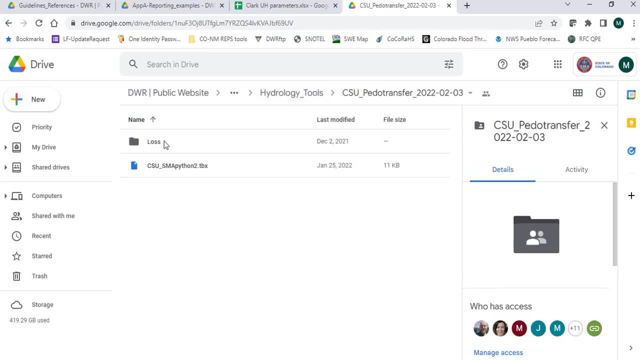 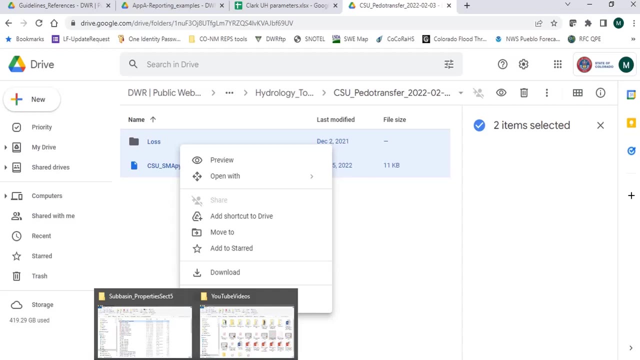 I've already done it, but if you were to doing it for a new for the first time, you just grab those and download all those files, put them again. we recommend everything just as a standard guideline here. we recommend you do every recommend, standard recommendation. recommend you put everything on a local C Drive or 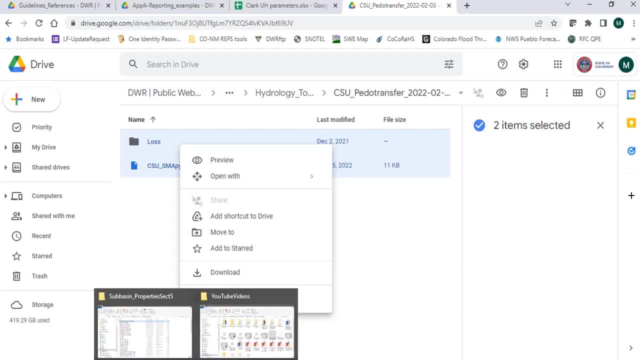 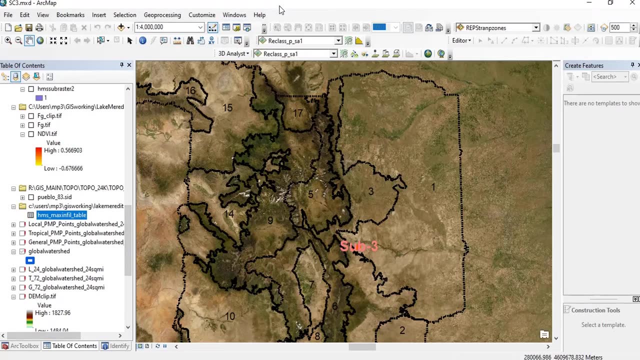 hard drive for use in arc. with arc map GIS, it just seems to work better. we have less, less problems. Okay, so let's go to the next slide. Let's go to arc map. I'm using- or, yeah, arc map, I'm using arc map 10.4.1. that's what. 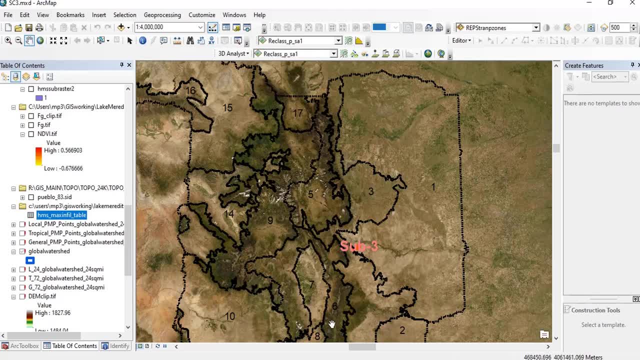 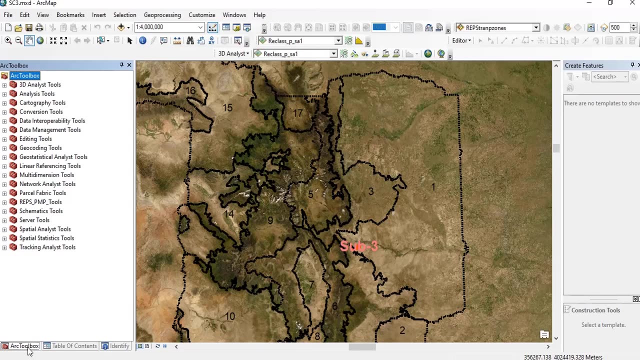 the guidelines were developed using. we've had people test this up through, I believe, arc map 10.8 or so and it has worked for that. we did do some changes to the Python script to accommodate that, but anyway, that's where we're I'm using. 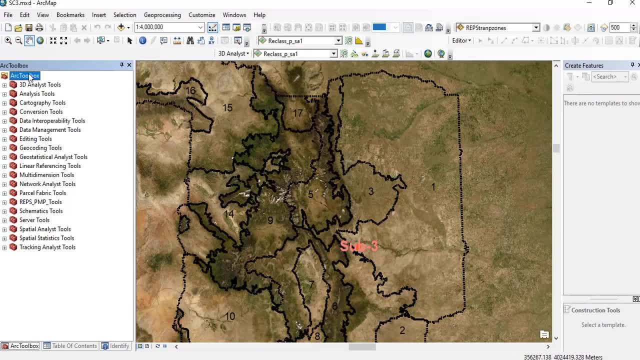 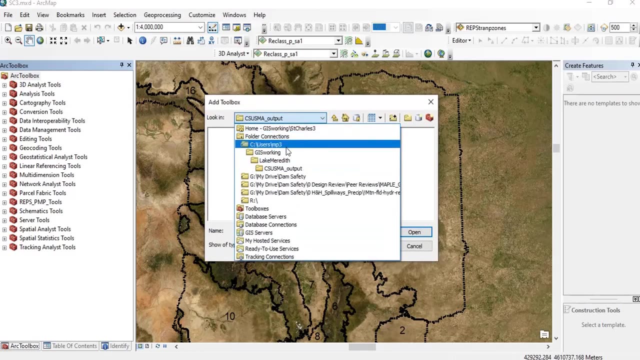 arc map 10.4.1. now, okay, so to add this, this CSU SMA Python arc toolbox. go to arc toolbox, open that right click and you want to add a toolbox and then we're going to go to your local C Drive, hard drive, where you've saved it and I have. 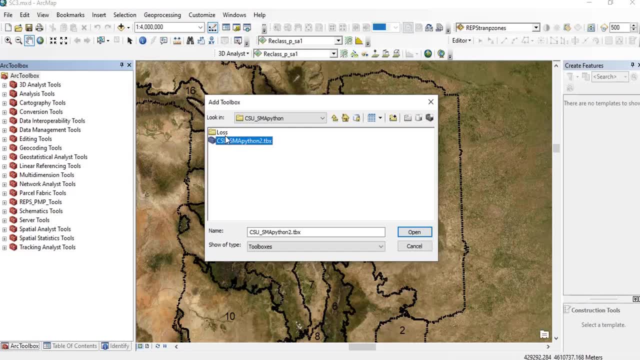 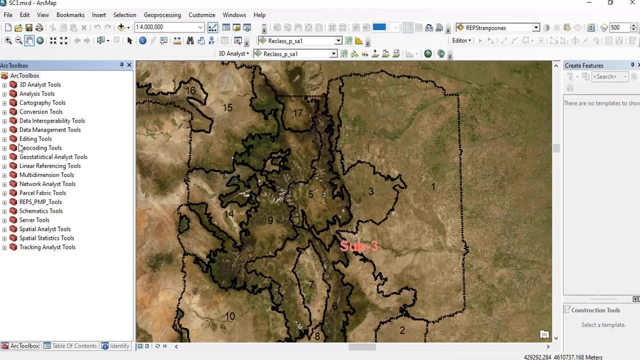 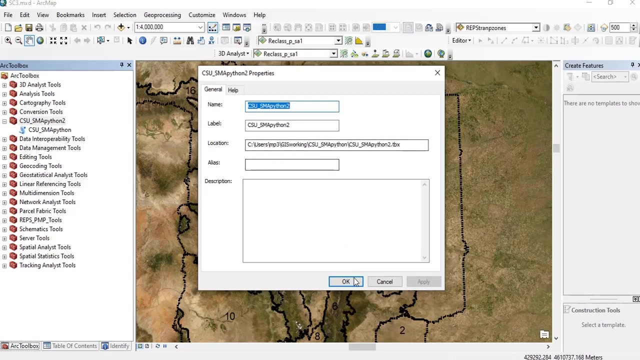 mine just here and I'm going to grab the TBX file. okay, and it's going to. just inserted that there as a tool, I guess in alphabetical order, and what I'm going to do is I'm going to check that is has that located on my hard drive and then I should have. I think in general it should. 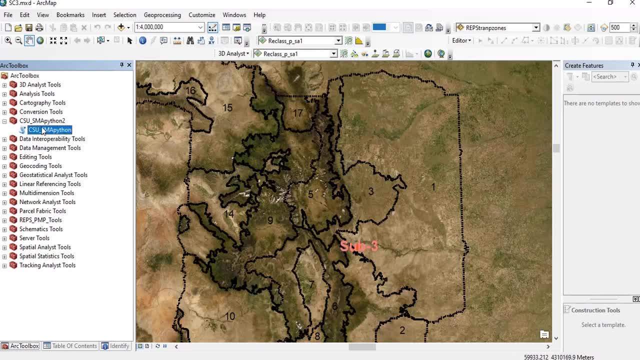 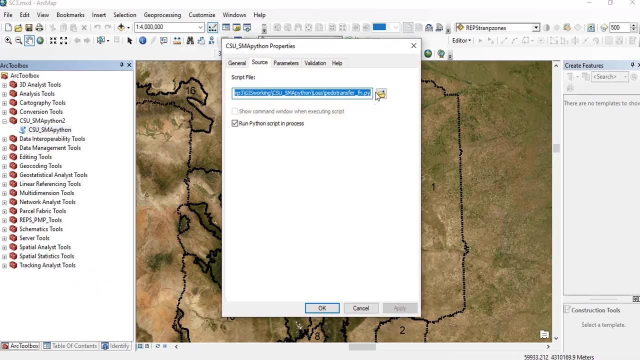 be linked relative to where the script should be set up, relative to where your toolbox is located, so it should come in with the script. if it's not there, you have to go. you may have to add the script and go looking for it, like in this case. we tell it that. 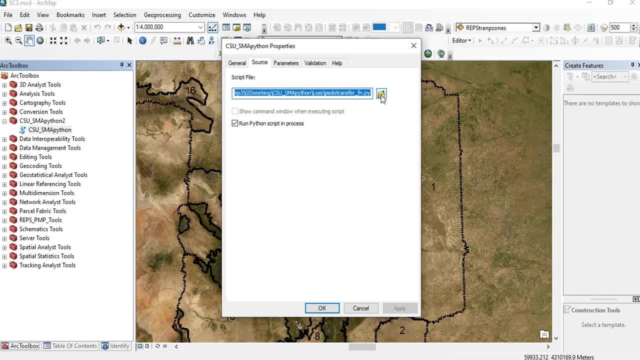 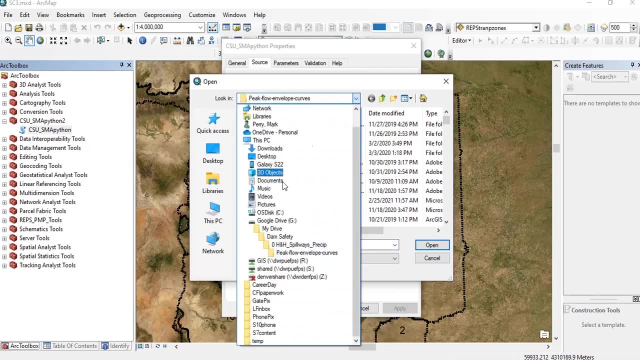 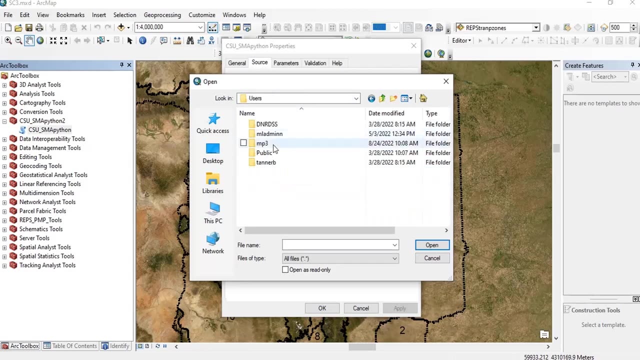 the script. it knows that this I didn't have to tell it, but I could tell it that the script is here in that same, in that same C Drive folder where we download, that we downloaded it to- so I had it- my userscom and GIS folder, CSU, Python, and that if I open this loss folder I find that that P? 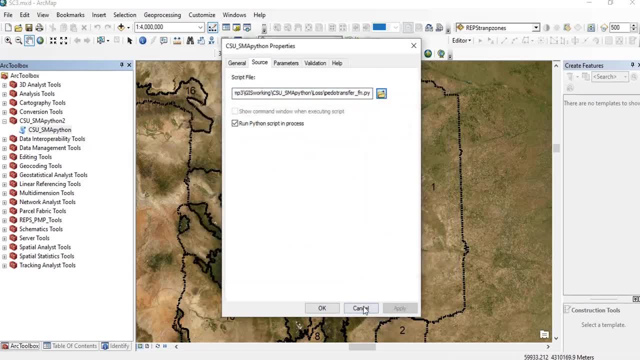 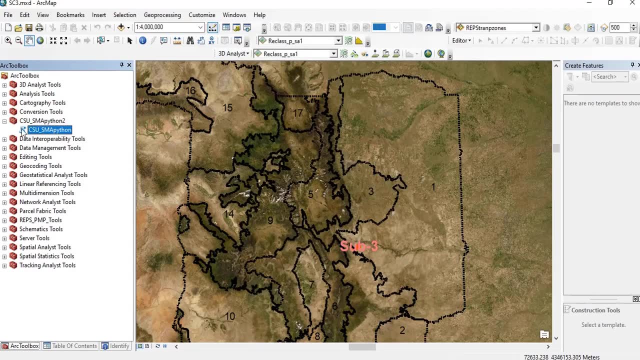 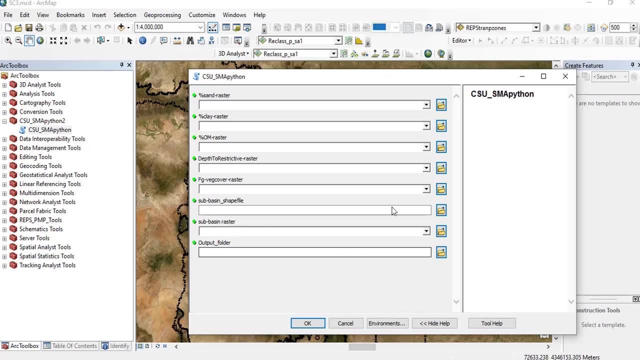 wise that Python script. okay, but it already came in knowing that it's there. so all I would, all I have to do, is now double click on this script and it opens this GUI or user interface. okay, and so I believe I went over this briefly, very briefly in section 5, but it's a pretty pretty for calculating our subbasin. 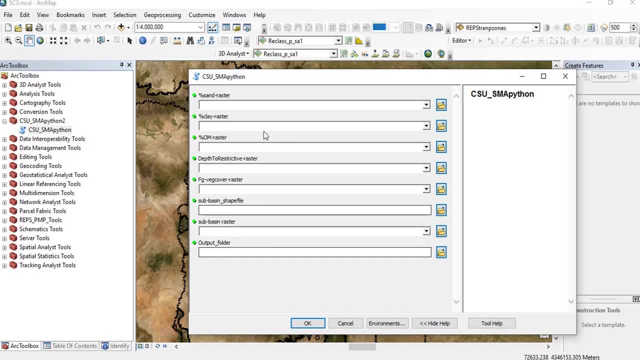 properties there as far as our sub basin soil properties. but it's a pretty easy user interface. we're just going to go looking for that raster, that g nets go raster sand and these need to be located there, need to be loaded into your map project and they'll just appear here as raster project rasters that you can. 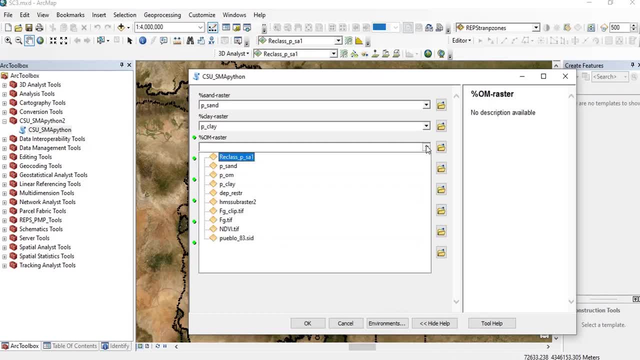 select. So then clay the organic matter raster and the depth to restrictive layer raster, this fractional vegetative cover raster, tiff image that we created, that we calculated using the raster calculator, and then we have our sub basin shape file, which we created from, exported from heck HMS in section 5 tutorial, and here it's a shape. 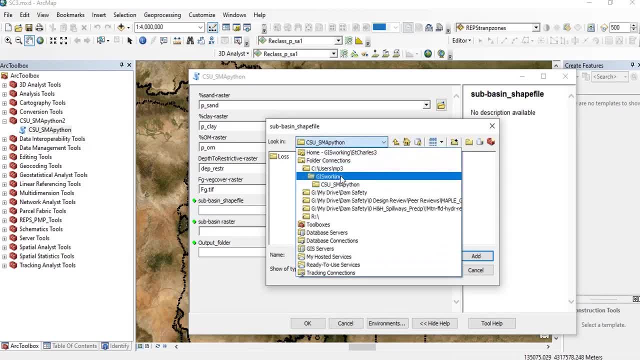 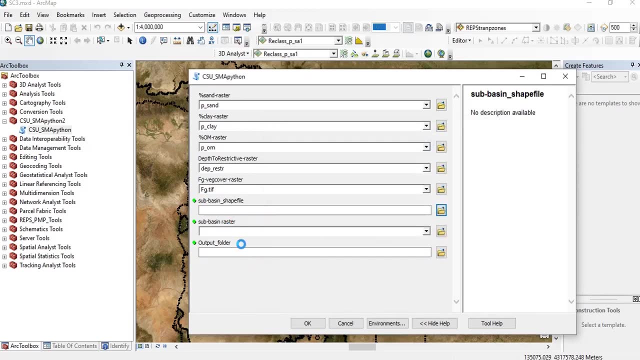 file Now in section 5. we actually are going to go looking for that and that's in my my on my C drive, in my project folder here over the dates, HMS subs. and then, if you recall, in section 5 we had to create a raster with the convert, this sub basin. 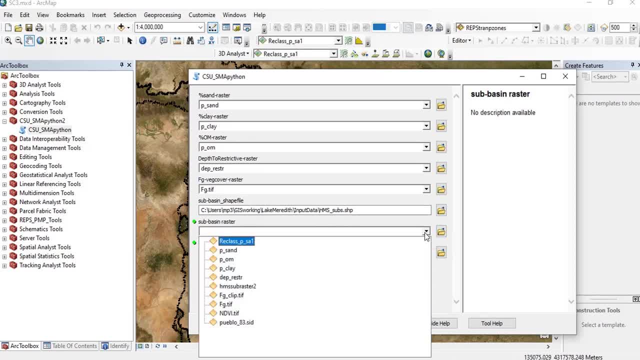 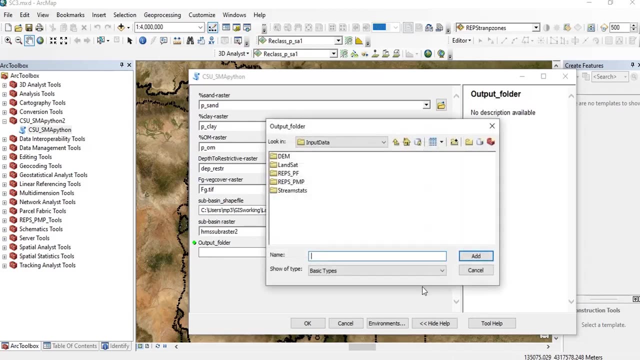 shape file into a raster image as well. it's, that was one of the changes that was needed to accommodate, to make this work in newer versions of ArcMap. but regardless, just then to add that and then create an output folder, and we want to do this on our again, on our local C. 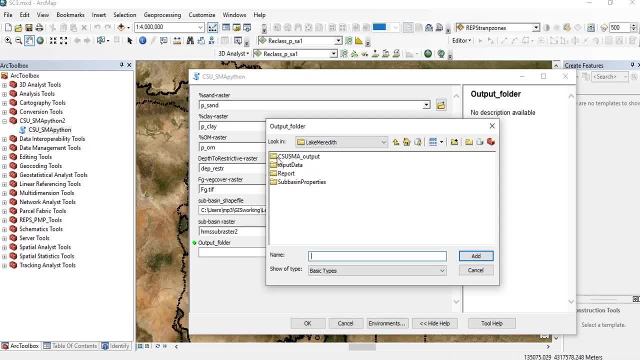 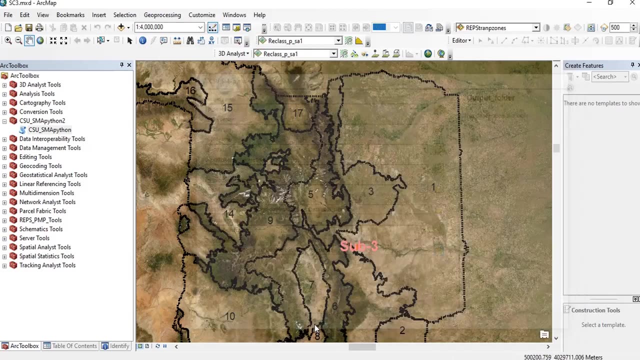 drive here. so I already had, I've already run this. I created that CSUSMA output folder on my hard drive, my C drive, in my working on my project folder and and then it's going to dump all of this output to that folder, okay, and show you what what it does. so you get this interface screen. 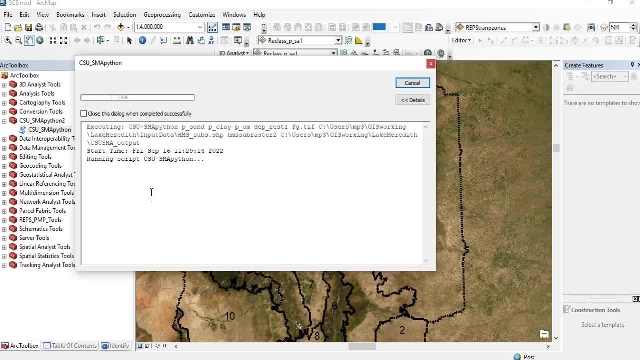 while it's running and it tells you. it does tell you a little bit about what it's doing, as it's calculating the soil properties, sub basin soil properties and then sub basin hydraulic soil, hydraulic properties from Saxton and Rawls. right that we went through like the fractional 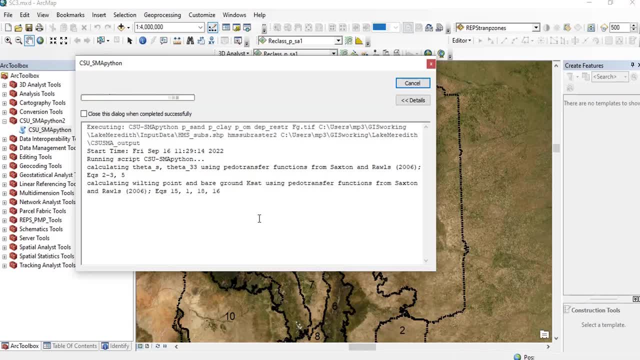 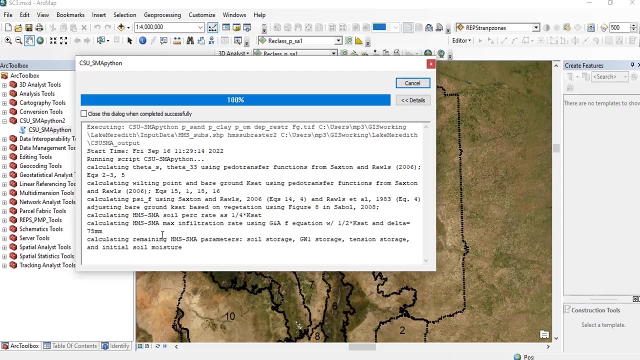 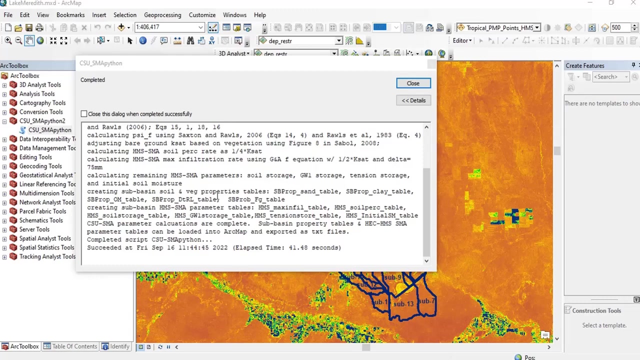 fractional water content saturation, wilting at, field capacity, wilting point, case, that adjusted vegetative, adjusted case at, and then water content, inches for saturation, field capacity and wilting point, and then it's going. now it's going using those to actually calculate the heck, yeah, the heck, HMS SMA loss method. 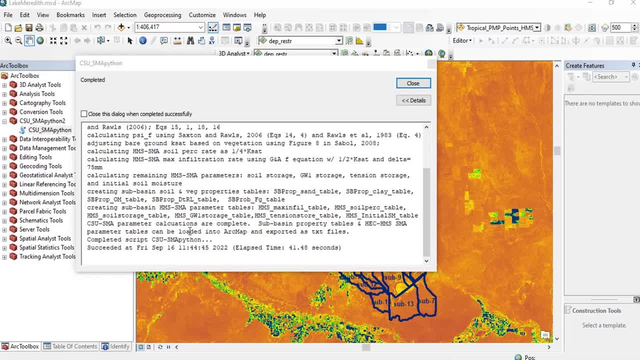 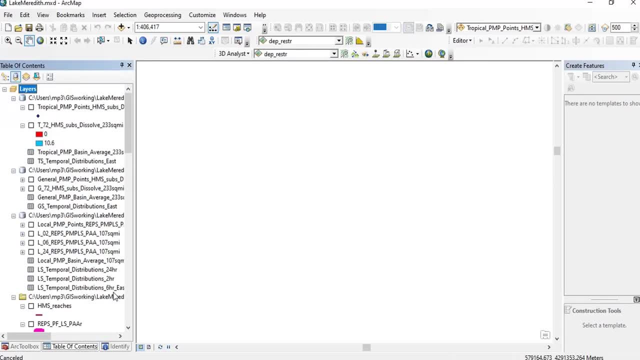 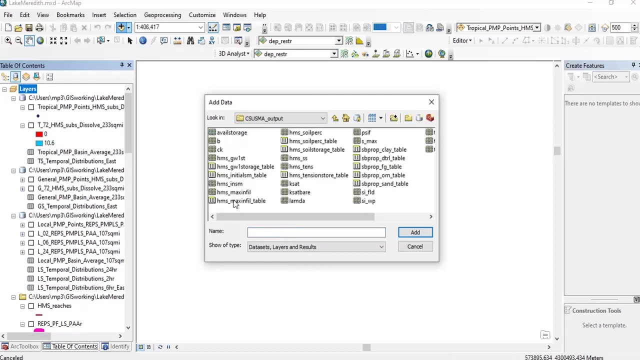 parameter estimates. okay, so it's completed, it is generated, all those parameter estimation tables, so let's take a look at those, go back to our table of contents in our project and navigate to on the hard drive, my, my C Drive, my project folder and that output- CSUSMA output folder that I created. 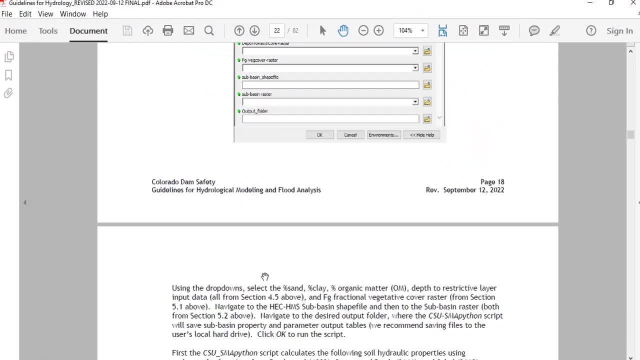 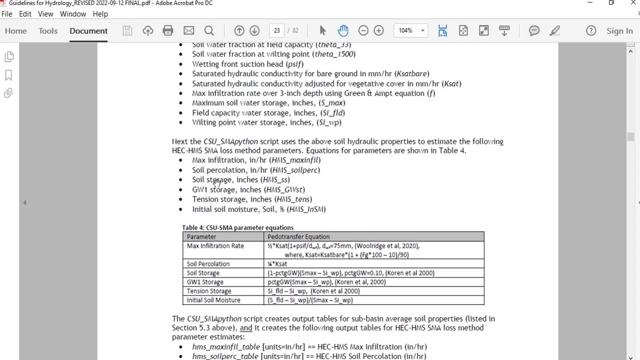 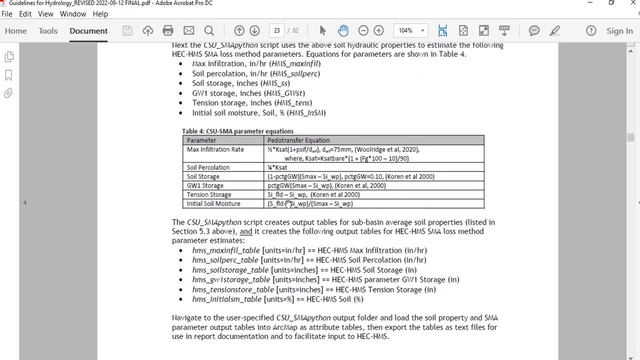 now, if you remember, let's flip back to the guidelines it's. we try to make this all pretty clear. keep track everything it's, it's generating and what it all, what it all means. so, if you remember, here we list the, the parameter estimation methods from urban master's thesis, and then the, the, the CSU estimate Python script. 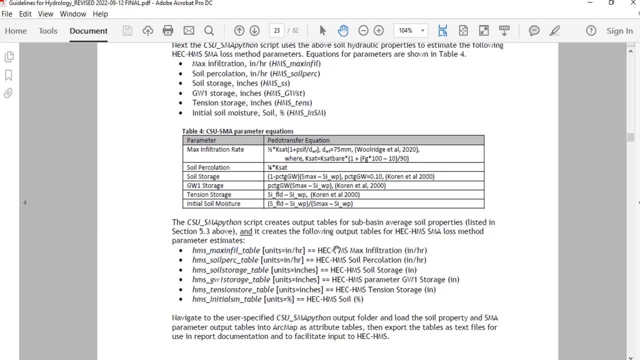 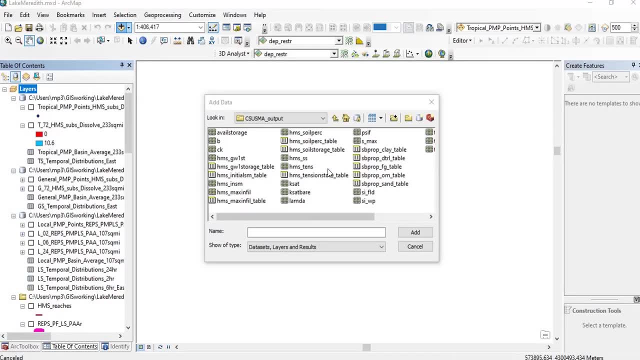 output, table name and then what the parameter, HMS parameter, that actually each one it corresponds to. okay, so if we just use these tables and go into art, the arcmap, the CSU, estimate, Python output, you will see that first of all, we have in the guidelines, we have max infiltration tables. let's just look at 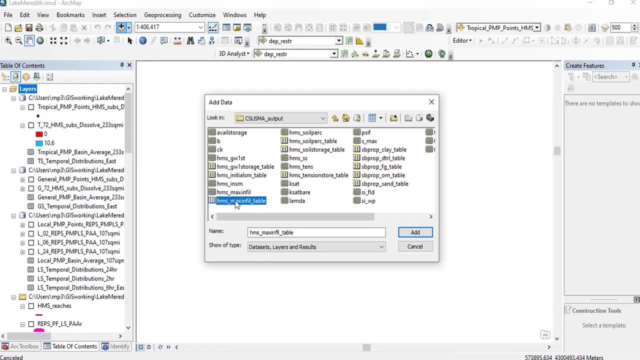 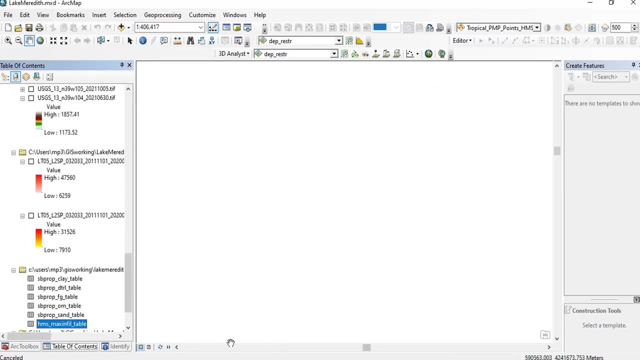 that one. there's actually what. there are six tables and we're going to bring those. we would bring those all into our mark map project, but let's just right now, let's just do one of them, the HMS max infill table, right, and that include that that contains the maximum infiltration rate parameters for each. 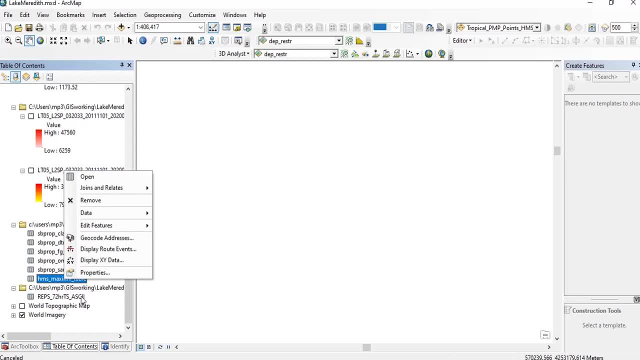 sub basin for our HECA HMS model for this basin. okay, so let's go ahead. if you remember, these come in as attribute tables. in order to export them from HM, from ArcMap, you have to open them first. if you're not super familiar with ArcMap and you remember my 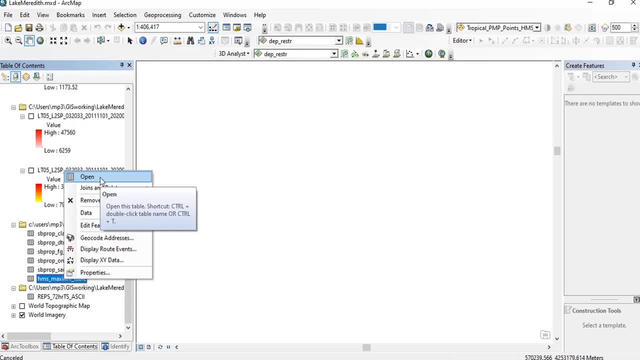 war the disclaimer we've given him all the previous tutorials. these are not meant to be ArcMap tutorials. it's just we just want people to have enough knowledge of ArcMap skills that that that's not a limiting factor in applying this in our new hydrology methods. so let's open that attribute table and 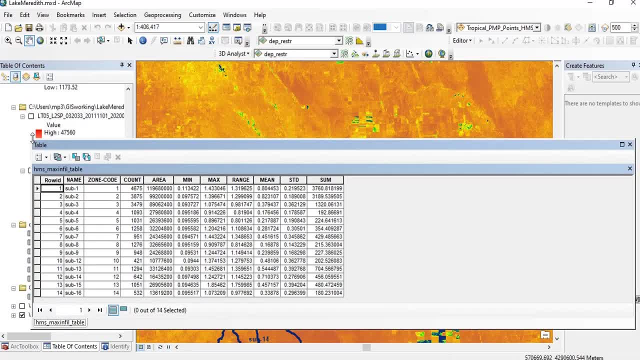 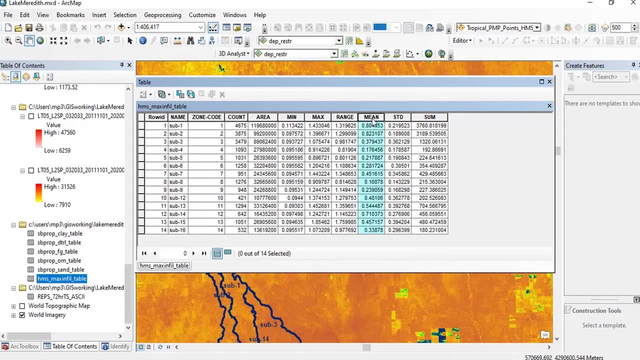 you'll see here again. this gives the the. the way the Python script is written is it gives all the zonal statistics for that parameter. but what we're, what we want to use always, is this mean column. that's our best estimate and we have those case at best estimate, a vegetative adjusted case at. I'm sorry, it's not case. 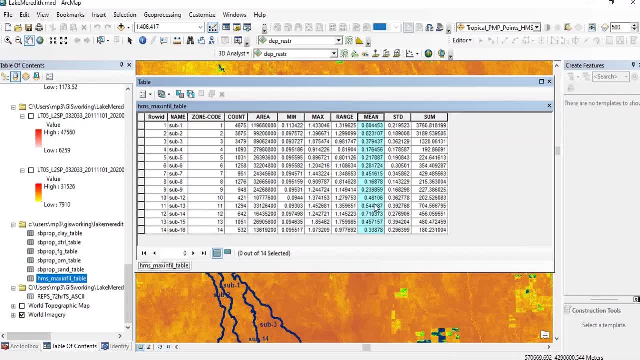 that's the max infiltration. it comes from that group and that's what we're going to use for the next column. and we're going to use is a group template in a subbasin. so we're going to walk through that model in a couple of. 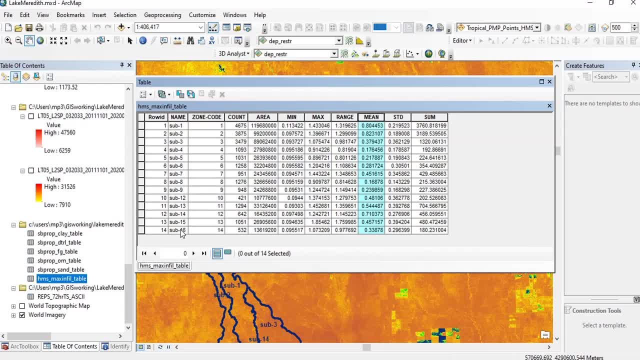 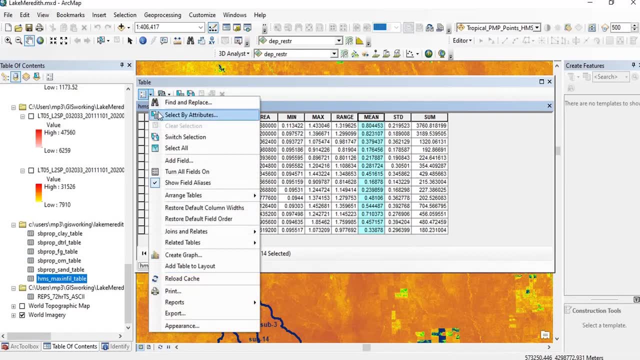 questions. yo, this kind of table we're going to. we're going to forget it because we're going to get some more data. we're going to get more data that we don't know completely. I might talk a little bit better about this table, but no problem, as long as we 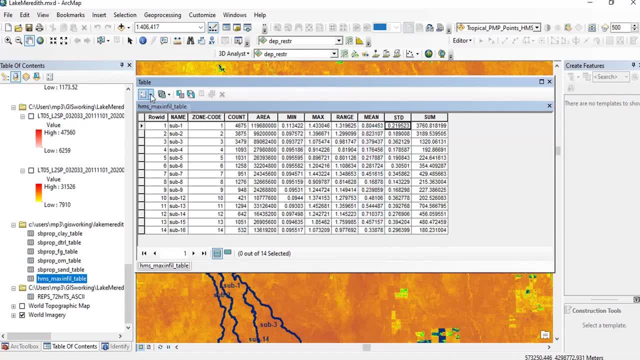 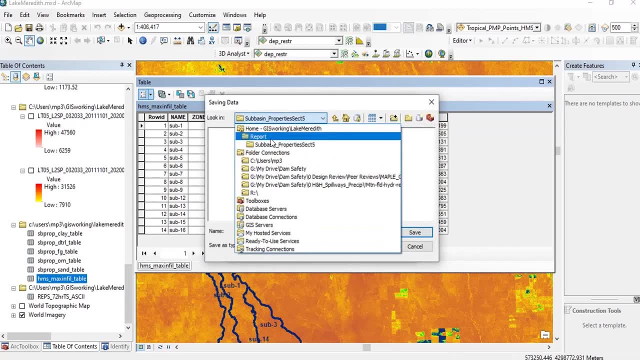 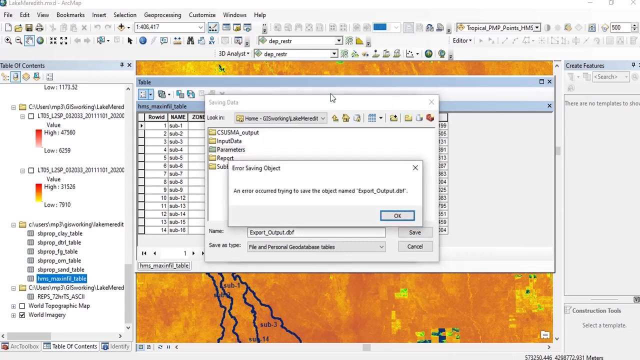 leave the table. that was a pretty good example of how we can Indiana very it to a text file. okay, so we'll just do that here and I can just put that in my project folder, as I'm going to create a folder here for parameters. I'm going to 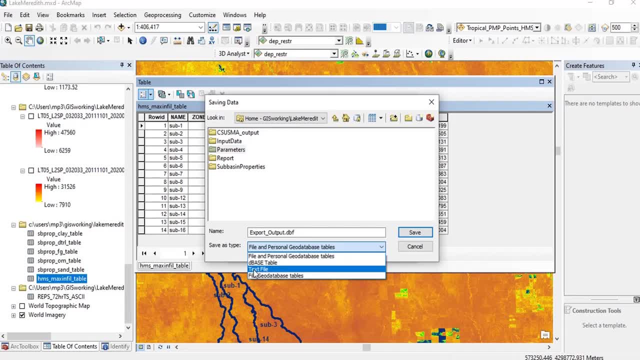 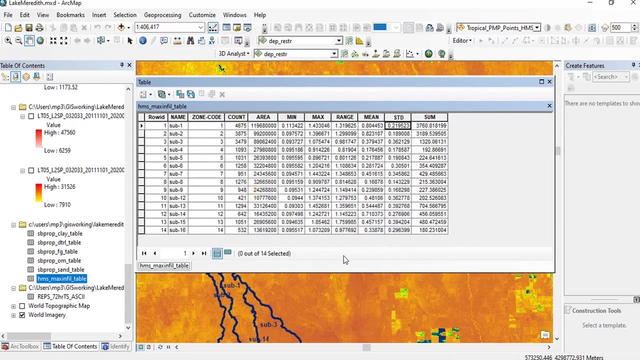 change the output file type to text file. okay, put that in parameters. and then I'm going to change this to max infill. okay, and that's going to give me this table output. okay, I don't need to add it, it's already added. but what I want to do is go show you what that looks like. so this: 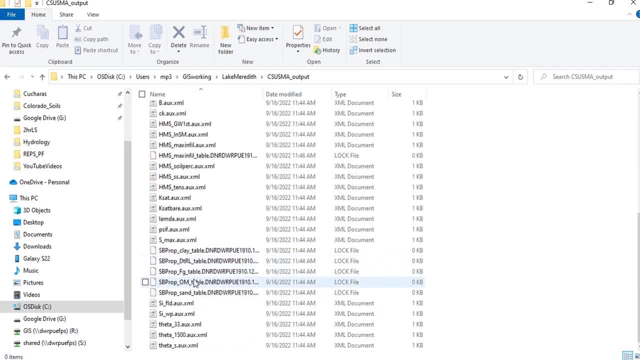 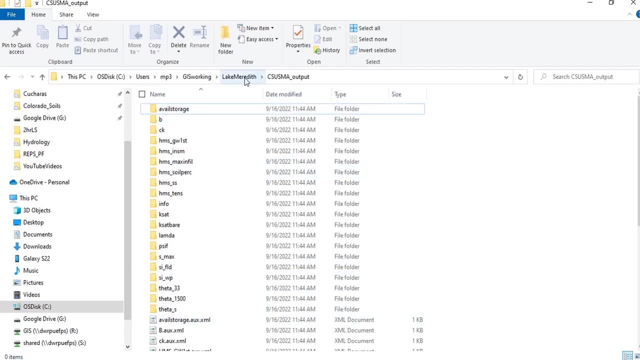 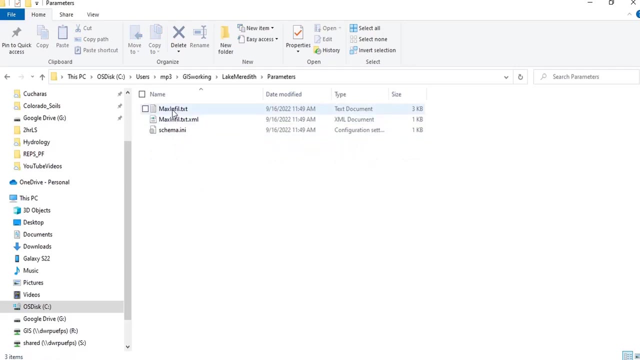 was our CSU SMA output. this is everything that all the files and folders it just created. these are generally ArcMap files, so we're going into ArcMap in adding them is attribute tables and then exporting them. so let's go up a level. look at that parameters folder that I just created and I created this text file. 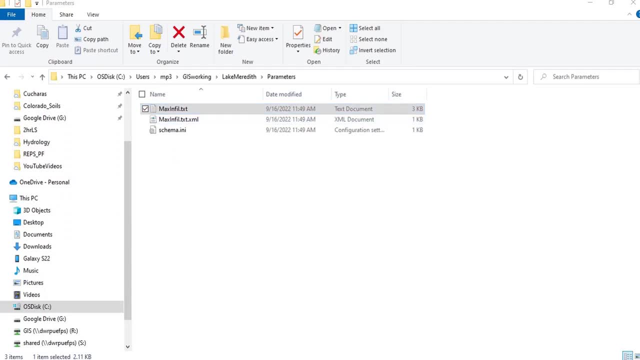 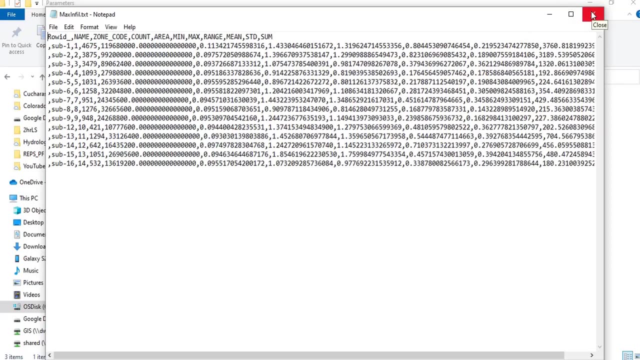 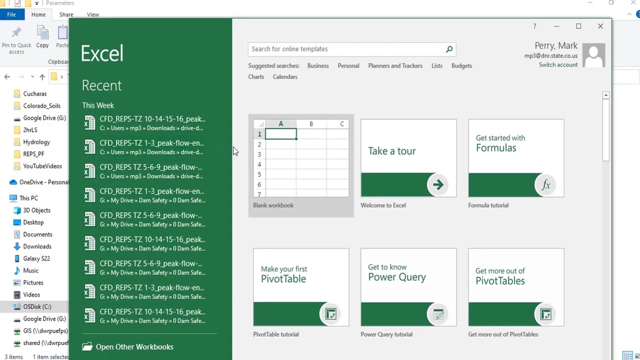 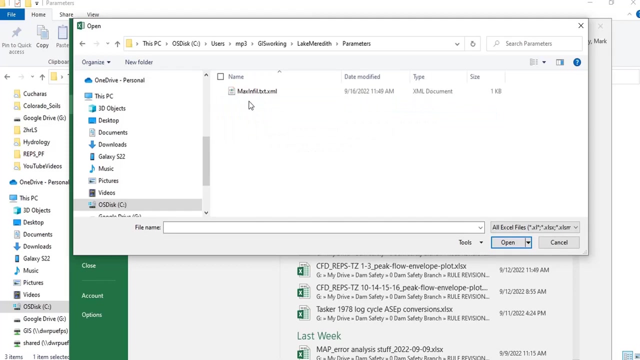 okay, so let's open that and ultimately, what I'm going to do is open that in Excel effect. I could do that now because this is pretty messy as a context: comment delimited, comment delimited text file. so let's go ahead and open Excel and simply open a new worksheet. okay, my parameters folder, and then I have to select all file types where. 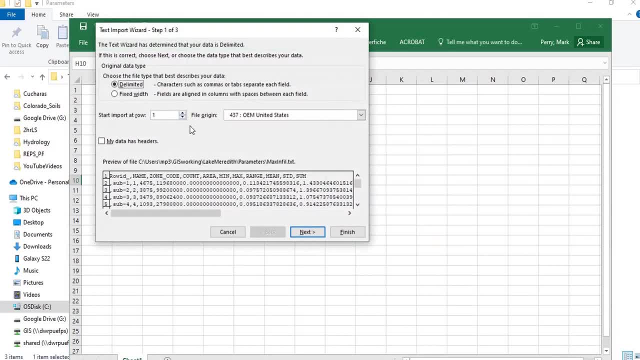 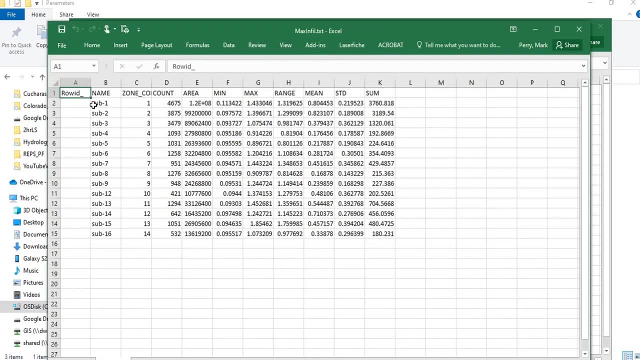 you see a text file and just bring in that common delimited text file, come on this and we get a nice, pretty looking table here: my sub basins and then our main parameter estimate fret. best parameter estimates for max infiltration from. our main parameter estimate for max infiltration from: 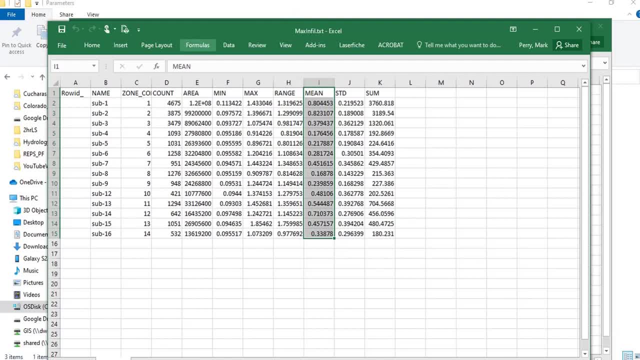 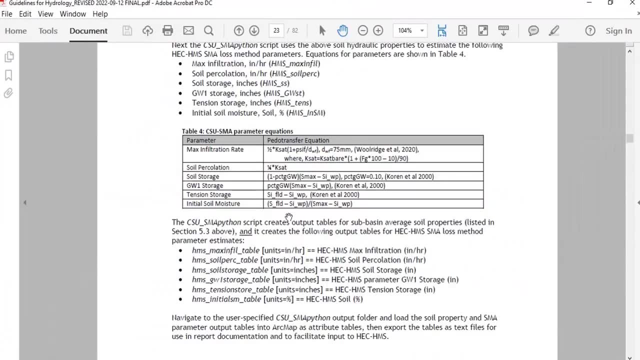 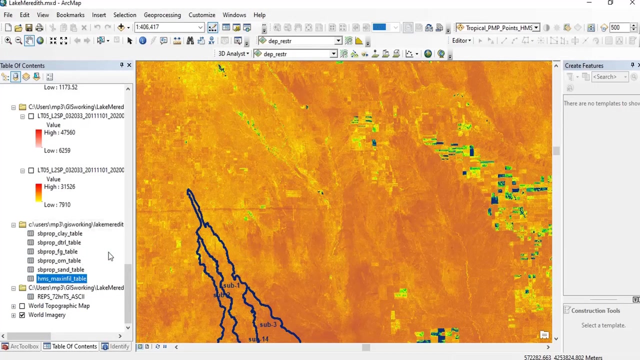 that csu sma python maximum fill table. okay, okay. so next all we do is repeat that for the hms soil park table. so storage table, groundwater, one storage table, tension storage table, an initial storage table, and we can even do that pretty easily. so go to the csu sma python. 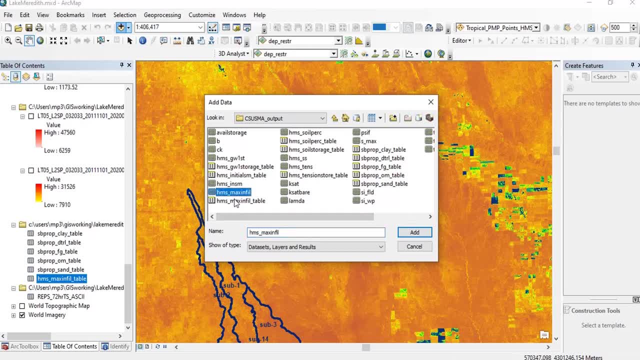 output folder we created and we're just grabbing. we already grabbed the infiltration, max infiltration table. yeah, grab the tables, not the raster. those are the raster images of the actual uh calculations, but we just want the table output. uh, then, so perk table would be next. so a storage table. we have a tension storage table, groundwater um one table storage table. 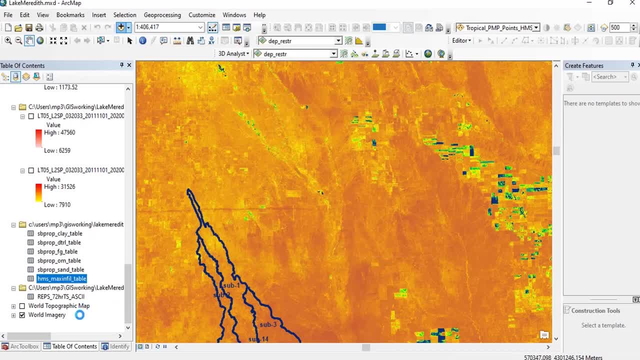 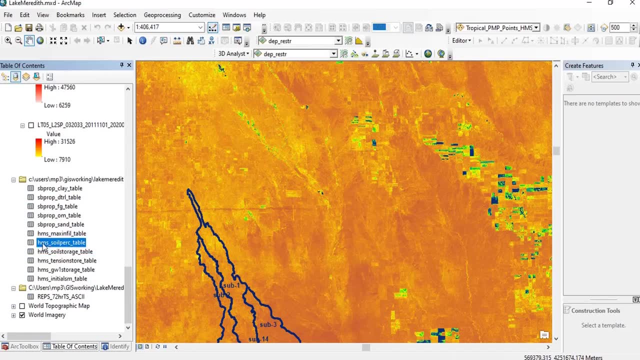 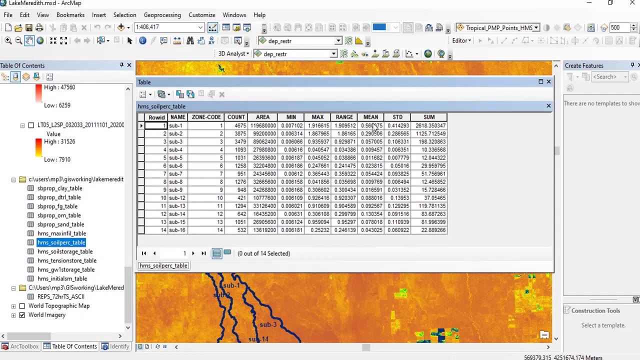 and an initial sm table. so that's it. just add all those and they're going to come right into, they are going to come right into arc map and we can do the same thing, same process. just open each of those. we'll see our mean. we'll see all our zonal statistics, our mean. 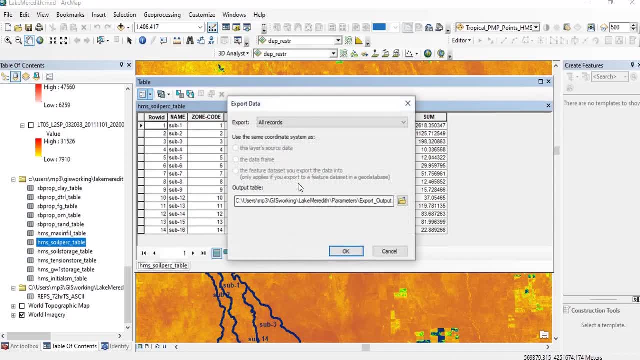 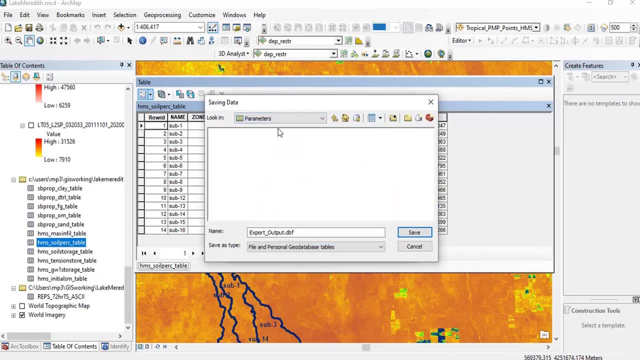 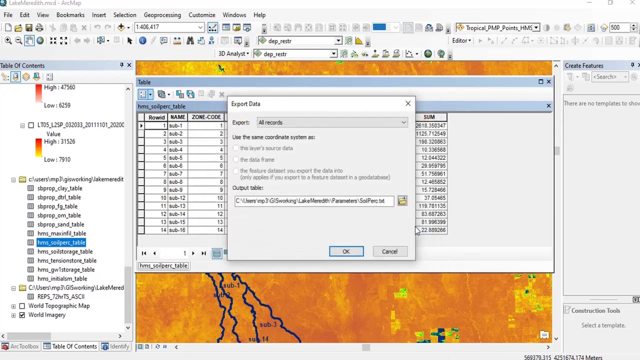 best parameter estimates and we'll export each one of those as again to our uh project folder on our on my c drives parameters um, a folder that i created and it's a text file, and so this one is just the uh soil perk parameter. that's all i need there, and so on. continue to do. 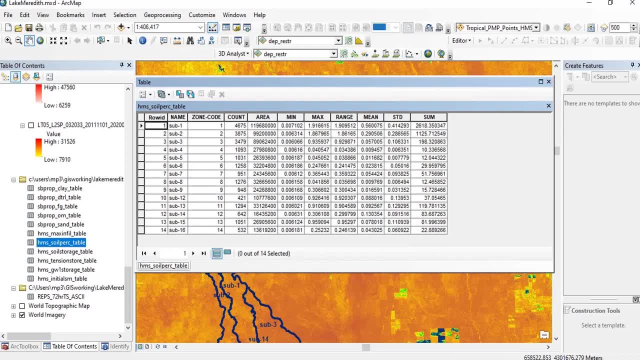 that for all of those maximum fill parameter, soil park parameter, soil storage parameter, groundwater, one storage parameter, tension storage parameter and initial soil moisture parameter. okay, so that's it. that's all. we need um from the csu python script to to set the parameters in the um. 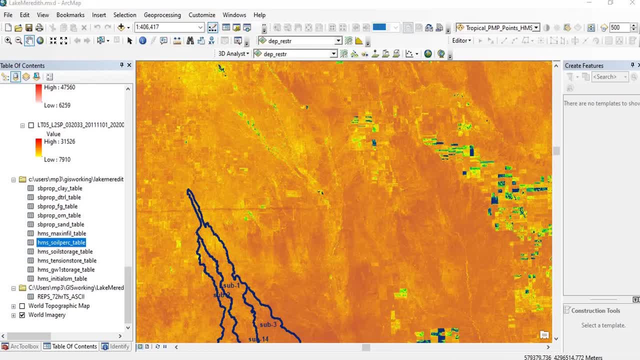 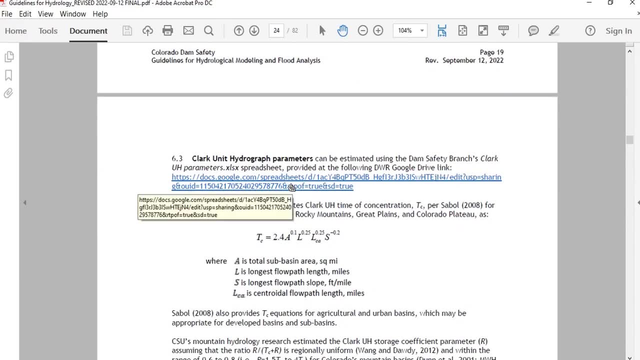 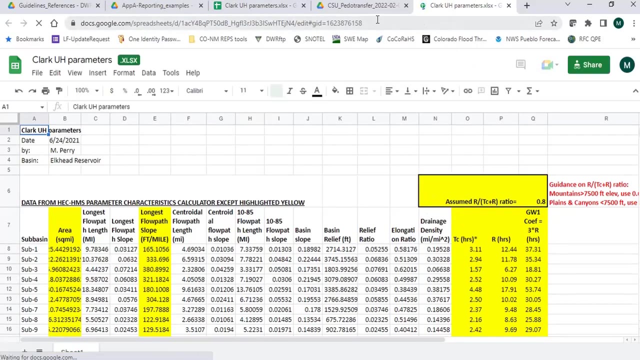 hms sma loss method. okay, so now let's jump. should be able to wrap this up now. let's jump back to um quickly, to the clark unit hydrograph spreadsheet. i talked about this briefly already. um, there's a. we have a sample spreadsheet on the in the linked in the guidelines. you can download that again. download. 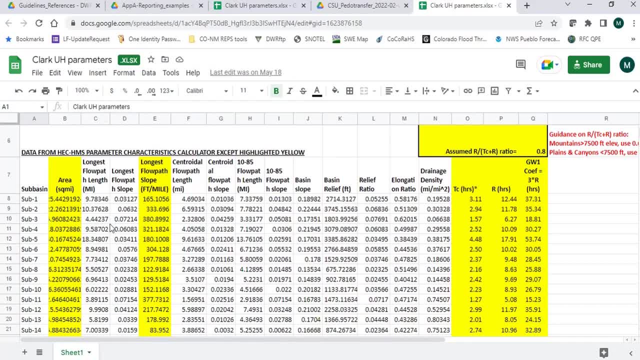 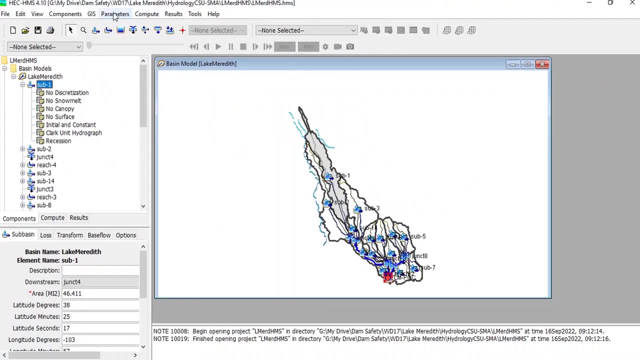 that to an excel file. but here i'll just go over it quickly. all you're going to do is um, you're just going to copy and paste uh, the. the properties from that came from the uh, hms. uh, let me go to that real quick. in hms, we um, went to the parameters menu and characteristics and opened this sub basin. 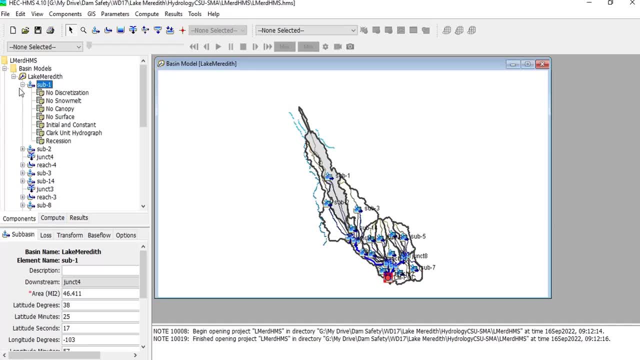 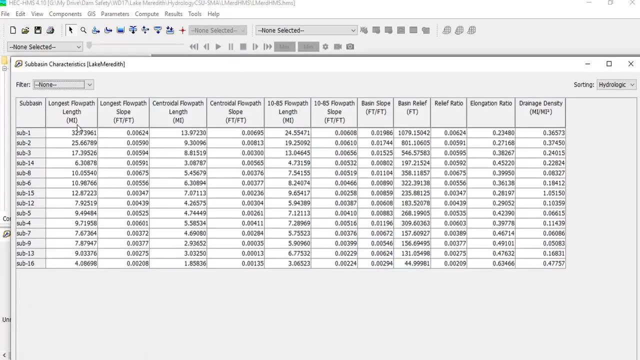 um menu and here i have. so i have sub basin one uh selected, so we don't want to do that and unselect the sub basins, parameters, characteristics, sub basin menu. and then we had all these properties. i just copied those out and, if you recall, we had then a sub basins uh, properties uh spreadsheet. we had a tool for that that we gave. 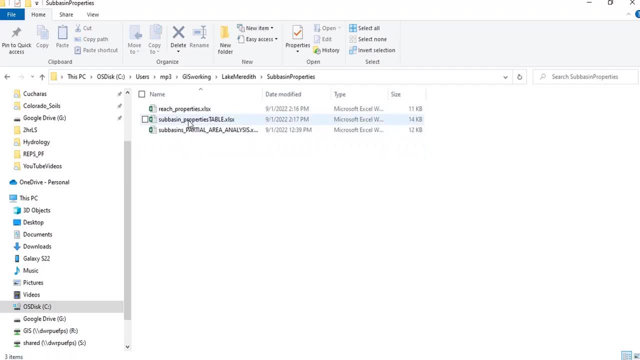 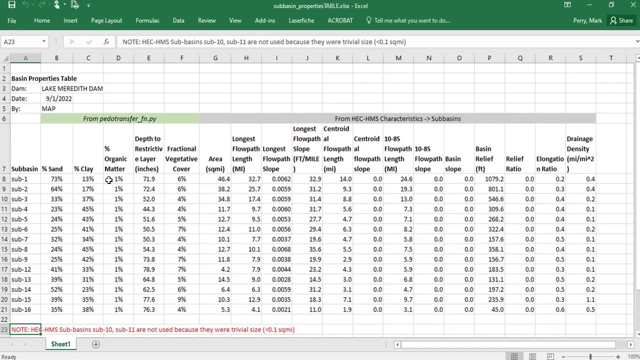 you. okay, so that was under sub basin properties and if we open that i had um all those proper properties in it plus the soil properties, the soil sub basin average soil properties that came from the csu sma python script. okay, so these things you can just be these properties from. 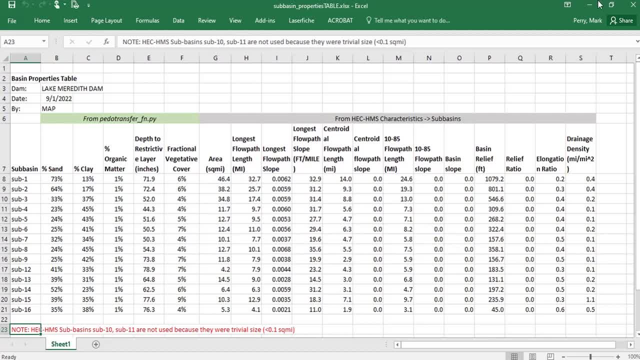 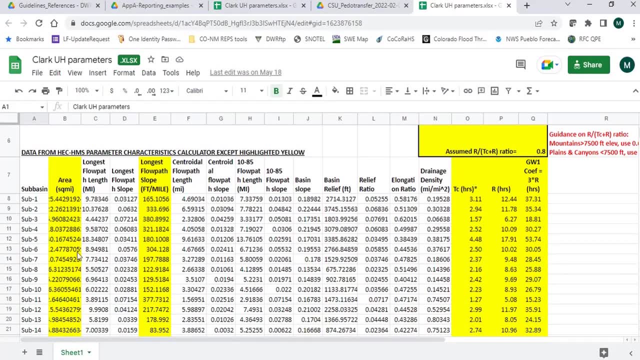 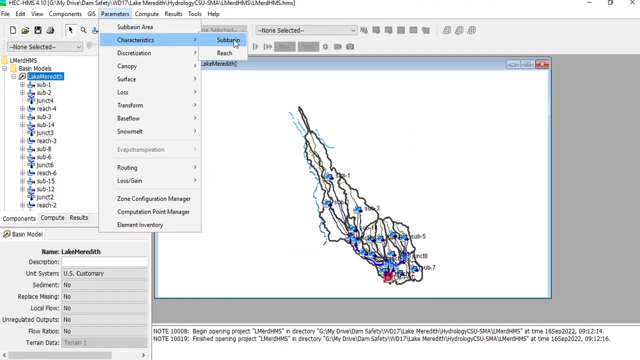 head catch ms characteristics sub basins can just be copied over directly into this example: um sample clark unit hydrograph parameters spreadsheet. okay, now the yellow, yellow um this: this has to come from the sub basin areas characteristics sub basin, or sorry, sub basin areas. um table that hms creates um. but i believe then 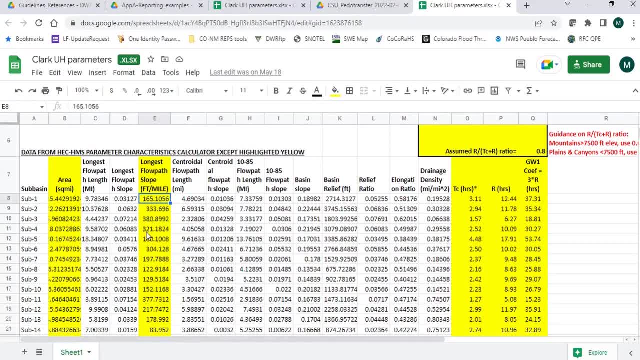 these, these yellow columns, are calculated, and again, we need to download this to xls to see this correctly: the feet per mile longest flow plus slope, i believe, is calculated. and then, um, these tc and r, yes, are- are calculated here, so you can see that the tc and r are calculated here, so you can. 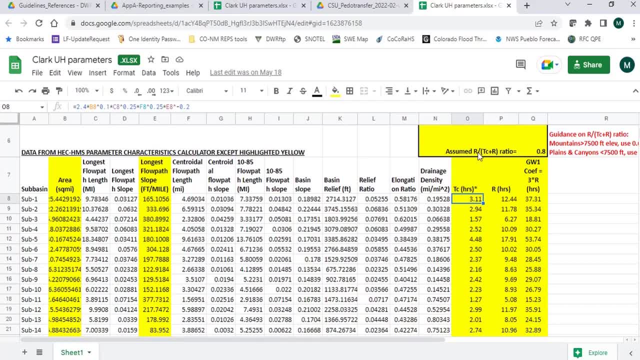 you can use this spreadsheet. you can enter, if you're using this uniform r, tc plus r ratio method that we talked about, you can just enter the ratio you want to use as your initial best estimate for clark new hydrograph parameters, and these are by sub basin um. it will, the spreadsheet will calculate. 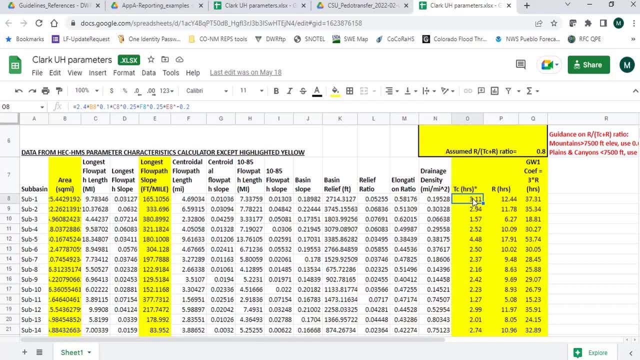 tc using our 2008 guidelines, sable 2008, our old hydrology guidelines. the tc equation from that and then it will calculate r based on the ratio that you as user give, given the spreadsheet, and then it also kept. we also calculated groundwater. one coefficient, which i'll show you, is per um. 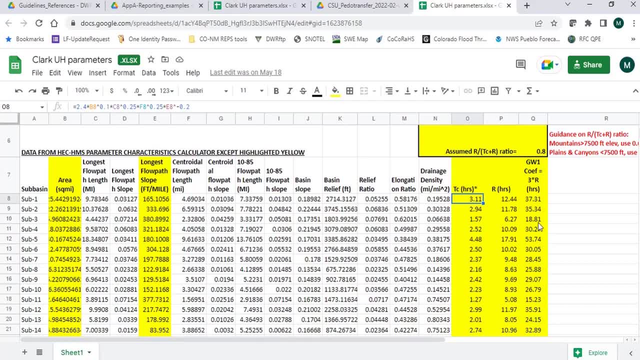 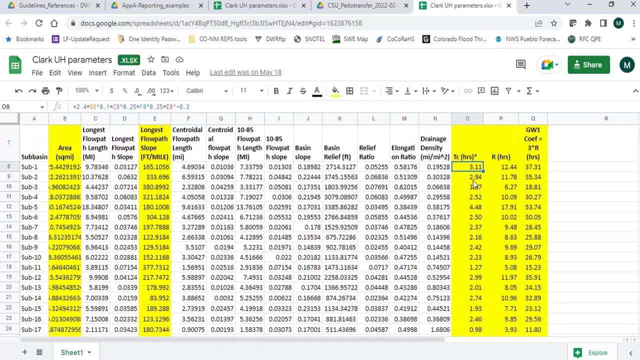 irvin, uh ben irvin's master's thesis: parameter estimation: um guidelines. it's that. that is that timeline for uh. groundwater um coefficient is three times the surface water are okay, so you can complete that spreadsheet and then you will have all of the um. clark unit hydrograph. 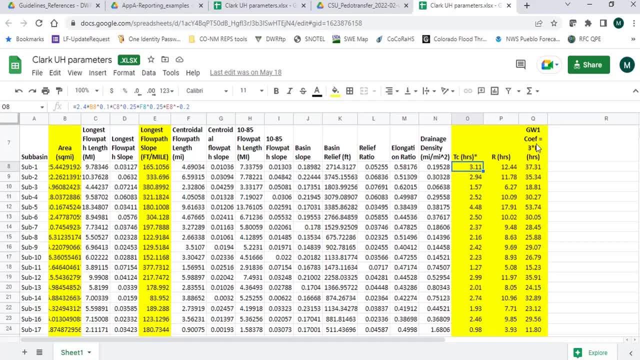 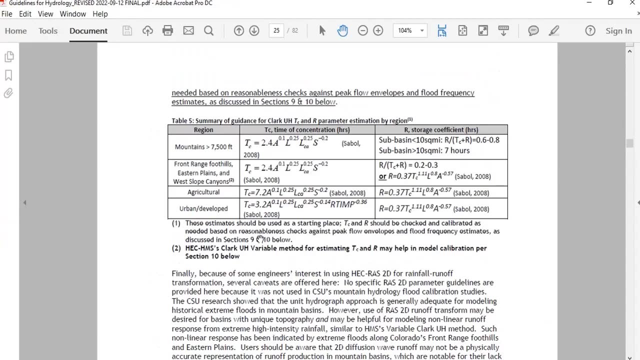 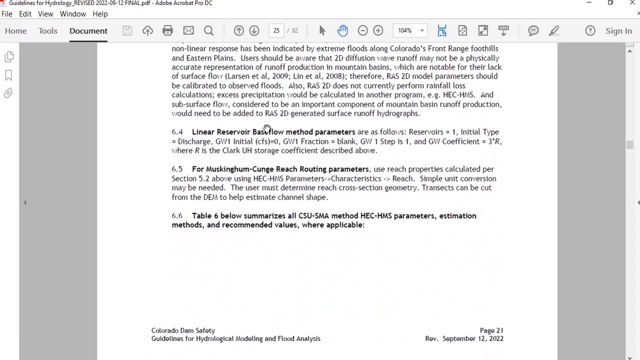 and groundwater. one, uh, our coefficient parameters, estimated for each sub basin. all right, and then? um then, what we'll do, uh, next, by the guidelines is, let me just go over the over the. there's a few miscellaneous parameters in the in the method here for our sub basin setups in heck hms linear. 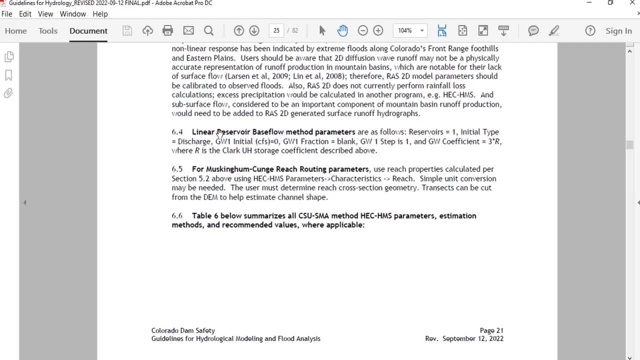 reservoir. so there's a few parameters in that and the parameters are just given here. they're very simple. reservoir is one initial type, discharge, etc. here's that. groundwater coefficient. three are um that come. that actually comes up twice and i'll show you that for muskum kange, then just the. reach routing um parameters and those come from the groundwater. one coefficient, and that comes up once and i'll show you that- for musky delcunge, then just the reach routing um parameters, and those come from you know, give us three years of余는 water, two centimeters and dellebuhm municipalities, so you can track that's kum crashes in the evaporative�. 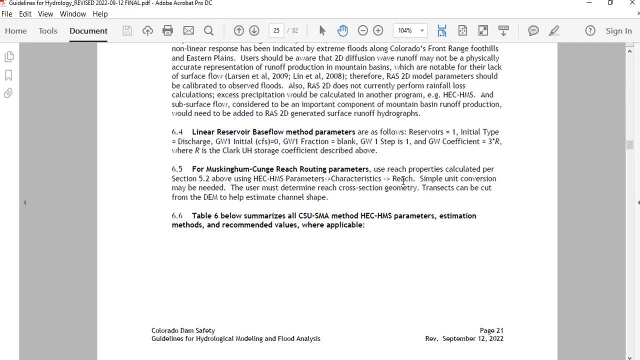 �at mornings that this energy vorne altitude and this requirement for Courshin green and the otherار UV 2D drillthis energy of American". regarding the operation cost to choose from a muscle to Hawaii tokens the from that reach routing table properties table we created in section um in the tutorial in section 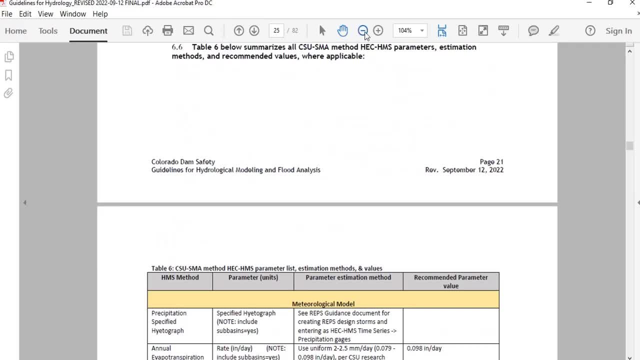 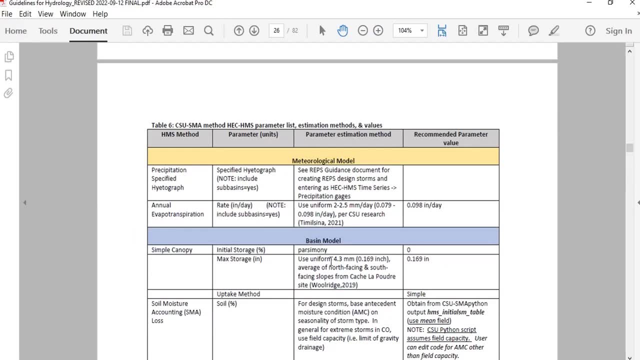 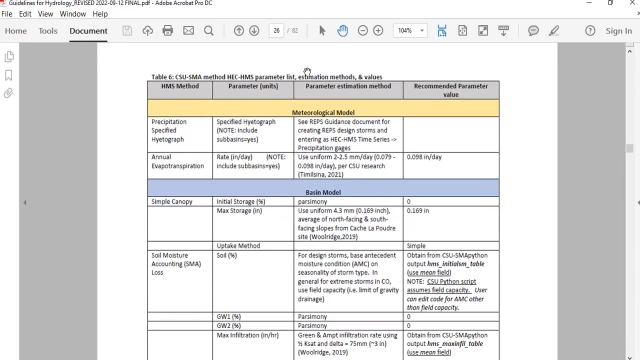 five of the guidelines. okay. table six is: we've heard feedback that people like table six. i mean it's, it's. i think it's very helpful. it's just a summary of all the parameters that are going to go into the heck hms model using this csu sma method. okay, so table six is kind of a master table um. 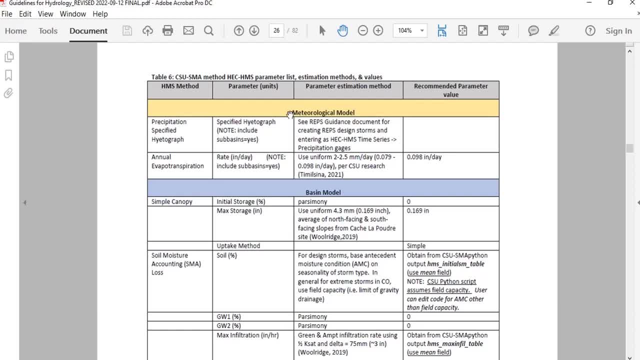 met heck hms method. it has the different um elements, model elements in it. it gives you the parameter, the parameter estimation method, and then, in some cases, the specific value or how to get the value. okay, so the met model um specified hiatus graphs- those come from reps- temporal um temporal. 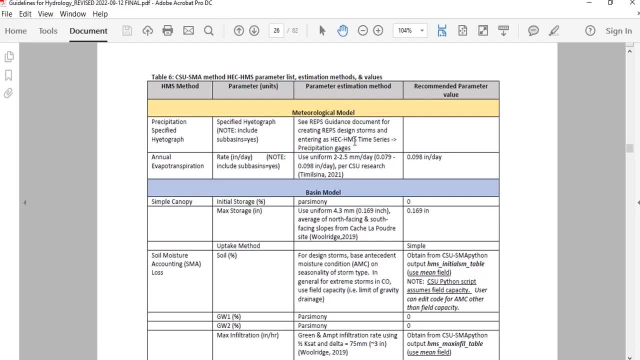 distributions and you create precip gauges in in uh tech hms's time series precip gauges. okay, evap, evap in the each met model will have evap um. the parameters are the rate and include sub basins where the guidelines, the these guidelines, the csu research, um study recommended um 0.098 inches. 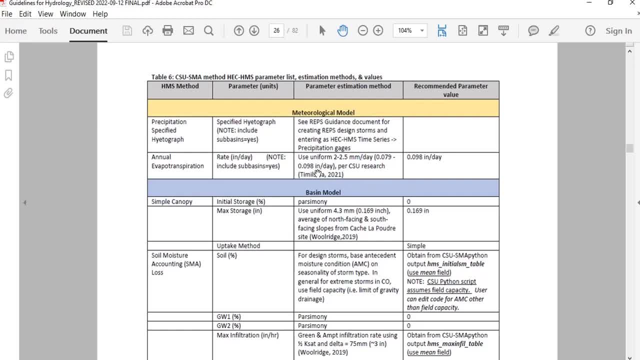 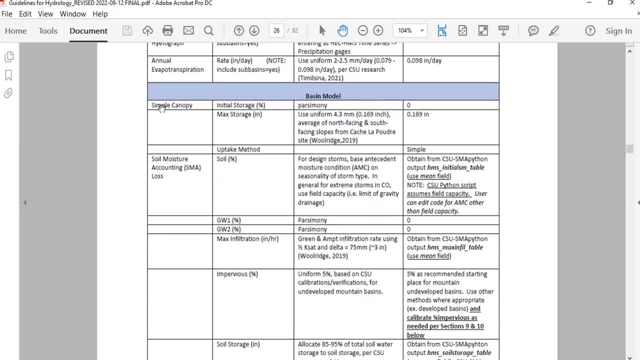 per day, and that came from um previous research, just from literature that they had uh researched. all right, then your basin model, the simple canopy method. uh, initial storage is zero and where we have parcimony. that's just basically a fancy way of saying, just to keep it simple, that's what csu did in their research. 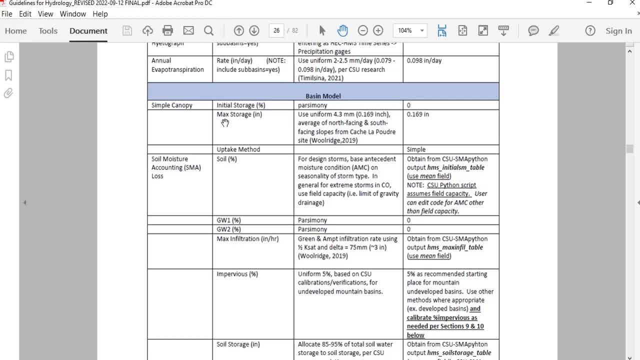 study. so that's what the guideline is here. maximum storage is 0.169, and that was based on a field uh research site that they have csu operates in the cash laputa basin, um, they, the. so then the soil model is based on a field uh research site, and that was based on a field uh research site that they have csu operates in the catch laputer basin, uh, the, the. so then the soil models would be single encICO and a single MiC s and csu minder basins, um. so that's good, um, as you can see that there's, i think, this shining area there's. 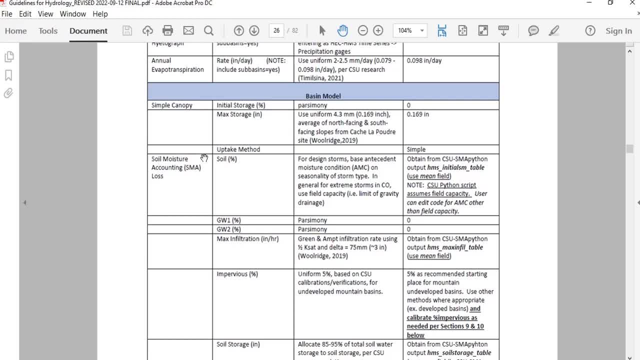 moisture accounting. Oh, the uptake method under simple canopy is simple. The soil moisture accounting loss method now. So again, just for I don't know. I'm not going to go through all of these in this table. You can read the table for yourself but say, for example, this: soil percent. 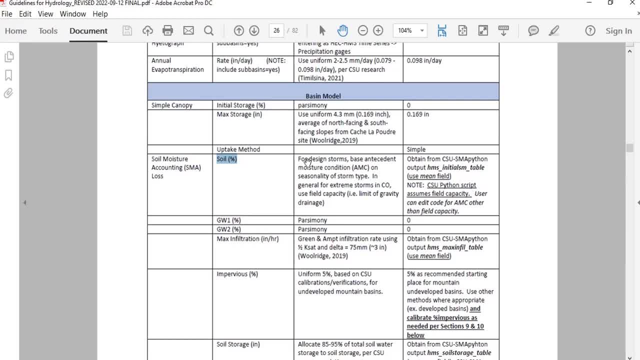 is that antecedent moisture condition, that initial soil value, So soil water value. And I told you the way this script is currently written. it is set for fuel capacity. You're welcome to change that. You can change that if you want to, but that's what we found kind of. 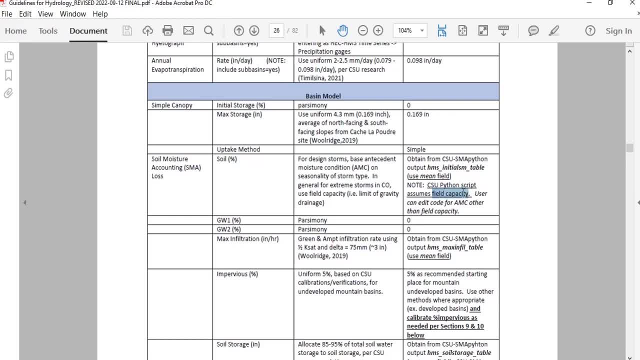 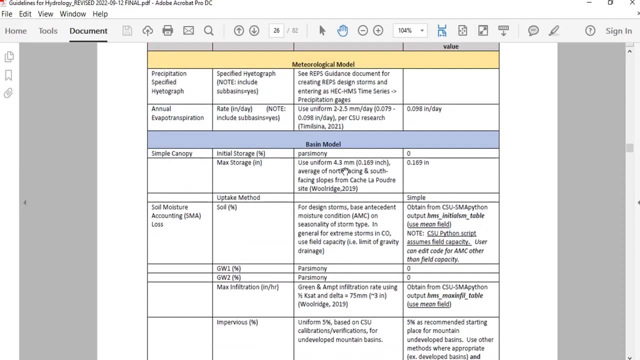 for most historic floods in Colorado. the soils drain quickly and fuel capacity is a reasonable number, Say, as opposed to assuming necessarily, like a worst case, that the antecedent moisture condition is saturated. but you could do that if you wanted to, So in under the 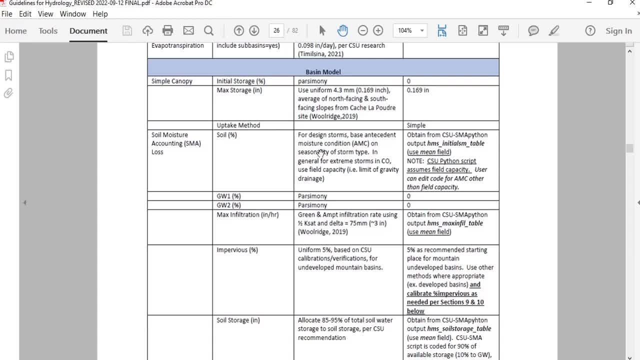 um parameter estimation method. uh, we use field capacity based on the CSU research um, that's gravity limit of gravity drainage. and where to get that? on this last column obtained from the CSU SMA Python output, in the HMS initial SM table use the mean field. Okay, Um, that assumes field. 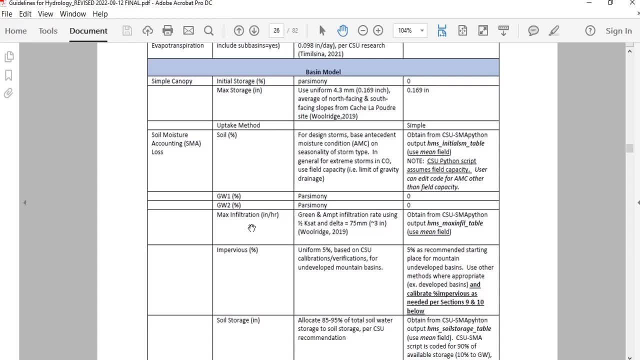 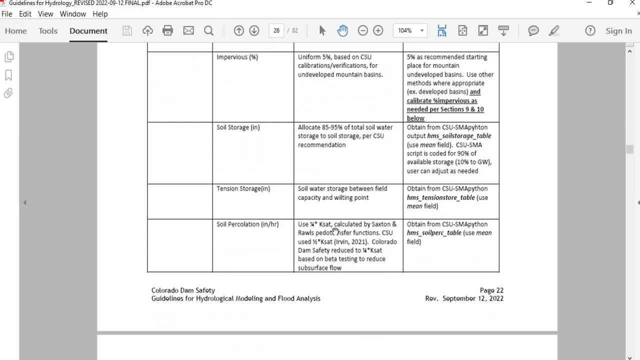 capacity. You can edit that if you want to. So this, um, this is this. table is going to go down through each of these parameters. Tell you where, where you get it, what the recommended value or and or what the recommended. 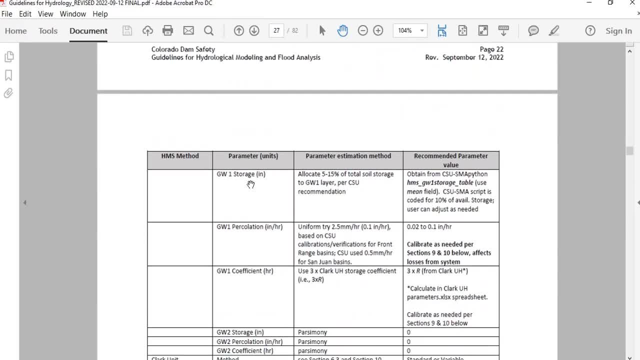 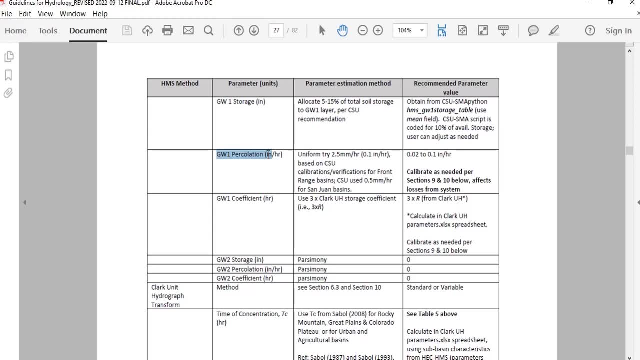 value would be um through the soil storage, tension storage, soil percolation, groundwater: one storage groundwater, one percolation. uh tells you. you know, some of these don't come from there. They don't need to be calculated by the CSU SMA Python script, They're just. 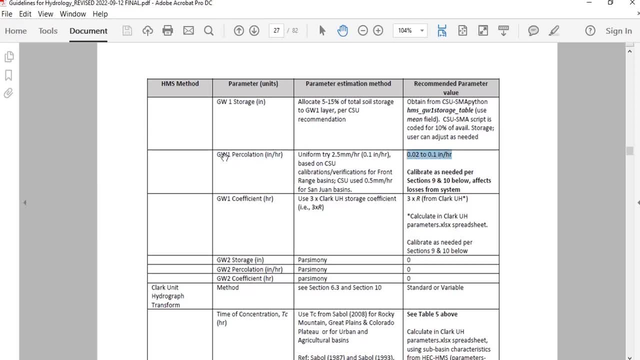 specific values that are recommended from the research study. So, for example, groundwater one percolation, if you recall, that's that rate that water can leak. Leak out of the um shallow groundwater layer and into the deep groundwater layer. loss from the. 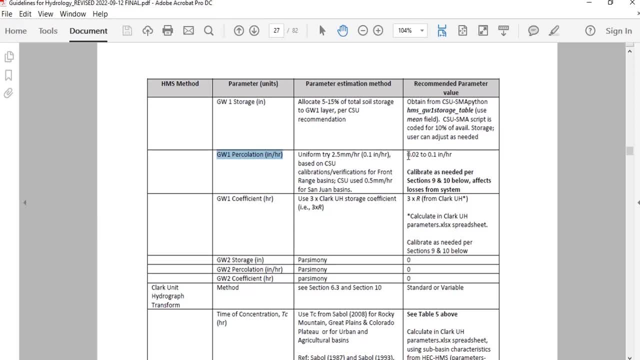 system And what they found, CSU found in their phase one of phase two studies, is about 0.02 to 0.1 inches per hour And that goes loss of the system. Okay, Groundwater coefficient: That's that number. that's calculated from the that just showed you in the Clark unit hydrograph three times. 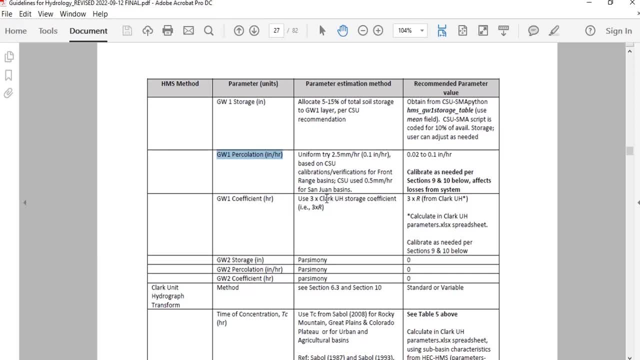 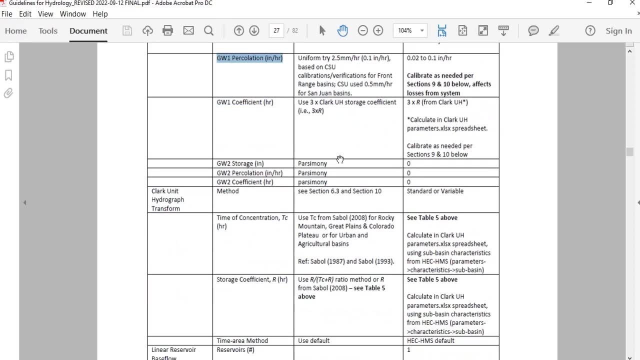 R. whatever your R method you use for your R to get um for the Clark unit hydrograph, a parameter three times R is what's recommended for the groundwater: one coefficient groundwater. two: zero percolate groundwater to percolation zero and groundwater two coefficient zero. Okay, 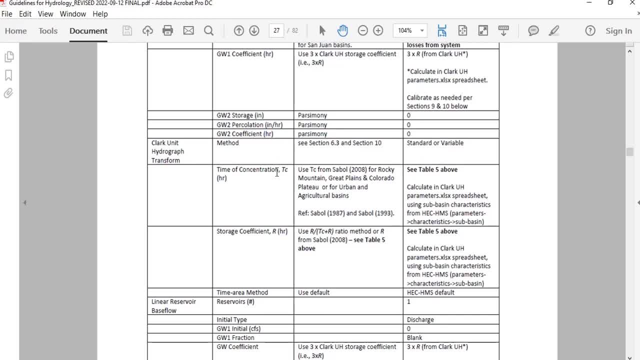 And then Clark unit hydrograph. we have those TC, time of concentration, um methods, standard or variable. I talked a little bit about that and we'll talk more about it later. but either the standard, constant TC and R values or the variable and nonlinear response to kind of concentration. 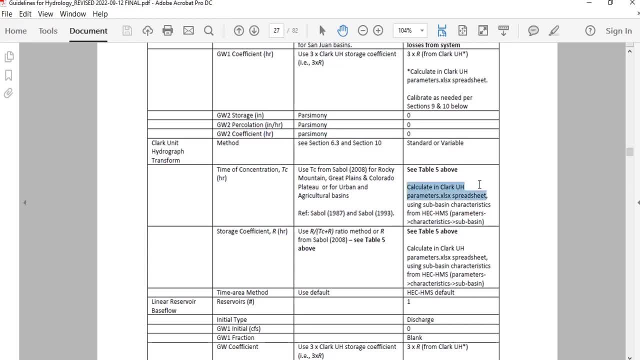 We talked about that thoroughly, Table five- and you're using this Clark unit hydrograph spreadsheet to calculate those that storage coefficient, hill slope storage- the methods for that, again, see table five- and you're using the spreadsheet, the sample spreadsheet, to calculate those. 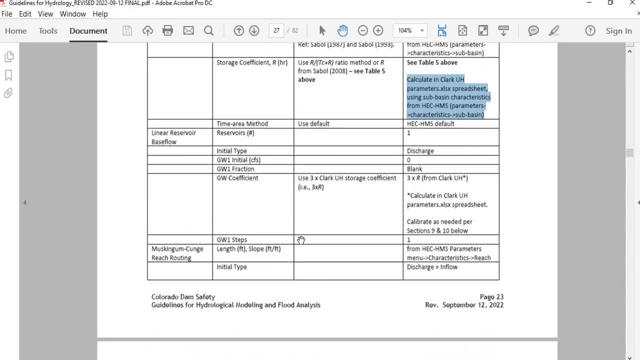 this time area method, just the default method. Okay, Then the linear base flow in HMS, um, that's, um, uh, giving you this table, gives you those summarizers, those parameters. They were written in the table five and you're using this Clark unit hydrograph spreadsheet to calculate those. 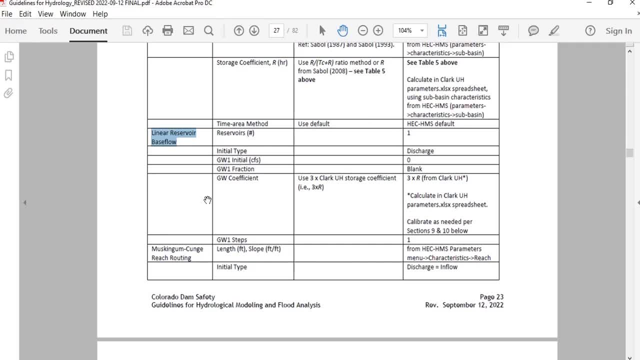 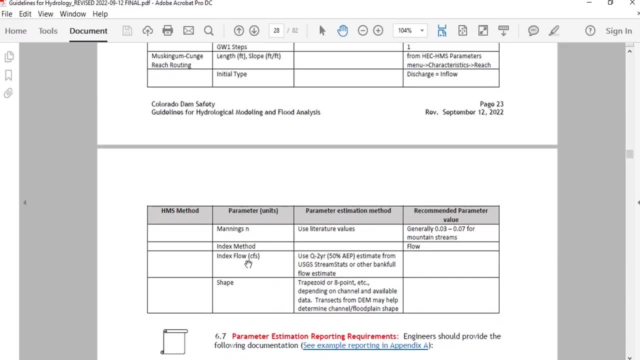 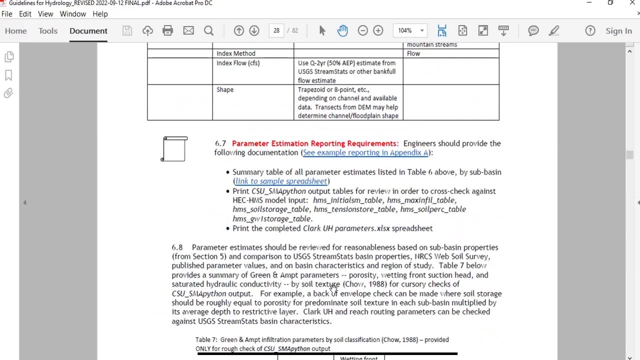 Then the text above I just showed you and then this table just summarizes the parameters you'll use for that element and the parameters and then the parameters you use there: um in the, um in your reach, routing, um method in in HEC, HMS. Okay, So now uh, the, if you recall, then we go. 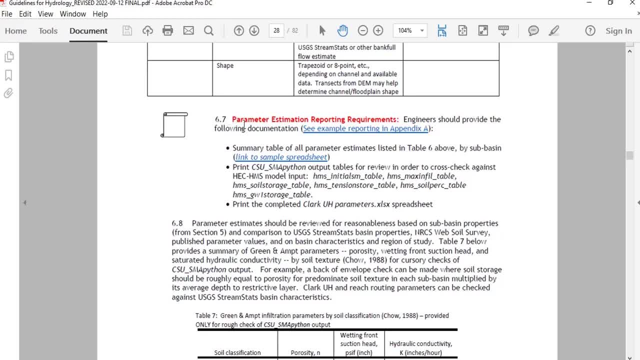 to um section six, seven of the guidelines. in this the red headings are reporting requirements. as we work through the guidelines And this little paper scroll icon, um, you can see example reporting in appendix A, the electronic appendix of the guidelines on a Google drive And then there's a link here. We want to see a summary. 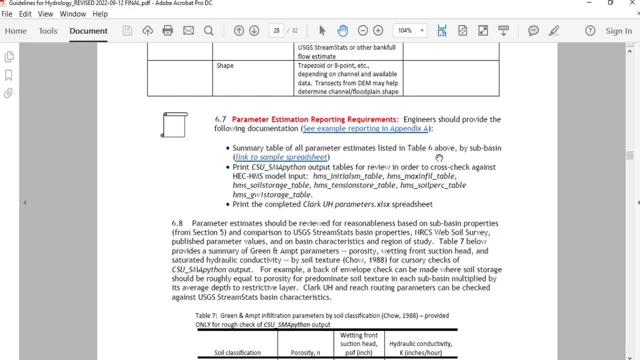 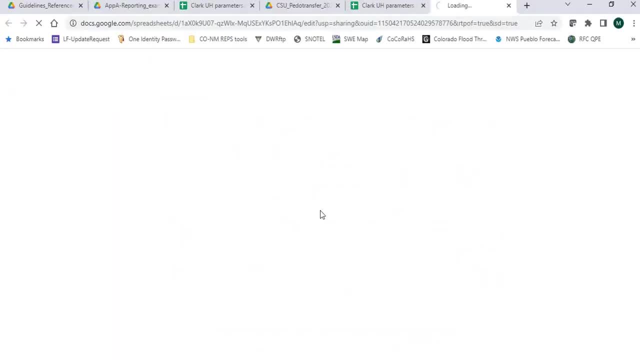 like to after table six here of all your parameter estimates for your model, And so there's a sample spreadsheet that take this table six spreadsheet and you can go to that, And what we want to see is that we want to see that completely filled in. 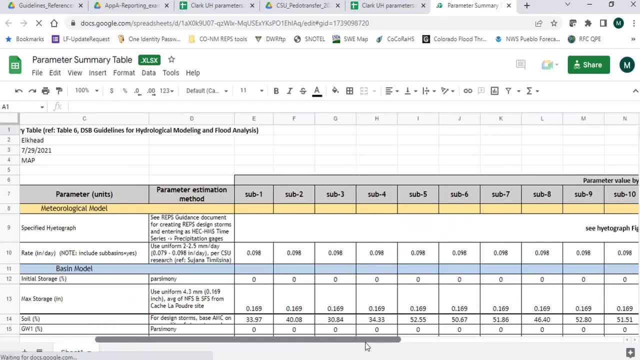 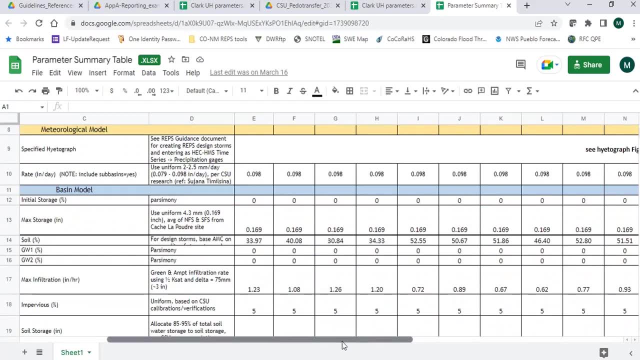 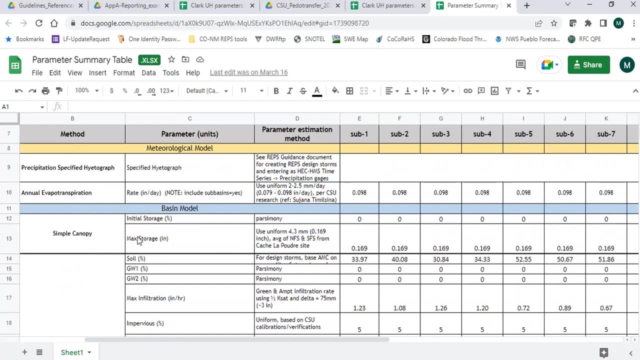 Um for your um for your study, for your basin, and then uh included in in your report so that you go through and fill this in: um for every single, um, HMS method, um element and parameter set. And what. 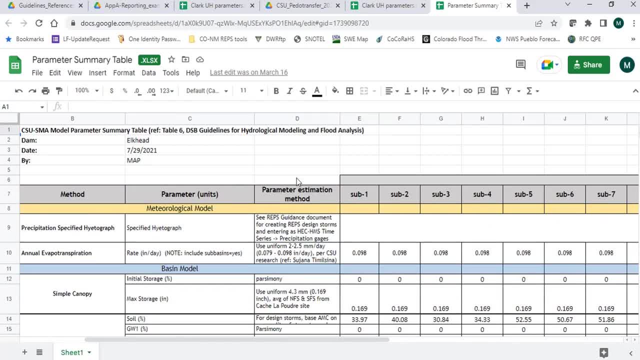 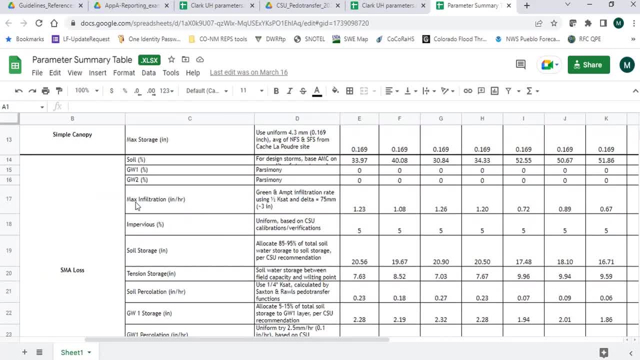 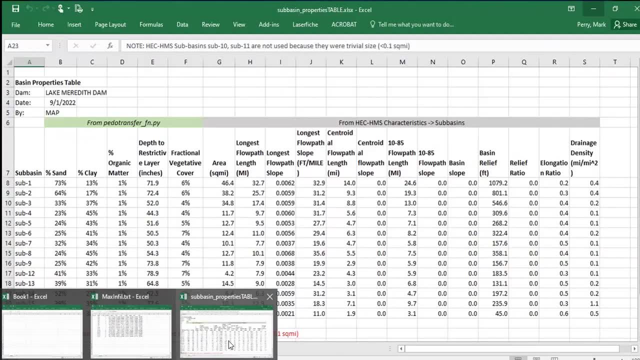 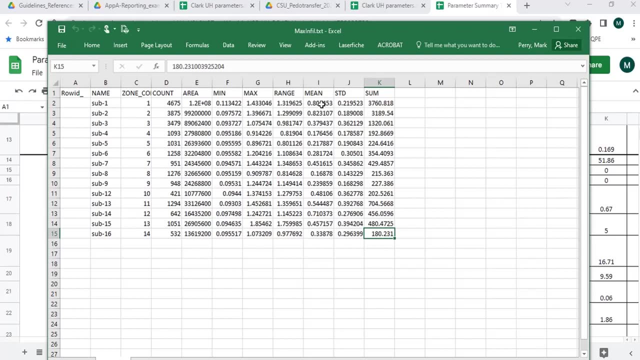 it's the easiest thing to do is just to open, say, your CSUSMA Python output text files. So we had that as a um, so we had that as a a table. here We opened the text, uh, comma-delimited text file And you can simply um copy those and from Excel transpose. 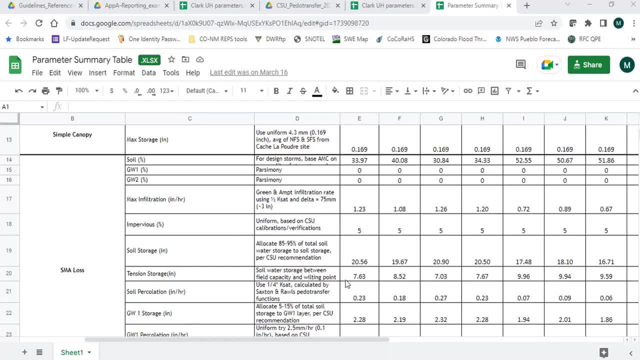 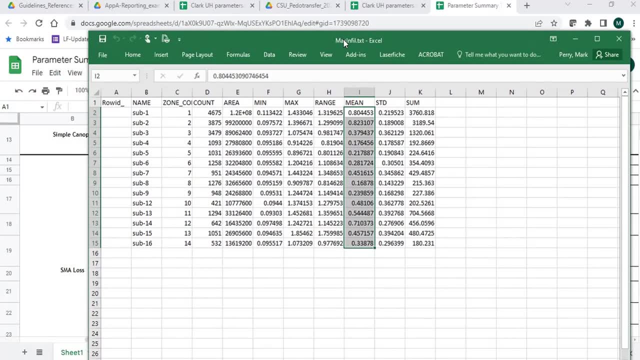 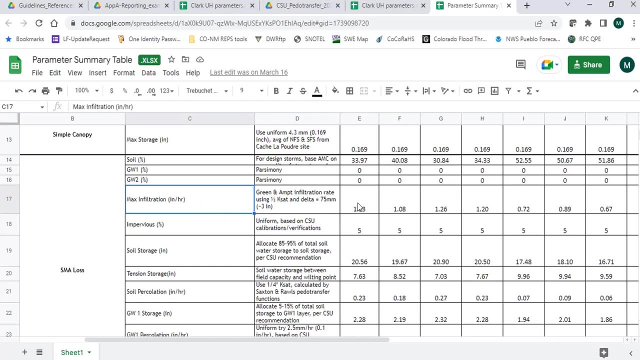 them and paste. paste, transpose those into uh the columns here for each uh column row. So this was max. this was the max infill parameter output best estimates from CSUSMA Python script. And so we just go to this max infill row and just paste, transpose those here. 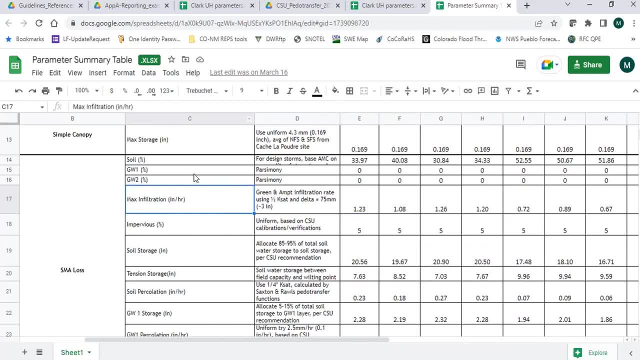 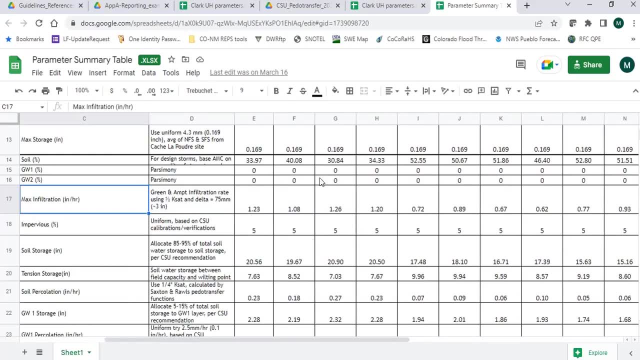 So paste. well, again, I'm in Google Sheets, but if, when I download this into Excel, I can paste and transpose those and just copy them, It will copy them across by subbasin and then that row is filled out And what ends up happening is this table. you can print this out or just have it on. 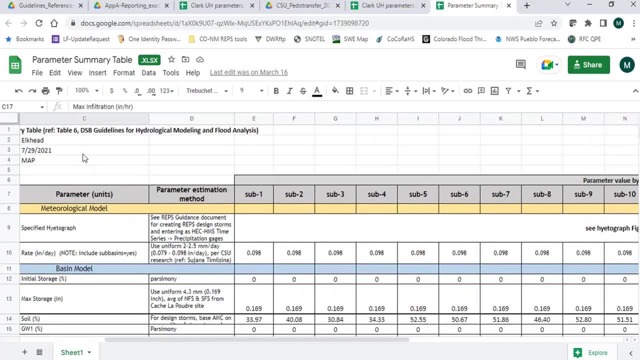 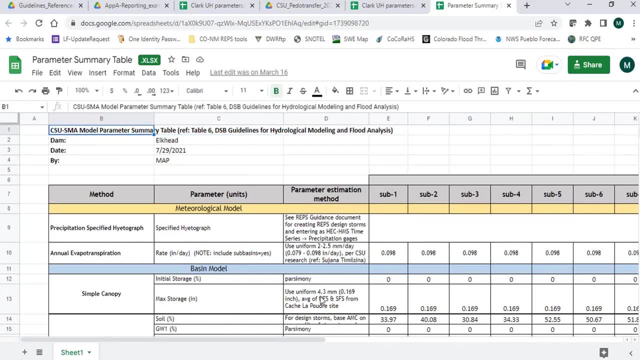 a second screen And this table six ends up being pretty much the guide that you follow to set up your entire HEC-HMS model- all the parameter estimates, So it makes having it all in one easy reference place here seems to make the model setup pretty easy. 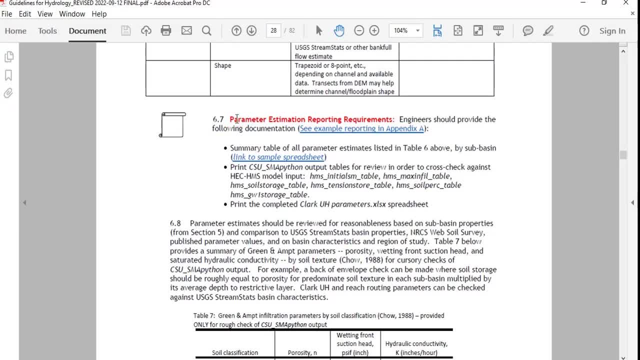 Okay, So other reporting requirements we want to see again, just like we did in section five with the properties, we want to see the output tables, the actual output tables that print out of the text files from the CSUSMA Python output tables, just to see that the you know exactly what. 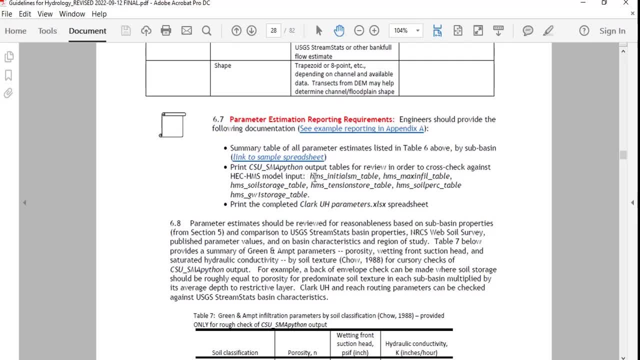 that the parameter best estimates. that mean column were copied over correctly and entered correctly into the HEC-HMS model, So all right. So that's that initial SM maximum fill table. soil storage table, tension storage table, soil PERC table and groundwater: one storage table. 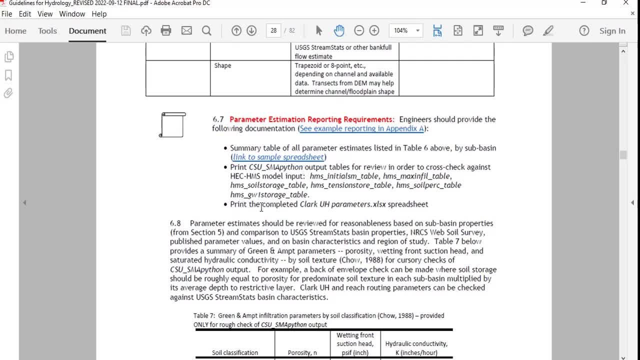 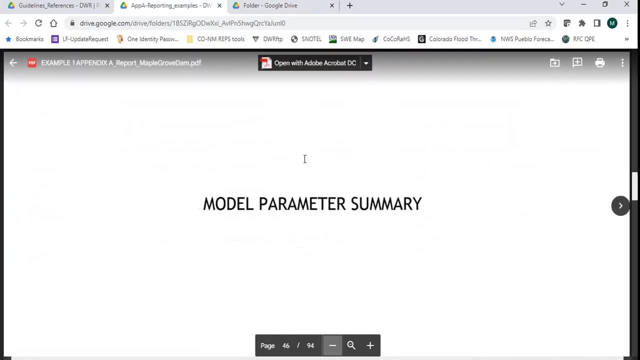 Okay, And then we, and then we'd also like to see the the completed Clark unit hydrograph parameters estimation spreadsheet, if you, if you, use that, Okay. So let me jump here Here to appendix A, and I've already to one of the examples. example A reporting. 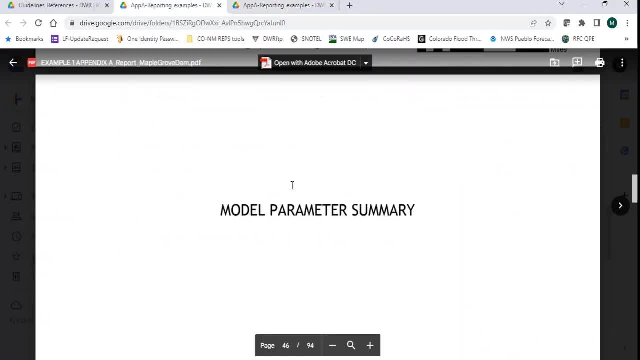 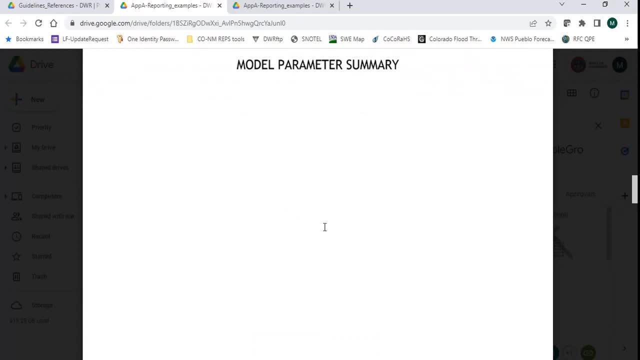 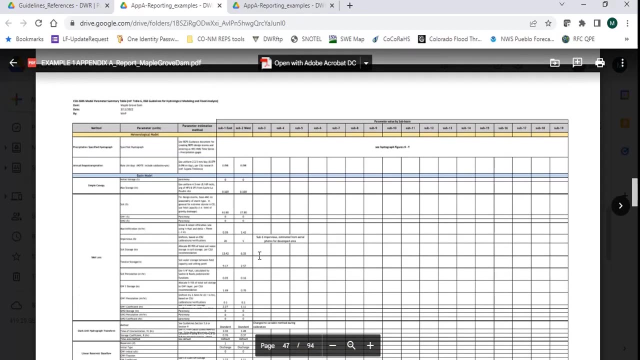 I think this was for Maple Grove Dam and I already have it- have scrolled down to the model parameter summary. So this section six, reporting, and let's just take a look here. So we'd have the. we want to see this table six, your, your table six, filled out for your. 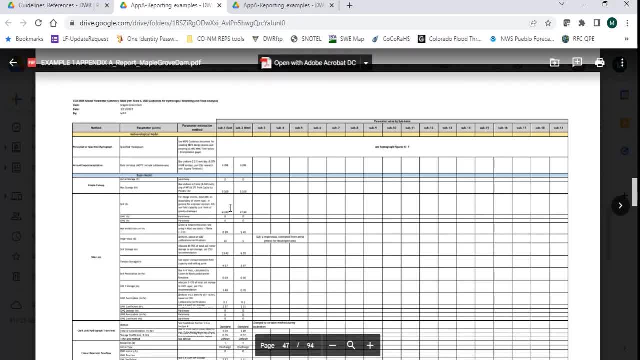 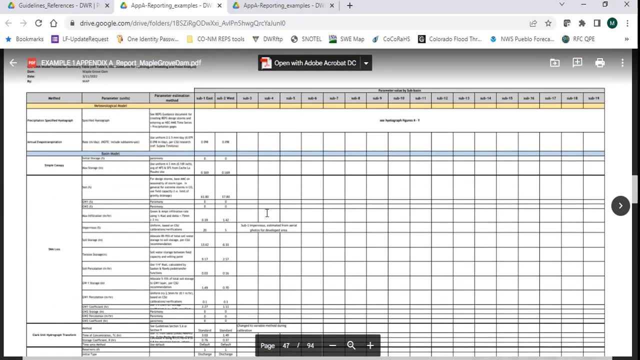 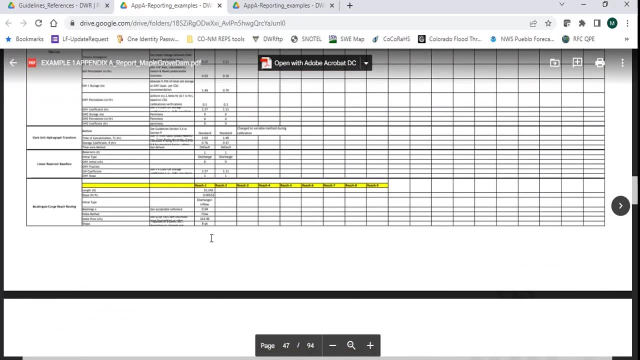 basins. In this case we only had two sub basins. It was fairly easy but we completed all the PR, entered the table, completed the table for all of the HEC-HMS parameters, all the elements, methods and parameters for each of those. 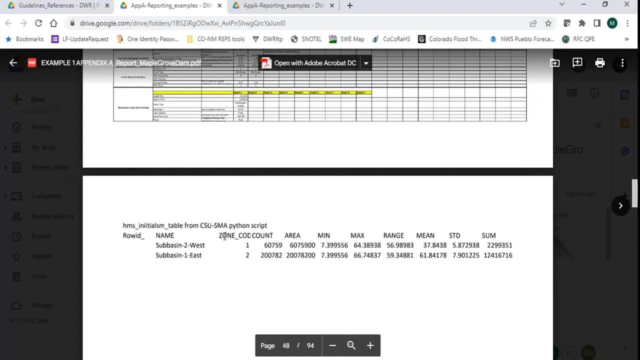 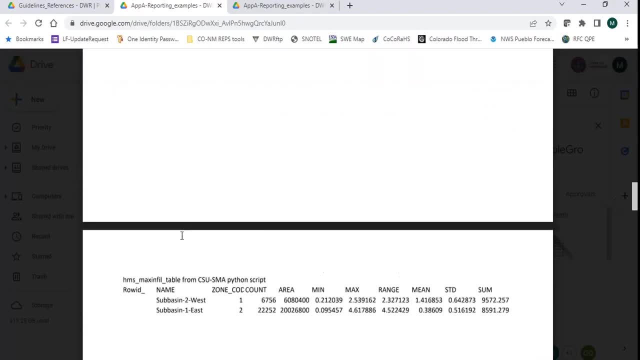 So that's that. And then again the CSU SMA Python script output for the parameter estimates. So for example, here initial SM, And so each of those is just It's going to. you're just going to print out that, either the text file, or open it in Excel and print it. 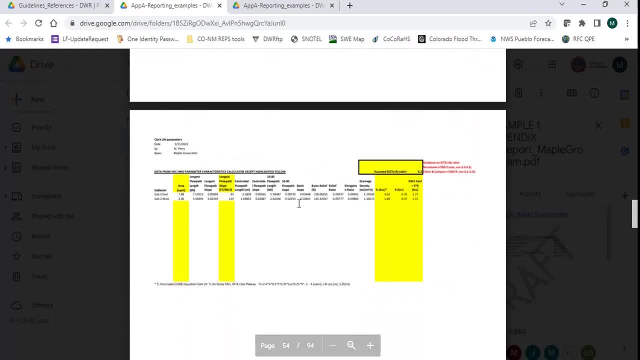 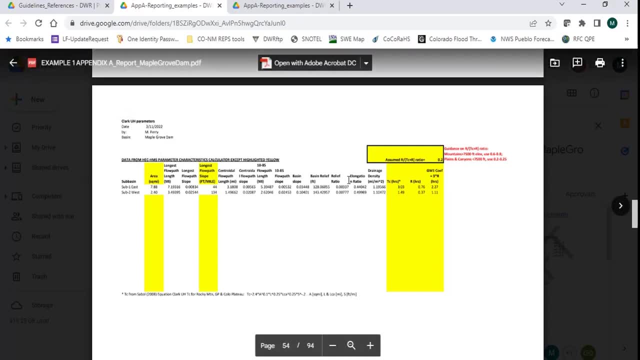 And we just want to see it printed to a PDF and included in the report and then print out of the your Clark unit hydrograph parameter estimation spreadsheet, the example we gave you, or if you have some other method of a spreadsheet tool to use that we just want to see a print out of those Clark unit hydrograph. 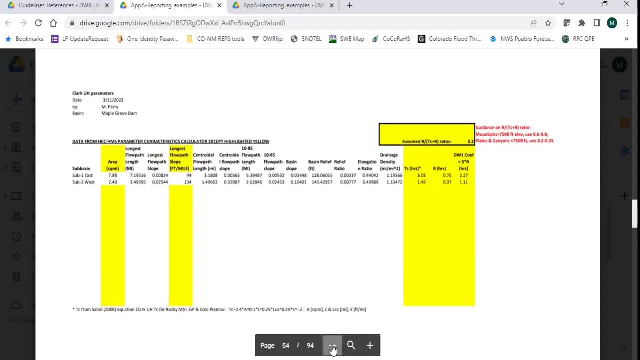 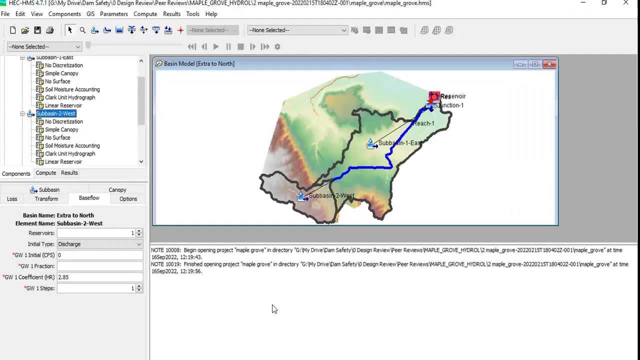 parameter estimates there. And that's actually It for the parameter estimate reporting. pretty simple. Let's jump to HMS real quick. I just want to show you an example model for one. that's been the all the parameters have been edited at input already. 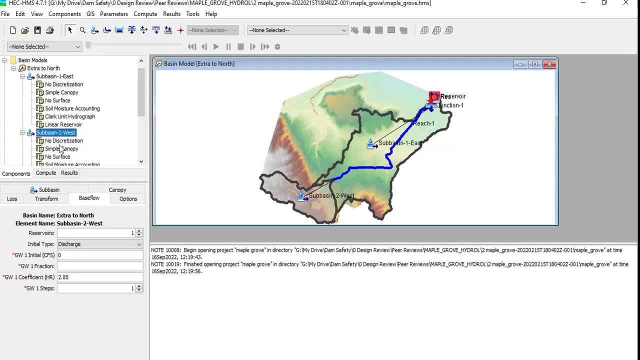 So we'd have our basin model and we have a sub basin here and the sub basin elements- the sub basin elements we have, or the element, the sub basin element. the methods we have, sorry, are simple: Canopy loss, soil moisture accounting, transform Clark unit, hydrograph, linear reservoir, base flow right. 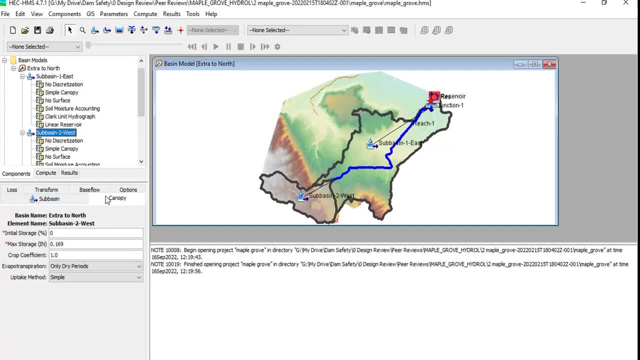 And then we can, we can flip through each of those. So canopy. we had that max storage, initial storage zero. max storage 0.169, crop coefficient 0.10, uptake method: simple. And then the loss. we have all these parameters, our percent soil right. 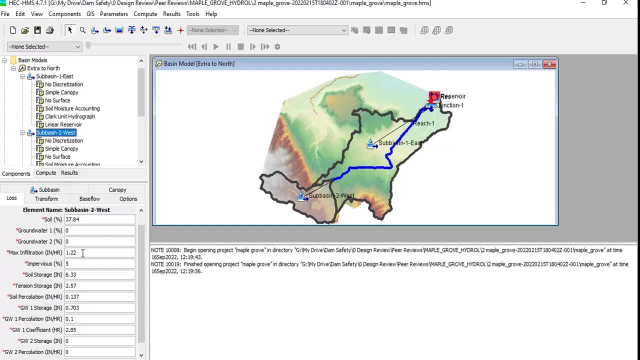 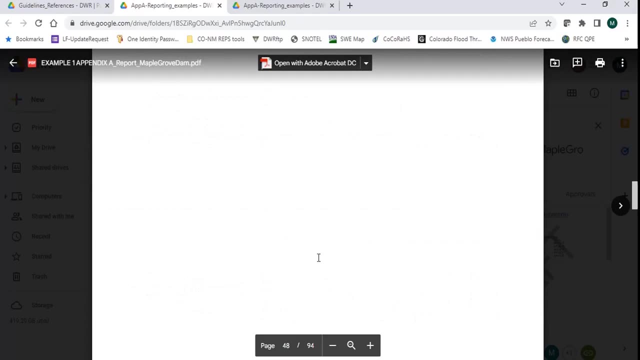 Groundwater: ground groundwater: 1% groundwater: 2. Max infiltration: 1.22. impervious store storage. So cross-reference again back to back to that table six and that all those parameter values were you summarize them all in table six. 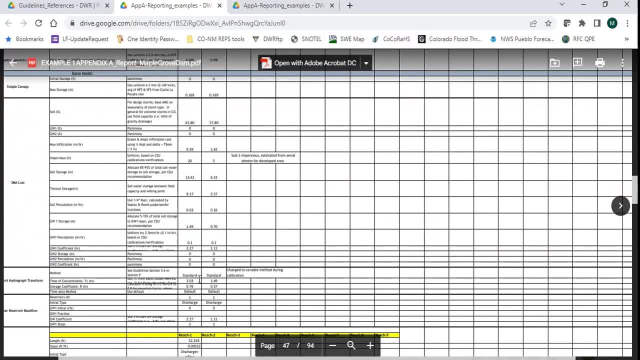 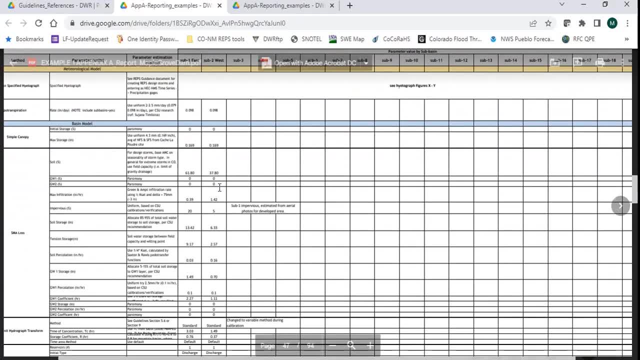 So they're all there for easy reference, Every one of those parameters. Okay, So so a loss, SMA loss method. so percent for sub basin. I was looking at the sub basin two West, So so percent starting in antecedent moisture. 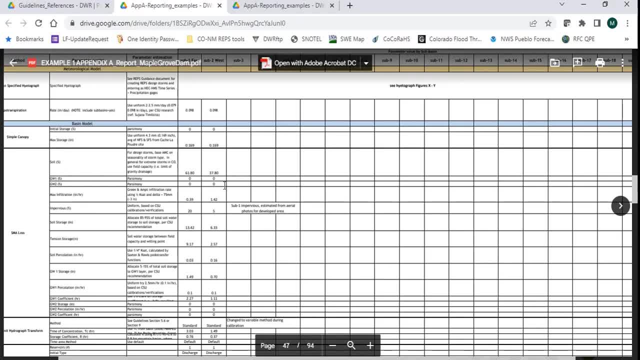 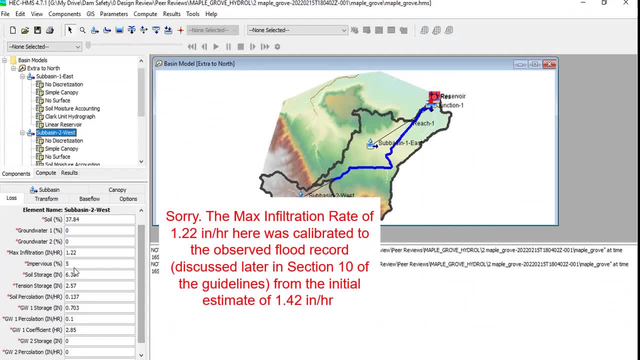 Okay. Condition: 37.8%: groundwater: 1% zero groundwater: 2% zero. maximum infiltration rate: 1.42. impervious five right. So that's where that, that's where that all can. you can get it all. 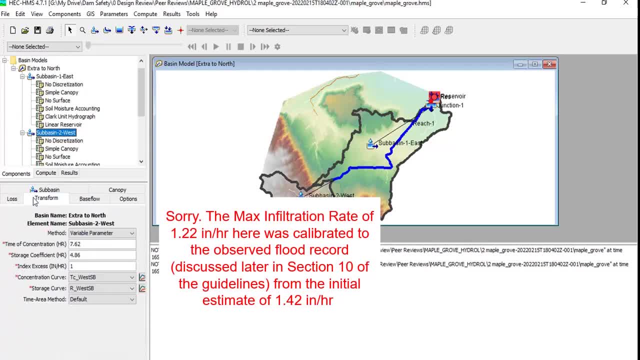 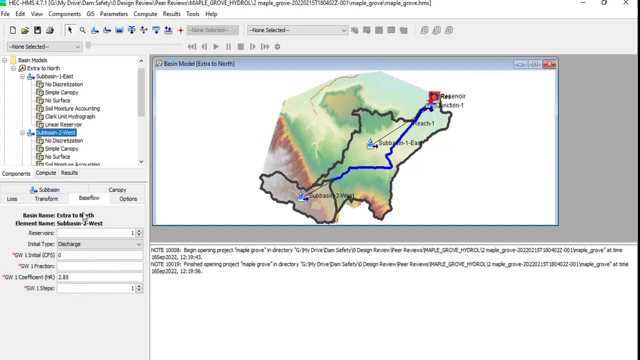 All kind of come kind of comes from transform the Clark unit hydrograph parameters And in here this is a front range base And, like I said, we ended up using the variable method, nonlinear response, in order to match, So the observed, to calibrate the observed flood record. we can talk more about that later. base flow method in our sub basin element and the parameters for that groundwater coefficient is three are right. 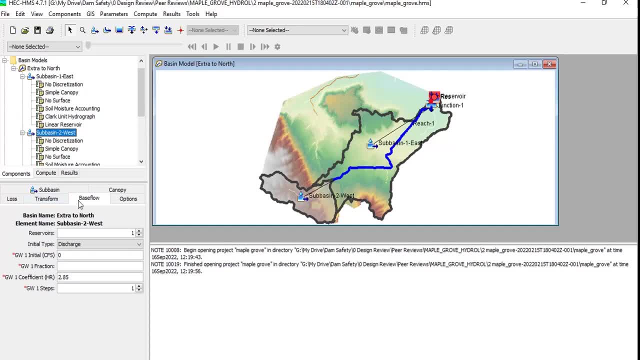 That's three. three times are the Clark unit hydrograph are in that I said that shows up twice. It shows up under base flow and under the loss method. where you have a groundwater, one coefficient- That's the same Three times- are set to get water out through inner flow. 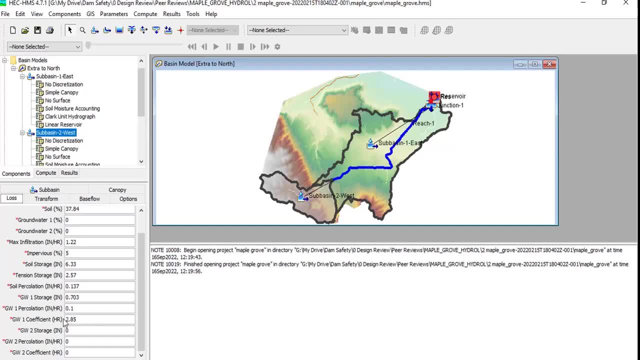 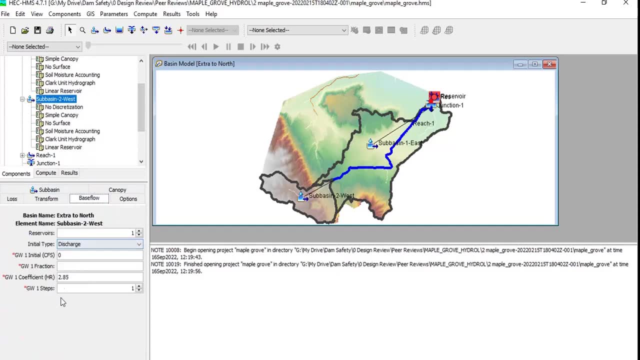 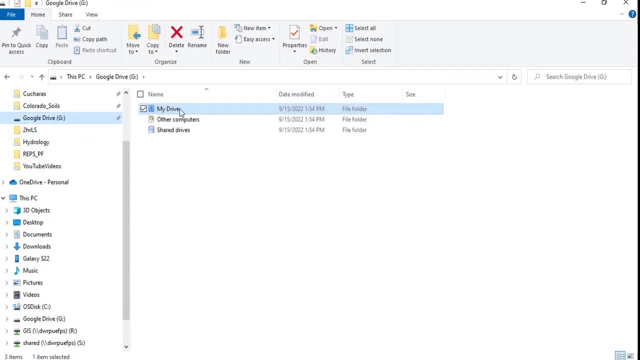 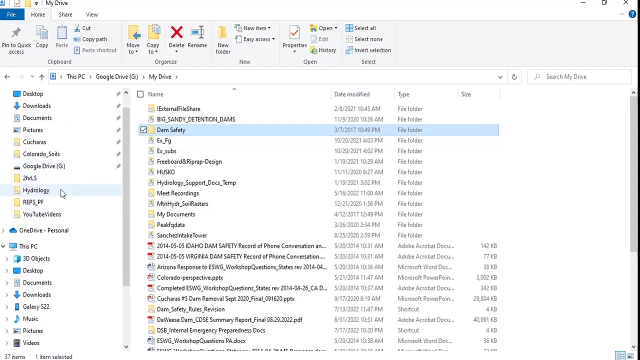 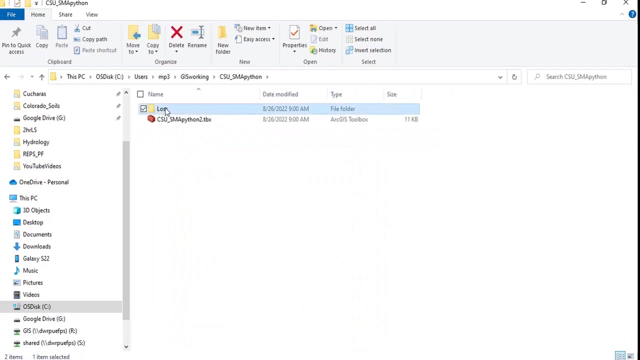 It actually goes through two time coefficients through the groundwater, one coefficient- And then through the base flow coefficient in HMS. want to take a look quickly at the at the CSU SMA Python script. Okay, here we are. This is with a folder right downloaded, the CSU SMA Python script in our toolbox. 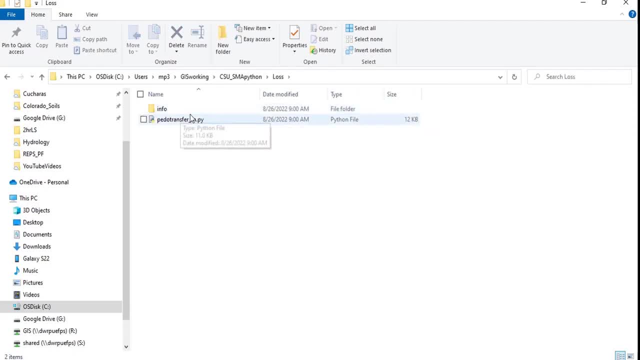 I mentioned that that could be edited. So it is just if you drill into that loss folder that you downloaded it. This is the pipe P. the dot P Y file is the Python script. You can just, if you have idle, you can just edit Python in idle. 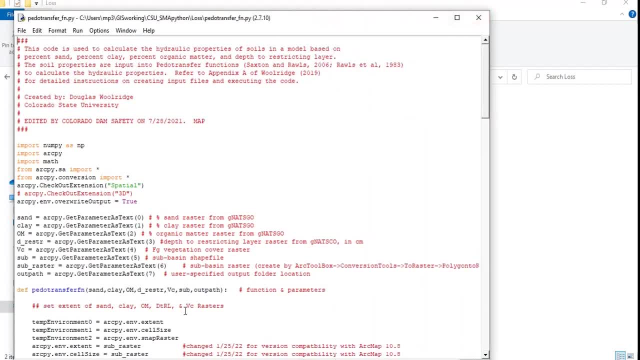 Okay, so here is. here is the code. We also have the code written out in Appendix B, The electronic appendix of the guideline. Okay, So here is the code. We also have the code written out in Appendix B, The electronic appendix of the guideline. 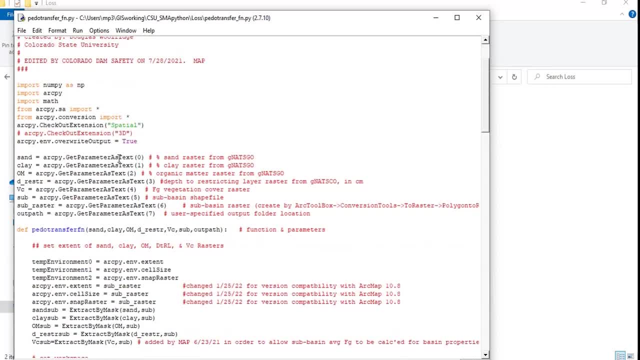 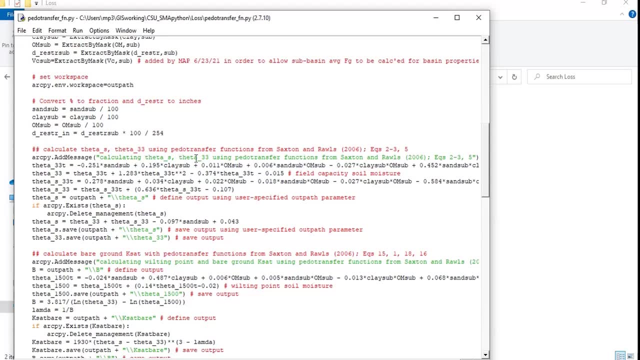 Okay, So here is. here is the code. We also have the code written out in Appendix B, The electronic appendix of the guideline, But you're able to download it and you you can edit it. So this is all editable and we tried to try to put enough notation in here that it's easily under, can be understood and referenced. 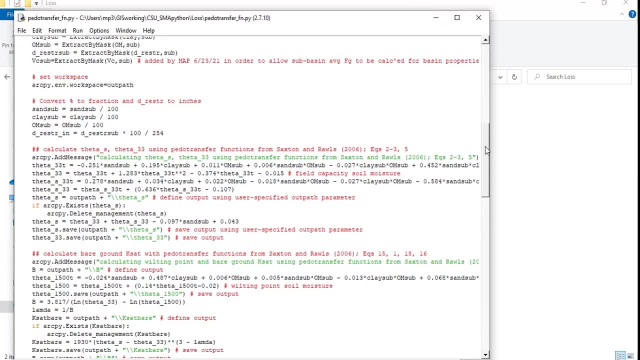 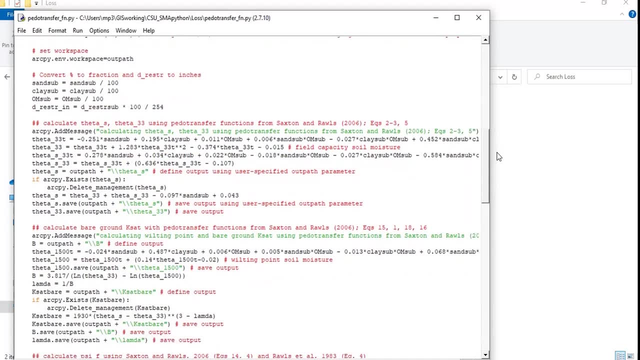 So it I would, you know, just say that it's fully transparent. You can read it, see what it does, And then if there are things you would like to change, for instance we talked about if you would like to change the antecedent moisture condition in that initial 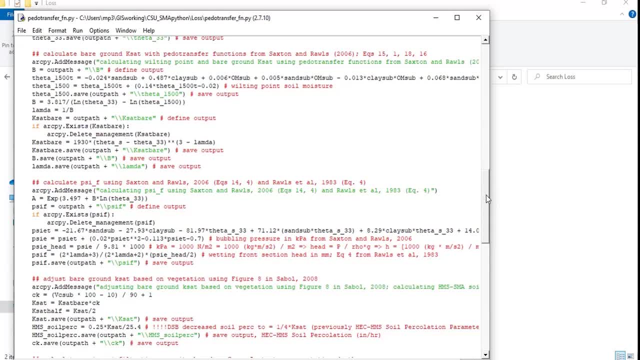 soil percentage. you can change that to something else besides field capacity. We also talked about that. we, that CSU, used the, the percolation rate to the from the soil layer to in HMS to the groundwater, one shallow groundwater layer of one half KSAT. 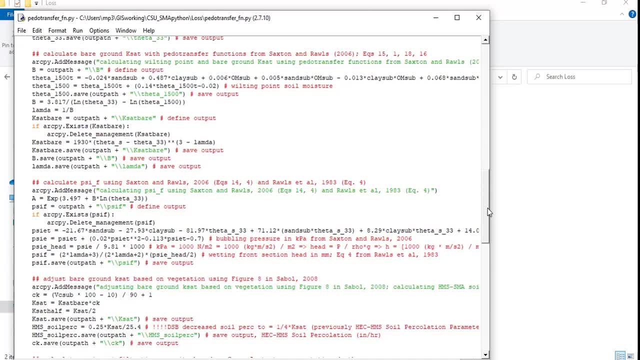 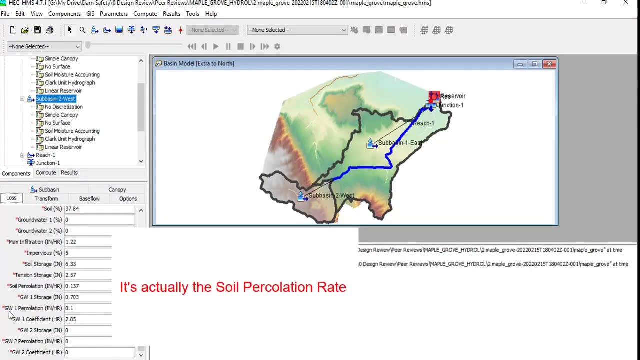 and we DM safety has found that we like kind of kind of calibrated to more of a one to one quarter KSAT so that the script, the way it's written, now uses one quarter KSAT for that, for that groundwater, Groundwater, one percolation rate. 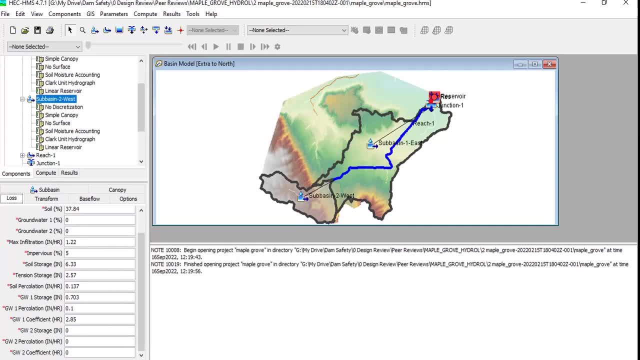 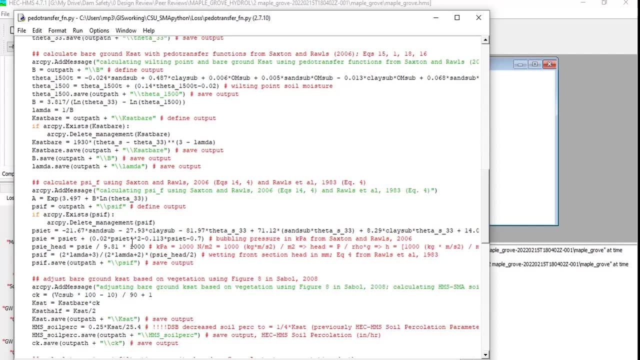 You can change that if you want to. the the general statement here is that we, when Colorado Dam Safety is reviewing the project, We will use our version of the python script and any so any changes you need, you as a user engineer will need to. should document any changes you make to the script and justify those in your reporting. 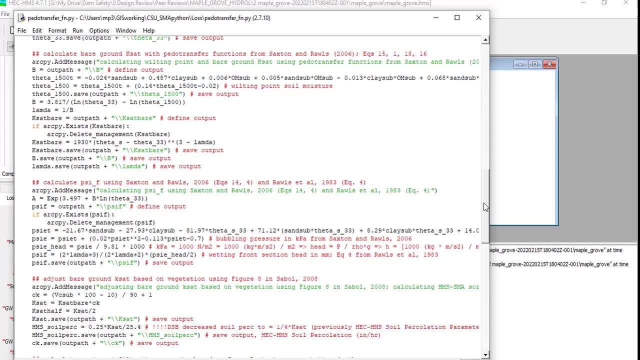 Explain why you made, what changes you made to the CSU SMA script, If you did that to estimate parameters, and why you did that and other than that. it's there to be, you know, to be edited as as you want. It's fully transparent. 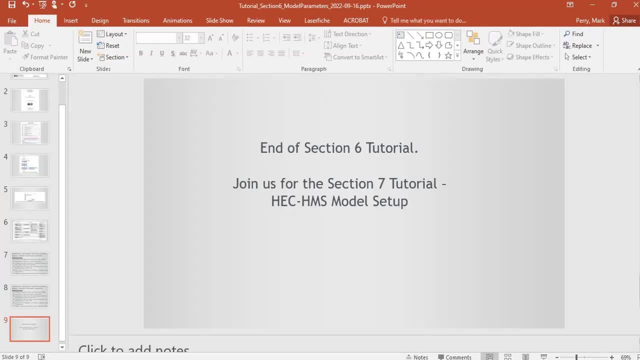 Okay, Okay. So that wraps up the our section Six, tutorial section Six of our new guidelines for hydrological modeling and flood analysis, And it was on the section Six was the model HMS, CSU SMA method, heck HMS model parameter estimation. 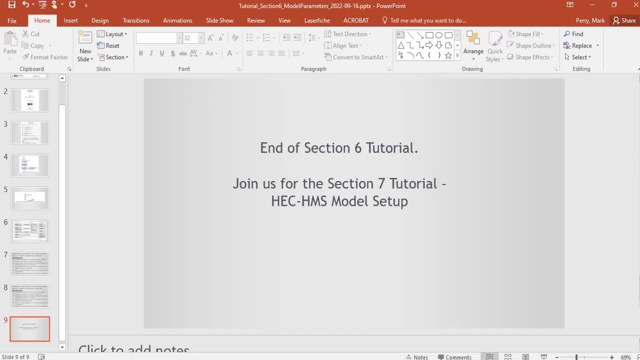 And just a quick recap. We- I showed- went back and showed the Properties output from section five just to show where we had. we got here and we were using those properties now in section six to estimate parameters. We went through the, through the guidelines and here in section six and did a pretty thorough discussion of how we, how we, what, the, what the, how the bottles set up. 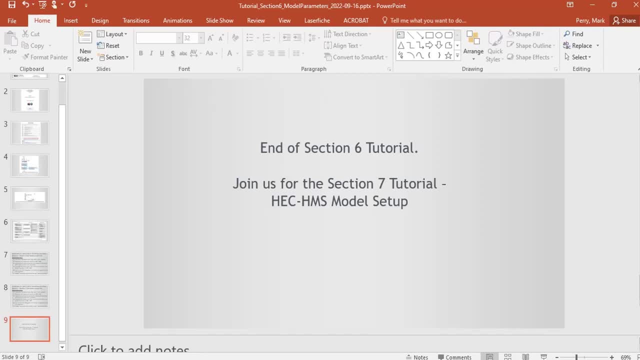 What all the parameter parameters are, parameters are, and how the parameter estimation methods were developed and what they are. so hopefully everybody feels comfortable with those and, like I said, at least where they came from. so you can we provide all the references- the urban master's thesis, the Saxon Rawls papers that you 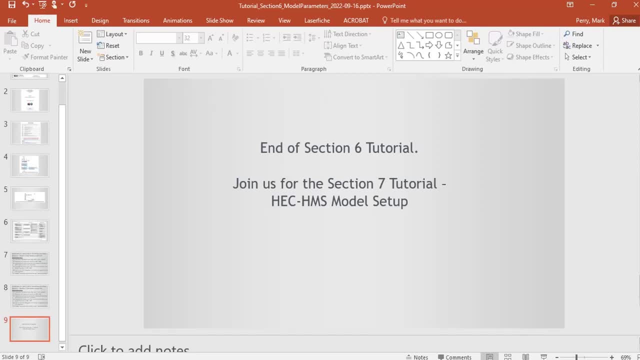 can go back in and see those for yourself. they're all provided on our dam safety Google Drive. it's linked in the guidelines document. then we went through the, the, the CSU parameter estimation, CSU estimate. Python our toolbox- how to download that. have loaded in our map estimate, run it and get the. 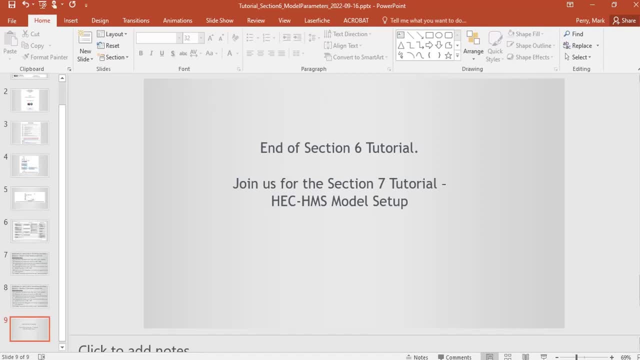 parameter estimation tables for heck, HMS export those we went through the our Clark unit hydrograph spreadsheet and to estimate Clark unit hydrograph. that you can use to estimate Clark unit hydrograph parameters. pretty simple. and then table six, which is the summary kind of our master summary table of all.